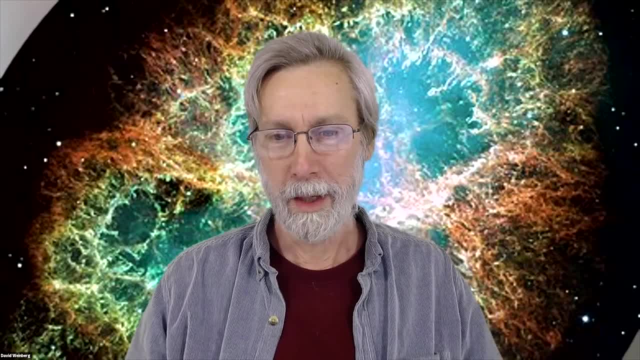 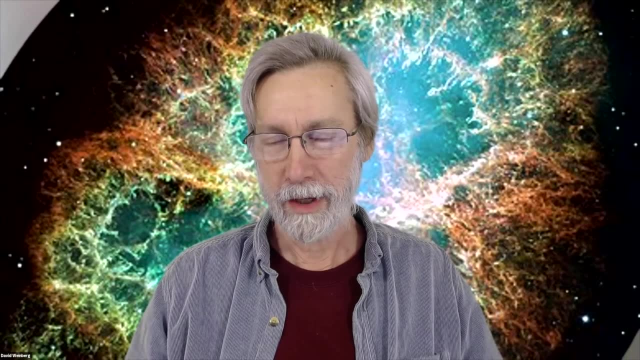 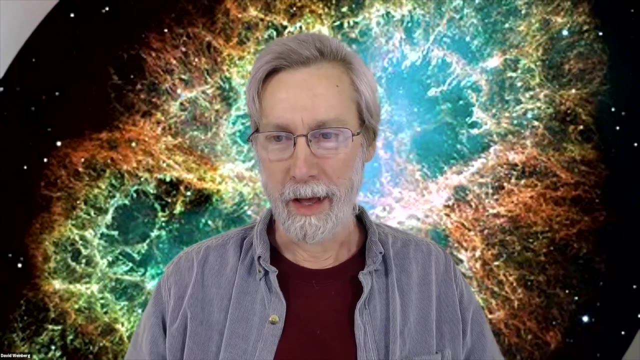 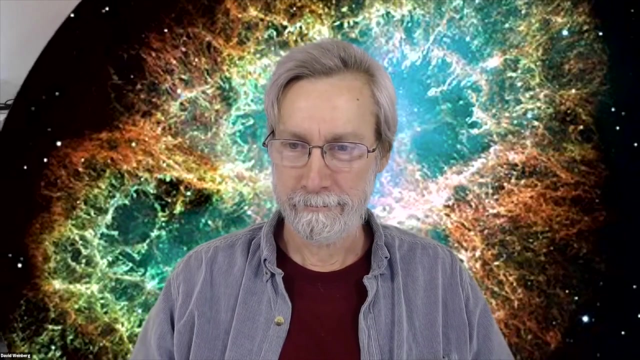 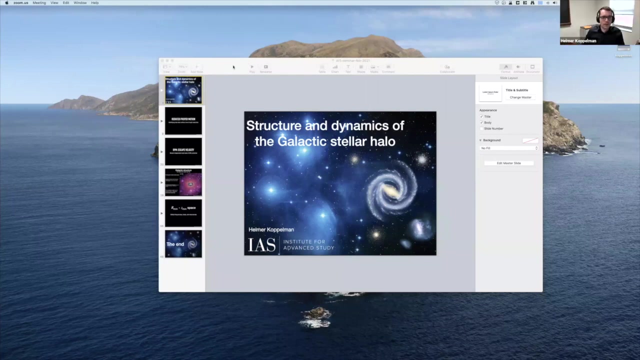 Amina Helmy and their collaborators have done a tremendous amount to combine Gaia and other galactic surveys to really identify novel features of the history of the Milky Way, And he will tell us about that today. So take it away, All right. thank you for the introduction, So I'm not going to talk about the merger. 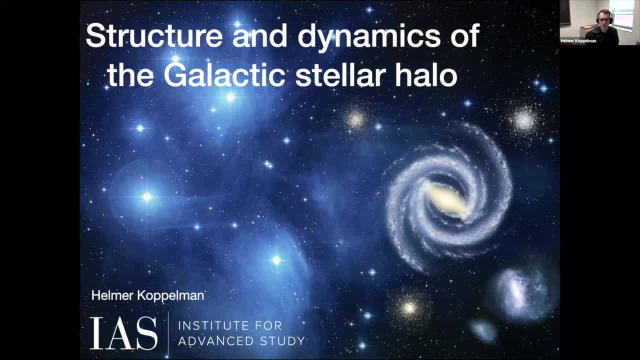 history of the Milky Way today, but most I'm going to talk about the how, the mergers of the, or how the merger history of the Milky Way affects the structure of the Milky Way and with emphasis on the structure of the stellar halo of our galaxy. 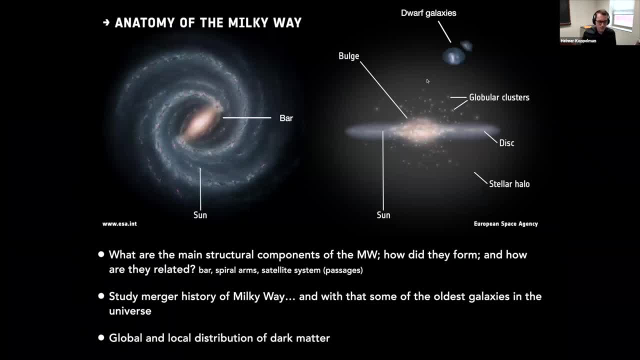 And so the main drivers for my research and the main questions that I'm interested in answering are: what are the main structural components of the Milky Way, how they form, when did they form and how are the different structural components related? And, especially, what is the influences of dwarf galaxies interacting with the Milky Way? 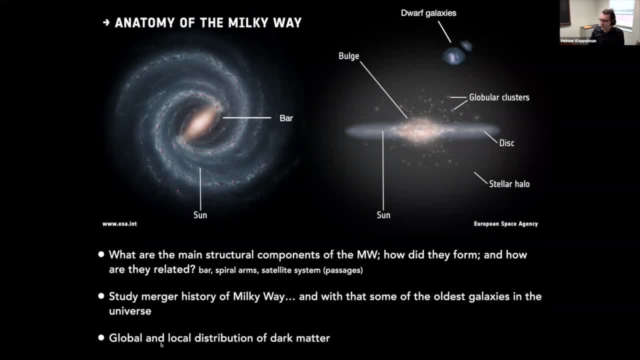 And so the other question that is interesting or relevant for today, which I'm interested in answering, is: what is the global, and especially the local distribution of dark matter in the Milky Way, And especially in the halo, because we know that the halo is mainly dark? 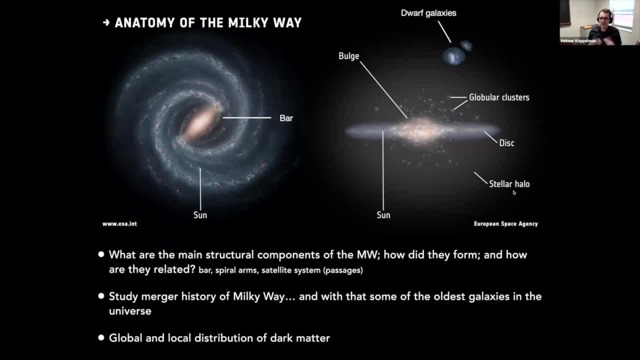 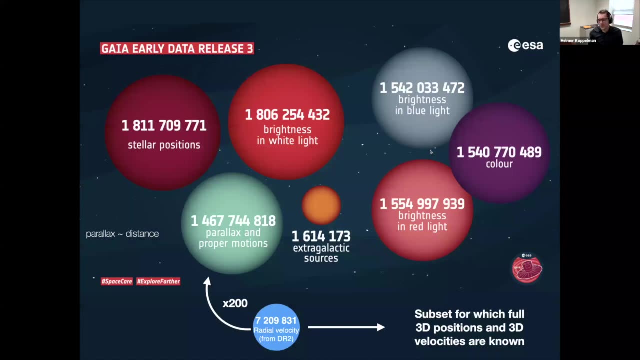 And we have a. we think we have a quite good understanding of how much dark master is in the Milky Way, but we don't know at all what the small scale structures of the dark matter in the in the halo, And so the currently the best way or one of the most popular ways of studying the Milky Way is using data from Gaia. 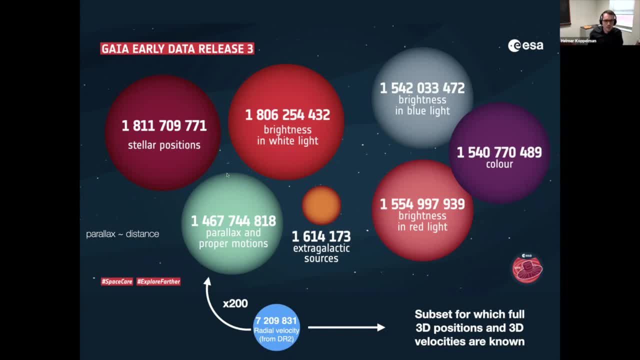 I think I've shown this before So I'll just talk about it briefly. So the most relevant for today's Green bubble here, which is the one and a half billion stars for which Gaia is measured Not only stellar positions and color and brightness information, so photometry, but it does also measure parallaxes, which is a measurement of the distance up to the star and also proper motions. 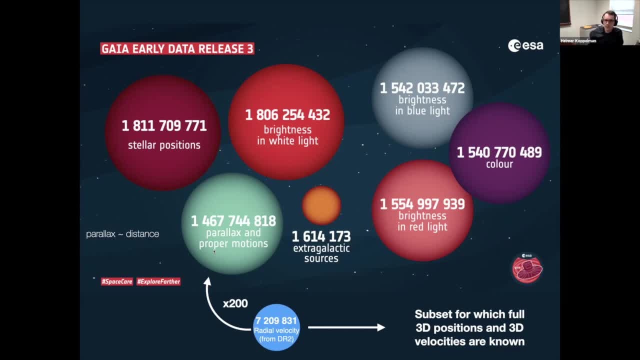 So proper motions are the motion of the star on the sky. So it's just two components of the three, the velocities. So you'll notice That for most stars- so only one in 200 stars in the Gaia data set, We have the additional radial velocity, or the line of sight velocity. 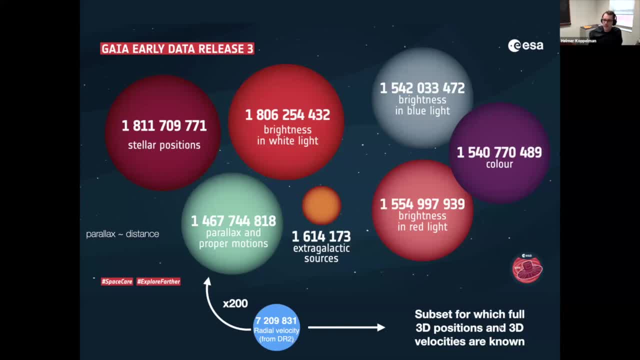 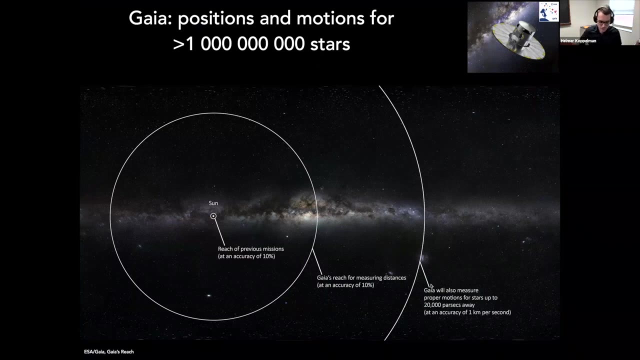 And so actually for most stars observed by Gaia, we have 3D positions but only 2D velocities. So we have missing information on the velocity And I think I've also shown this before. but I really like to emphasize kind of the 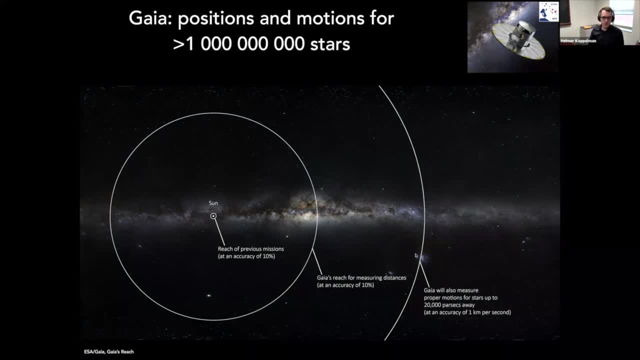 How large the volume is that Gaia has observed currently or by the end of the mission, the expected volume, And so we're looking here at the an image of the Milky Way. This is the galactic center here, And this is the sun about eight kiloparsecs away from the galactic center. 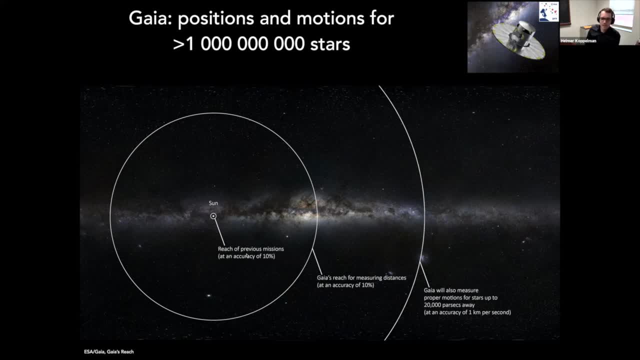 And the small volume around the sun is the reach of previous missions. So before Gaia, the reach with accurate distances. So it's if you compare the larger volume for which Gaia is Measured accurate distances, Then previous missions were only really probing the backyard of our sun. 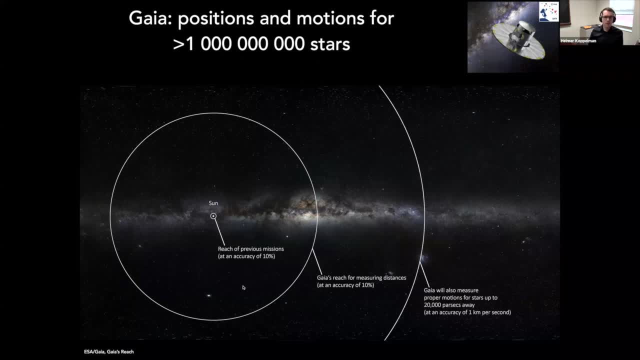 And not at all the large scale structure of the Milky Way. But also, you do also see that, even though you know the improvement of Gaia, the Gaia data is significant with respect to the previous data, Still this volume is not, it doesn't capture the entire Milky Way. 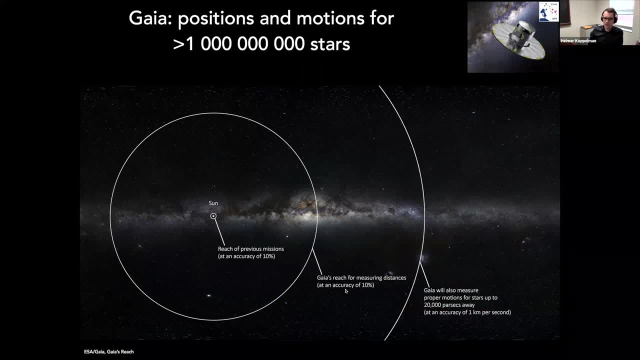 But especially if you stick to a high, accurate, high, accurate, high position data, You will find there are still relatively local sample of stars And the larger volume here is the volume for which Gaia will measure accurate, proper motions, Which it is able to do for stars which are further away. 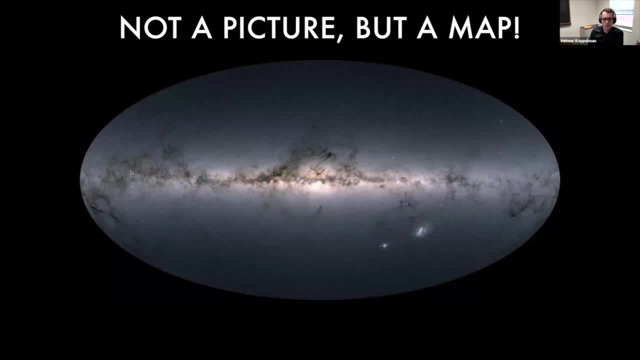 And so to emphasize this a little bit more, So if you see an image like this, it's not actually an image or a picture. Well, it's a map. And so for all of the stars here, So for each dot- and you can't even see the dots here- 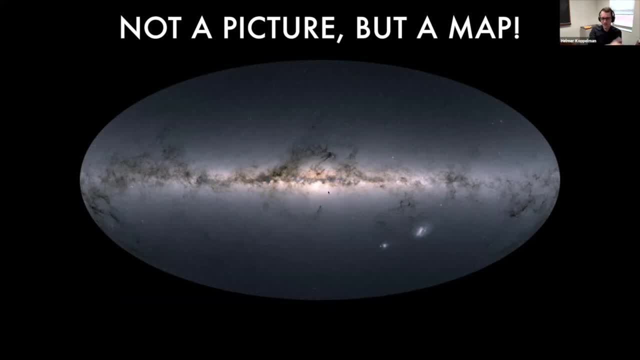 We've measured brightness, color information, or Gaia has measured. I keep saying we, but Gaia has measured Photometry, positions on the sky, distances and proper motions, And so I'm afraid this will not play well over Zoom. 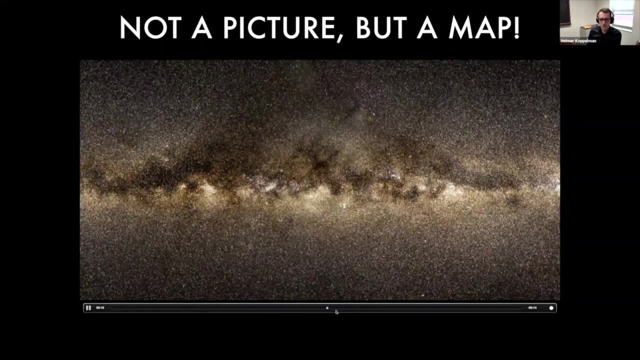 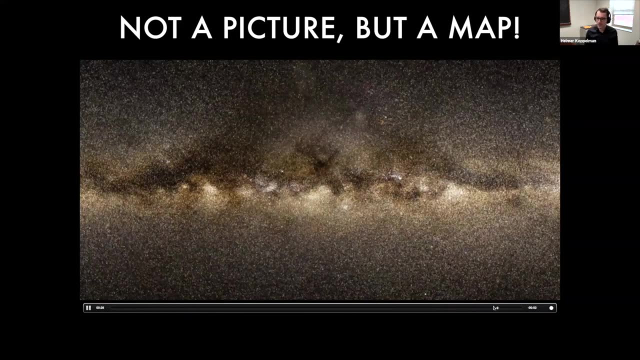 So I'm going to fast forward it, But you know, for all of these stars, we know how they move, And so we can fast forward this in time. We can see how the entire Milky Way is moving around, And I think this is something that's easily skipped over and forgotten. 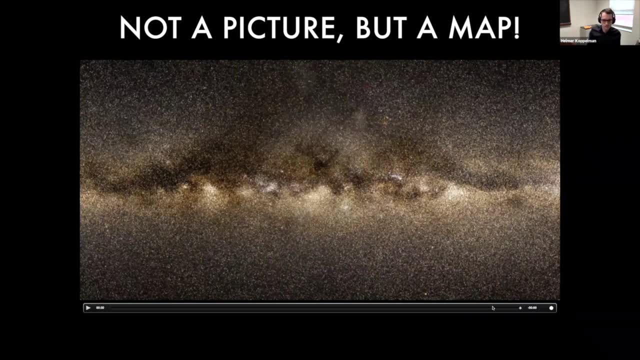 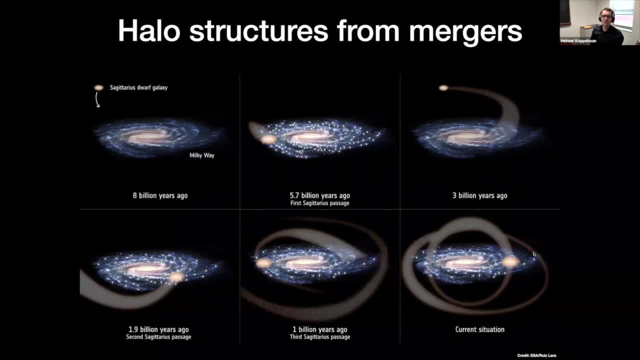 I just wanted to emphasize this. This is the kind of data that I analyze, And so when I'm talking about structures in the halo, it's a very general term. So what kind of things am I talking about? And I'll keep talking about it in general terms, because there are many different ways to interpret structure in the halo. 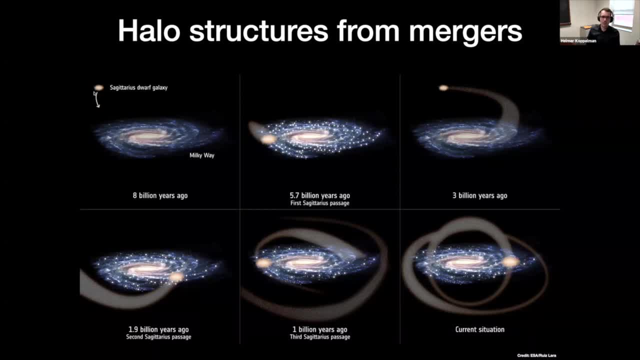 But one example is the typical picture. One example is that if a dwarf galaxy emerges with the Milky Way, is that its stars get stripped from the dwarf, from the core, And so in the end you end up with the stars from this dwarf galaxy populated in these streams that are orbiting in the halo of the Milky Way. 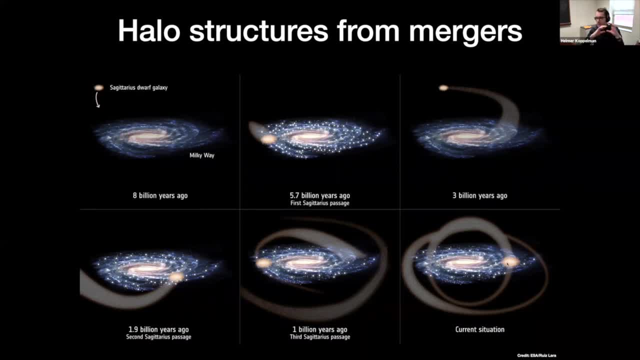 So for the specific Sagittarius dwarf galaxy, there is still a core intact in place, But for dwarf galaxies that emerged a longer time ago, the entire dwarf galaxy will be disrupted, And what you're left with is just this stream, these streams of stars. 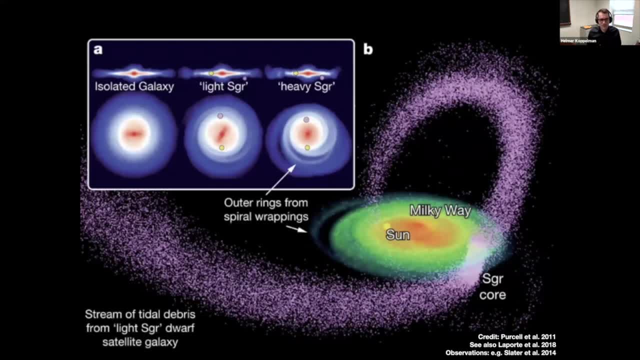 And so to give some kind of understanding of what kind of interactions can take place in the Milky Way, is that you know, if you model the specific merger of the Sagittarius dwarf galaxy with the Milky Way, is that not only the dwarf galaxy is disrupted? 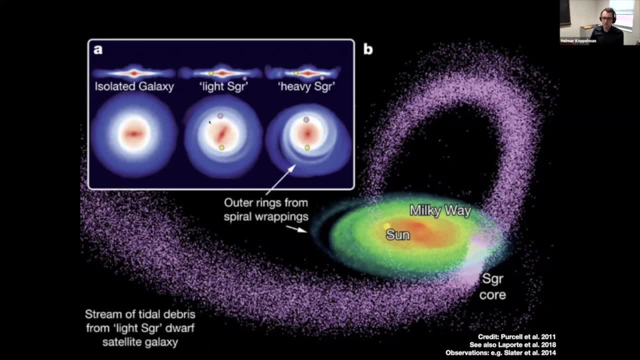 but also part of the Milky Way Is affected and perturbed, And so we see this here. So this is a relatively old simulation, But this is also very recent and current work. So ongoing work is to understand the interaction between Sagittarius and the Milky Way. 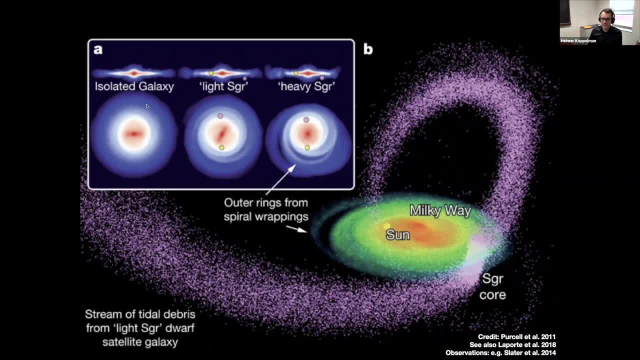 And so one way to look- for you know the structure that is induced by this merger- is to look in the outer region of the disk of the Milky Way, Or in the left. here we see an isolated galaxy And then the two other panels. 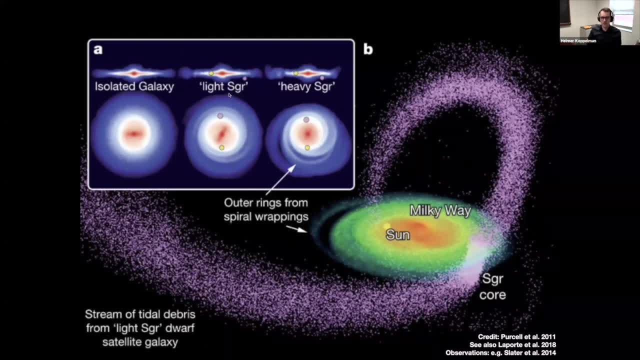 Show a light version of Sagittarius or a heavy version, So with a lot of mass. And so we see that, especially in the outer regions of the Milky Way, there are a lot of perturbations and there's a lot of structure being created by this merger. 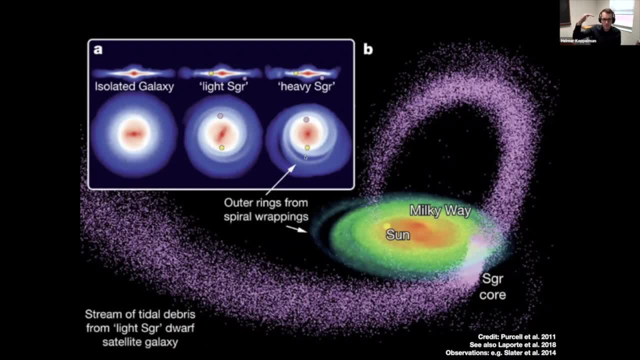 And so this is just one example of the different, you know dynamical processes that can take place in the Milky Way, And I just wanted to emphasize that. you know there's a lot of interactions happening between different components, between different events happening. 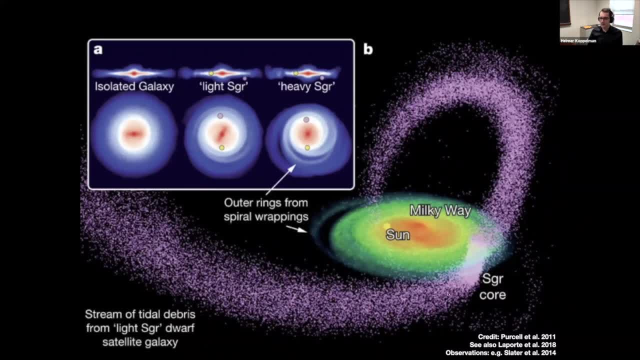 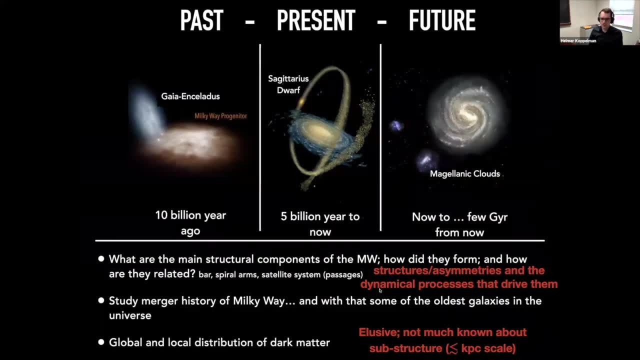 And obviously Sagittarius is not the only merger we've had in the Milky Way. There are many other mergers, And so the question really is: you know, what is causing all of the structure that we see in the Milky Way? 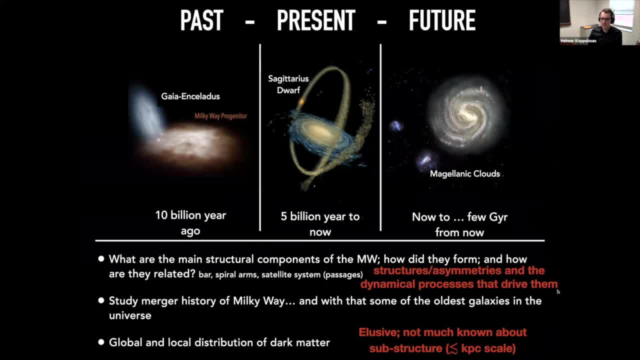 And what are the dynamical processes that drive them. And just to emphasize, so, these are kind of our current understanding of the most important mergers that have taken place in the Milky Way, Which is, as David was saying in the beginning, Gaia Enceladus. 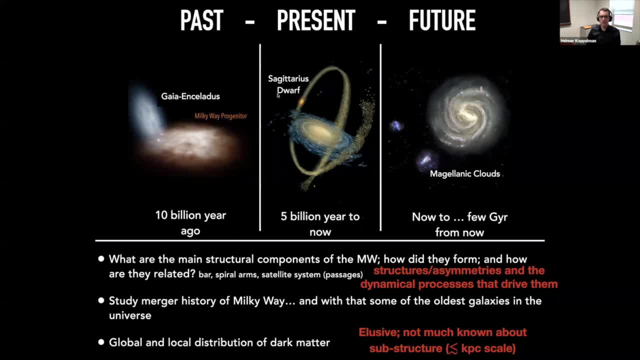 Which merged a long time ago, Then the Sagittarius dwarf, Which is started merging a long time ago but still is merging with the Milky Way, And then there's also the Magellanic clouds which are, as we think, on, the first infall with the Milky Way. 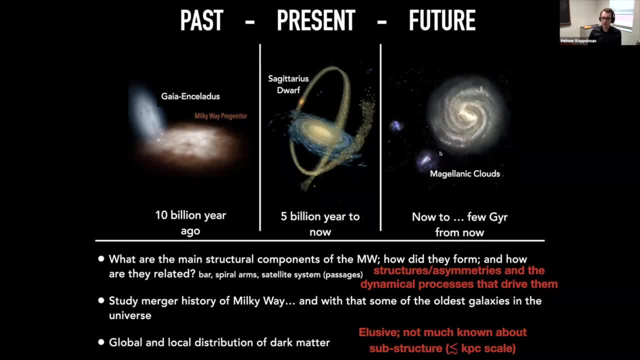 And are already perturbing the Milky Way. They're pulling on the Milky Way And so the question really, so it's really a complicated question. to try to disentangle, you know, the different effects And also internal processes. For example, the power of the Milky Way will also induce structure in the Milky Way. 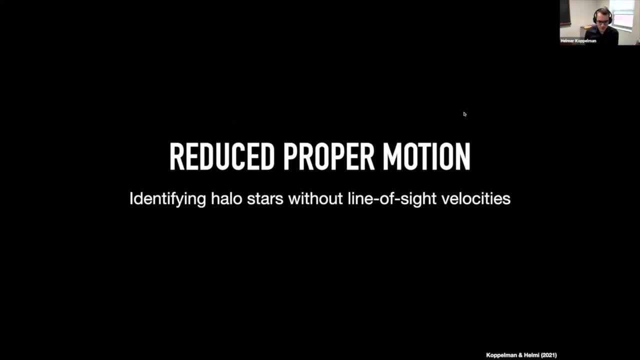 Right. So I'm going to cover- or try to cover, if I have enough time- four recent papers of mine. So the first will be on a reduced proper motion selection, Which is, simply said, just a way to identify halo stars without needing or without requiring the need for line-of-sight velocity information. 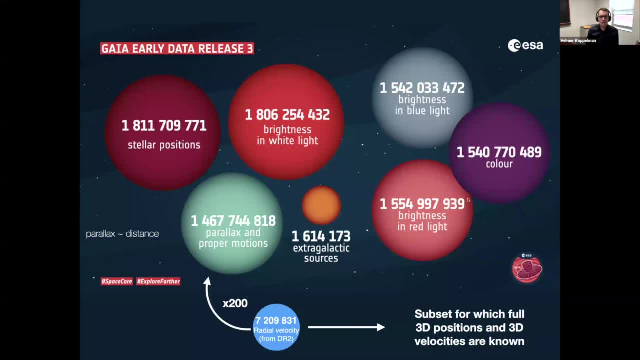 And so, as I was saying before, most stars in Gaia don't have this line-of-sight velocity information, And so if you have a way or a method to look for or to identify halo stars, that doesn't require this additional velocity component. 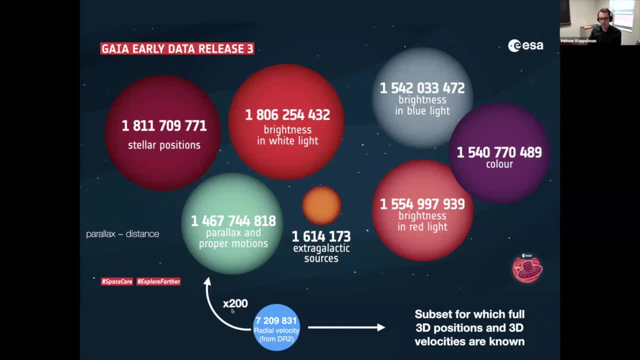 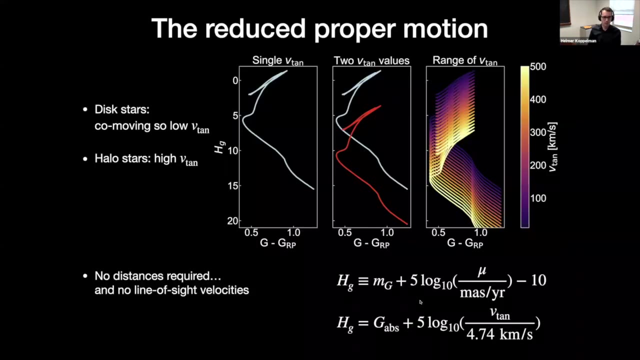 Then there's a potential increase in about a factor of 200 stars. So potentially you have a lot larger sample of halo stars Then you would be able to obtain from this small bubble here. But the downside is that you're missing this one velocity component. 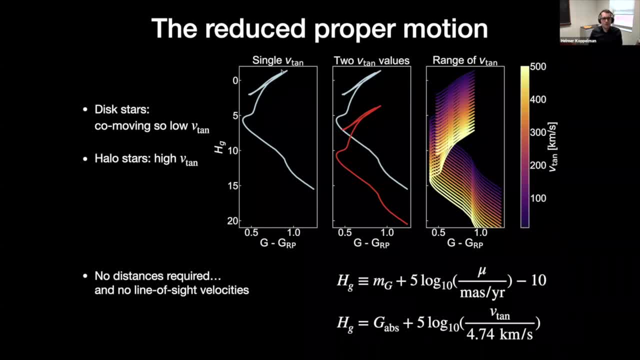 And so one way to omit or to select halo stars without this velocity component is using a reduced proper motion, Which is just this equation here. So Hg is the reduced proper motion, Which is a combination of the apparent magnitude of the star Plus a term that is the logarithm of the proper motion. 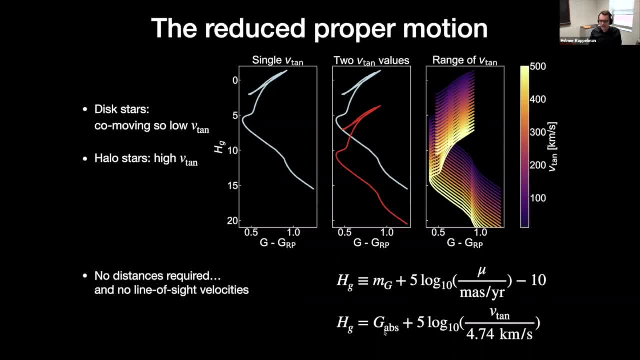 And so an easier way or a more intuitive way of looking at the reduced proper motion is by rewriting it Into a term of the absolute magnitude and the logarithm of the tangential velocity. And so, if you plot the reduced proper motion as a function of color, 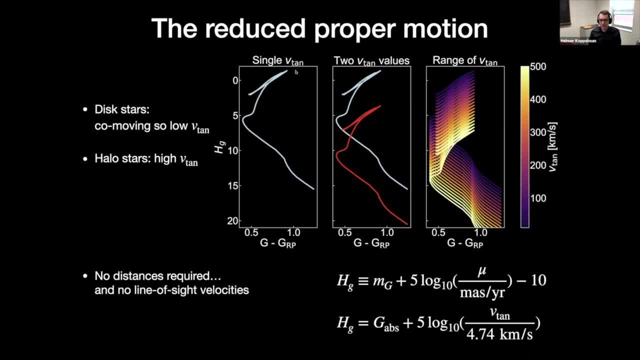 Essentially what you get for a single stellar population Which has a single tangential velocity. What you get is just the color magnitude diagram. So this is just a single isochron, And that's because the reduced proper motion is the absolute magnitude plus this offset. 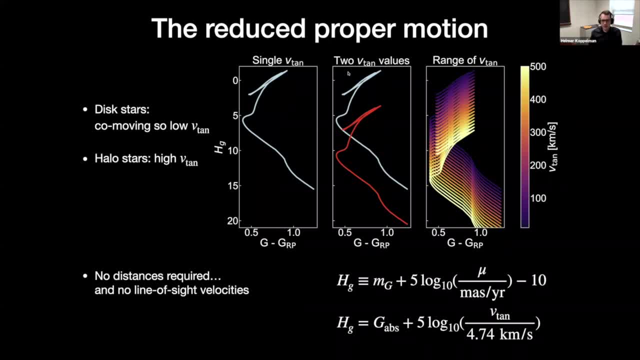 And then? so if this stellar population has multiple tangential velocities, What will happen is that in this diagram, the stellar population will split into parallel sequences, And especially the main sequence Is split into parallel lines, Especially for the actual population of stars in the Milky Way. 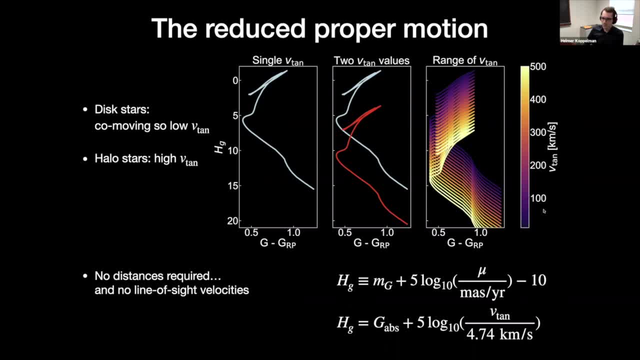 Which have a range of tangential velocities Ranging from close to zero to large- I don't know- 500, maybe larger kilometers per second, And so what this will look like in the data Is a set of isochrons which are split and offset. 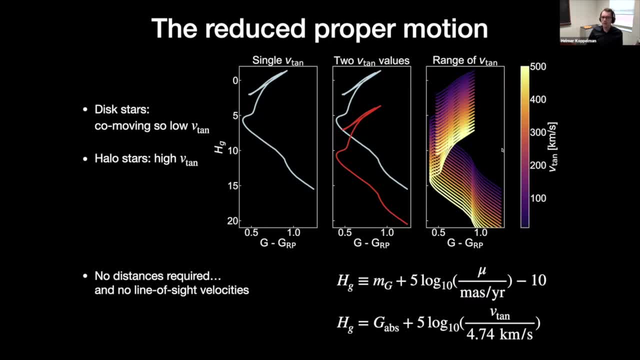 By the tangential velocity of the star, And the reason why this is interesting Is if you look at halo stars, Then they typically have large tangential velocities. That's because disk stars are co-moving with the sun And so, relatively, the observed velocity of the disk stars is low. 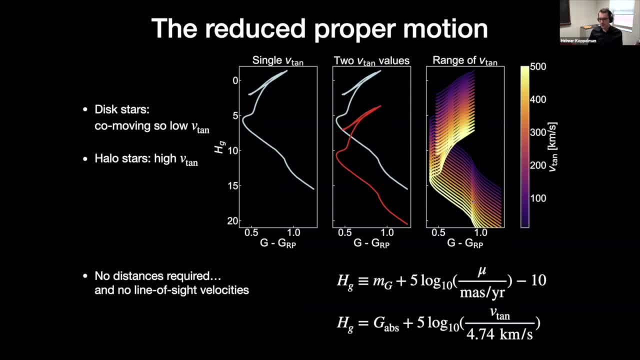 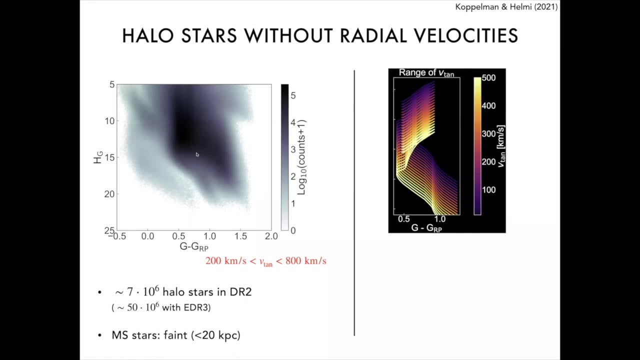 So what you want is really select in this diagram stars that are in this yellow region here, Which are stars with large tangential velocities, Which are then likely halo stars. Can I ask a question? Sure, yeah. Why are you combining these? 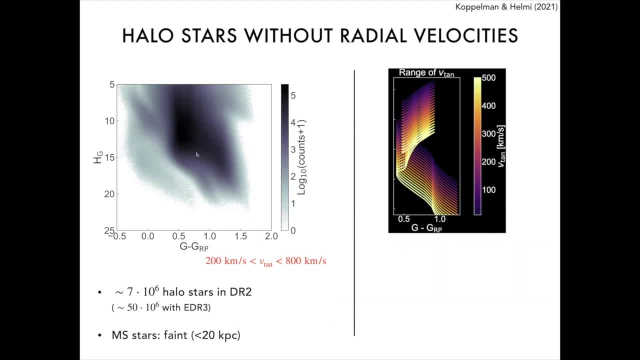 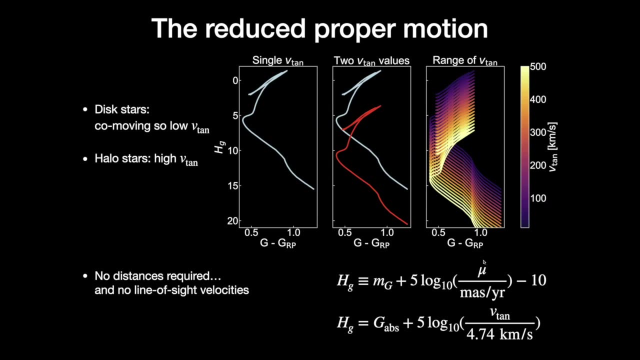 You measure these two things separately And you're combining them into one quantity And selecting on the basis of that. Why don't you select in this 2D plane Using a paramagnet in proper motion? you mean? Yes, It's just for the reason that if the combination of the two 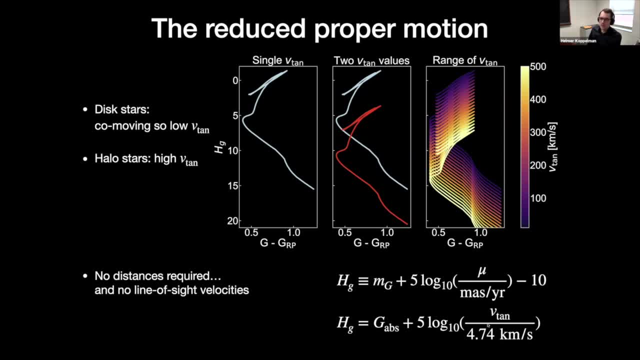 Can be rewritten in this here, And so you can select based on tangential velocity, Which requires the distance. But just by using this equation here We don't need the distance information. There's also a third dimension here, Which is color right. 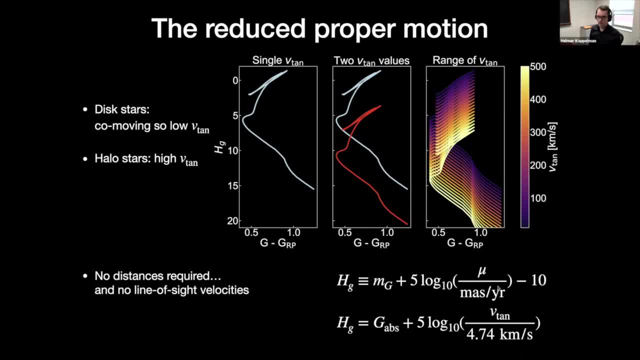 Also. yeah, So you would need to at least make it a selection in a 3D space If you were going to use them, though, But so it's just a matter of it's easier Or it could. yeah, Yeah. 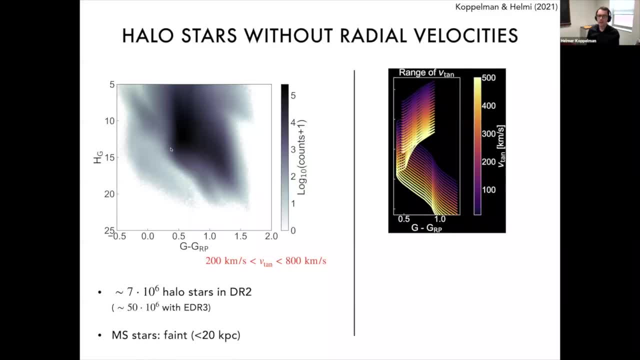 It's just a matter that it's easier, Yeah, And so here on the left we're looking at data from Gaia, And so this is the same, with this proper motion, And this little, this small tail here, This population, here are the halo stars. 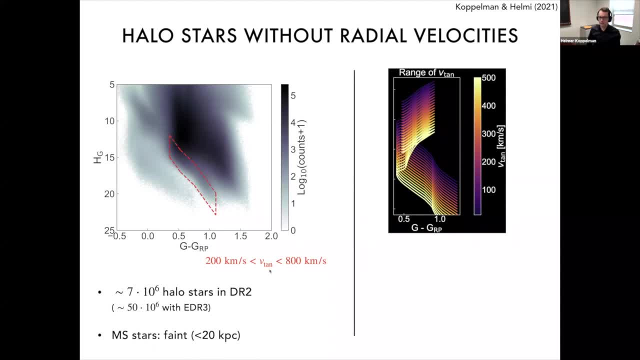 And so we select them, actually by drawing a box Based on where we expect to find stars With tangential velocities Between 200 and 800 kilometers per second, Which which gives these upper limit and lower limit. And so in this, in this box here, 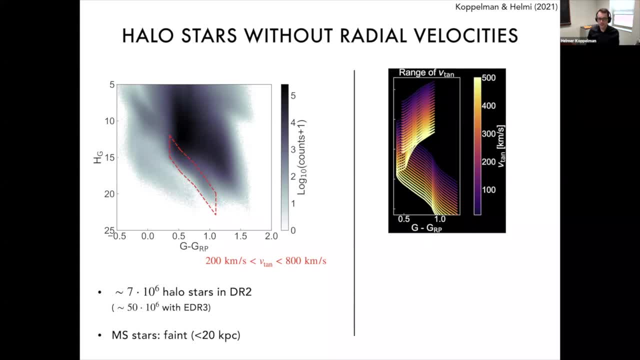 There are About 7 million halo stars, And so this is using old data and with the newest data I checked, So this data released in December, There are actually 50 million halo stars, And so, if you compare it as to what you know, 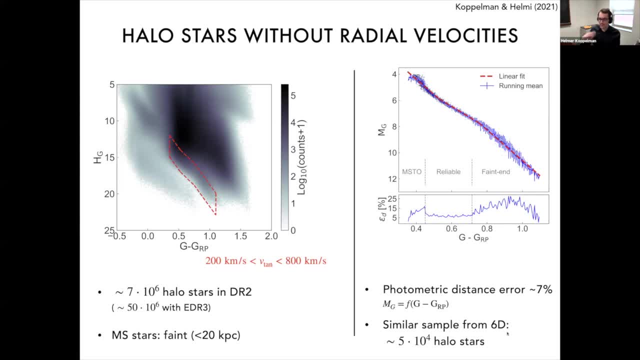 the number of halo stars that are available. If you need this additional line of sight velocity, Then this is just 50,000.. So there's a Significant increase in the number of halo stars And a side note To these stars are selected to be main sequence stars. 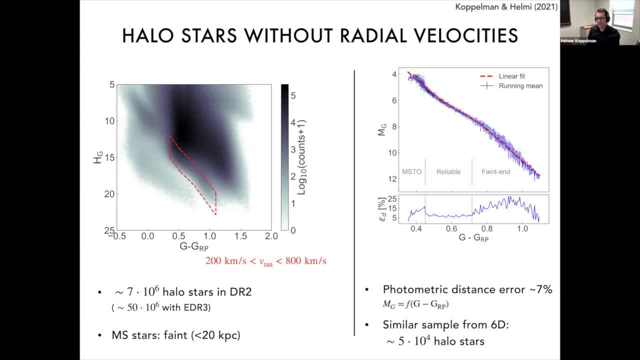 And just because the main sequence, especially in this, the color range, here that's indicated. But it's two dashed lines Because the main sequence is relatively linear. We can use the, the color, absolute magnitude relation Or a main sequence Stars. 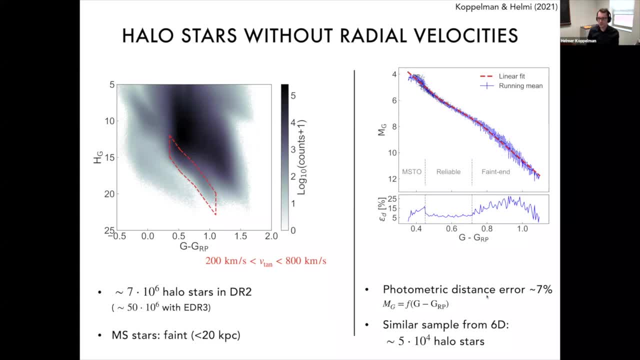 To calculate photometric distances. So the Typically the distance as measured by Gaia As a relatively large uncertainty, So 20%, is already relatively accurate. So the photometric distances with uncertainties of 7% is Much more Accurate. 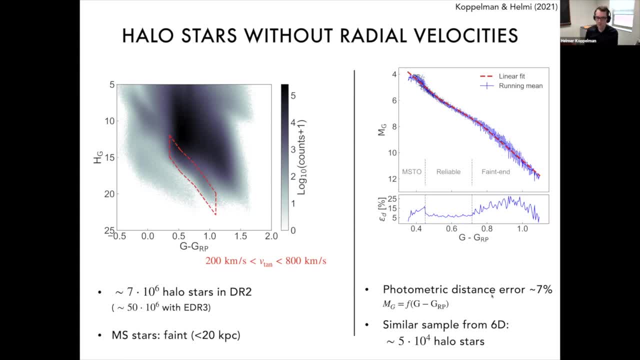 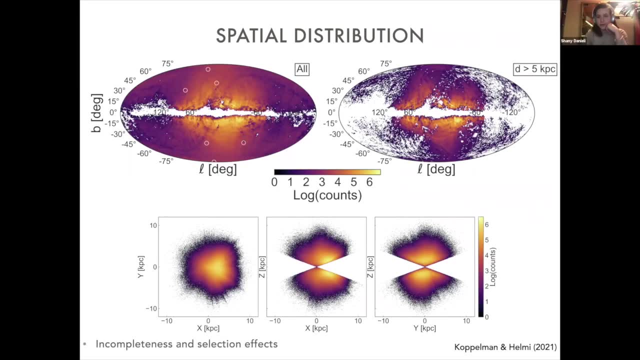 And the distance is measured by Gaia Typically. So this is a nice benefit. Can I ask something? Yeah, Yeah, Yeah. Can I ask something? Sure, Sure, Sorry. Do you know what's the purity of your sample using this selection? 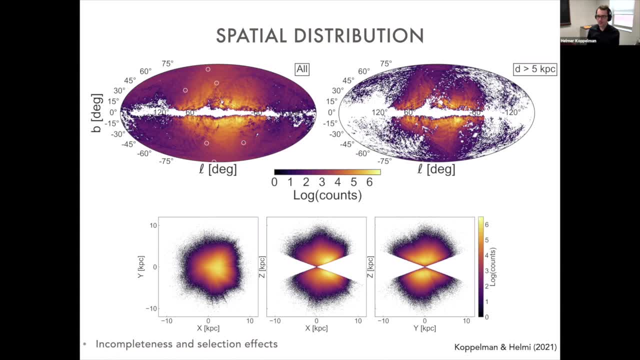 Yes, No. So for most of these stars it's really difficult to assess the purity, So we cross-matched it with Stars for which we have measured chemical elements, For example, And so there the purity is really high. So we 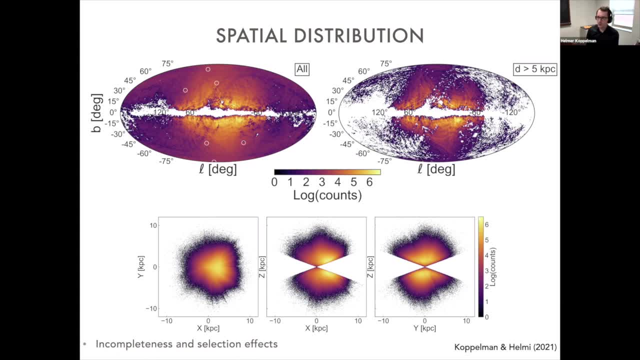 we expect that actually all of these stars are really halo stars Based on their chemical Compositions. Well, I mean, you can at least. You can at least cross-match with with stars That you have proper emotions for right. 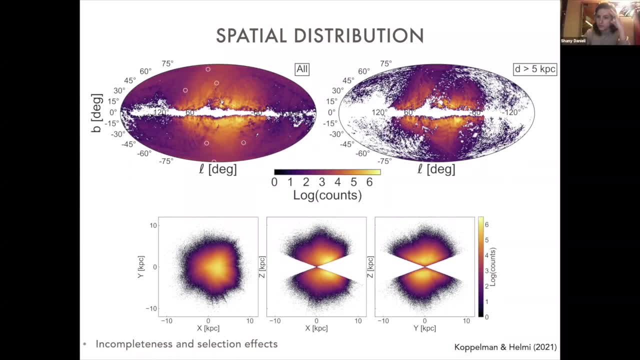 The smaller sample, but you can at least check This. 10 to the four Stars: Yeah, So for the smaller sample the purity is so compared to. so if it cross-match with the smaller sample, Then a purity is really high. 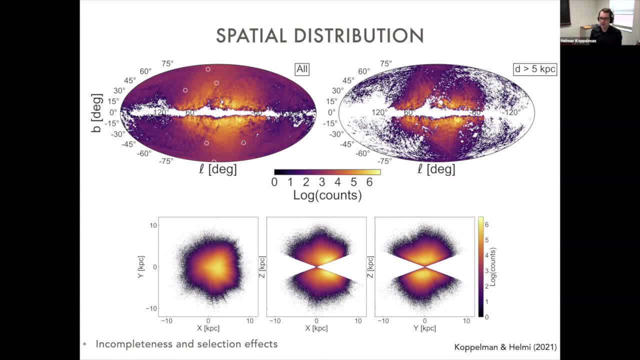 Actually, all of these stars are in halo orbits. The only issue is that only for The smaller stars. The only issue is that only for maybe 1 in 200 or maybe even less 1 in 1,000 of these stars. we actually have this additional information. 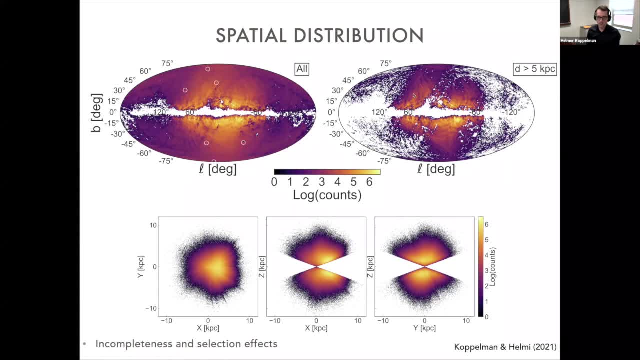 So we are extrapolating a lot here. Well, it's difficult to really claim this, but yes, I think that the purity is really high. Helmer, can I ask a question regarding this? For some of these, I assume you do have the full 3D velocities. 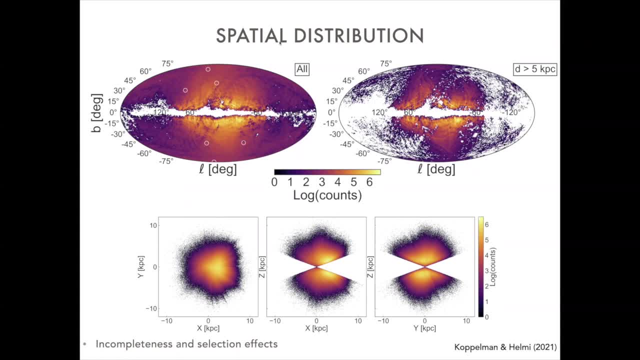 So for that set, is it possible to make a comparison to see how well the reduced proper motion method identifies the halo stars? Yeah, so that's what we did, And so the method works really well. So I don't have any plots to show this, but the reduced proper motion method does work quite well. 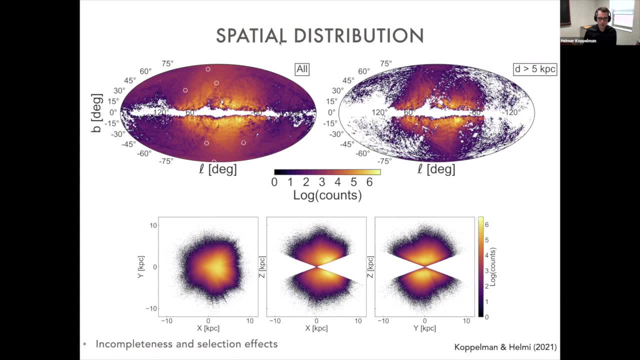 So we tested this on simulations, So mock data, but also on the actual data using this subset, for which we have the 3D velocities. Yeah Right, So this is the spatial distribution of the stars. So the top two panels show the sky coordinates. 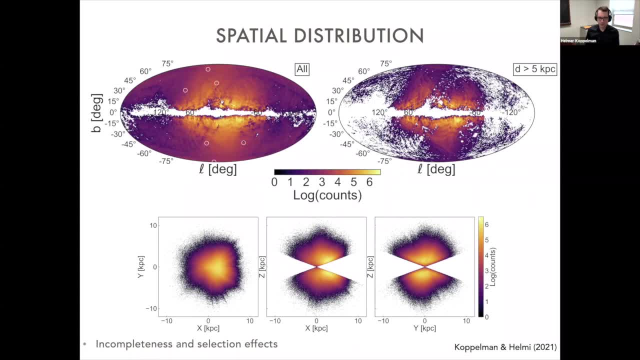 So galactic LMB, which is oriented such that the galactic center is at the center and the plane disk of the Milky Way is just kind of removed, So it's kind of the white region here, And so you see that A lot of the there are a lot of features on the sky and especially for the subset of halo, stars that have large distances, so are farther away from the sun than five kiloparsecs. the sample is really incomplete and there are a lot of selection effects. 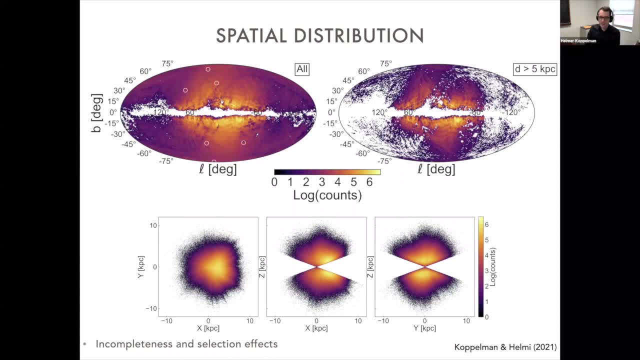 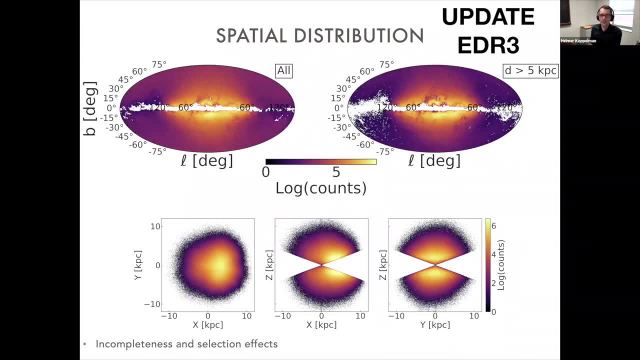 And this is just because of the quality of the current Gaia data And so this is using kind of old data. So if we compare this to what is available now, then we see that already with EDR3. The map, the sample looks a lot smoother and a lot of these incompleteness effects and selection effects are removed. 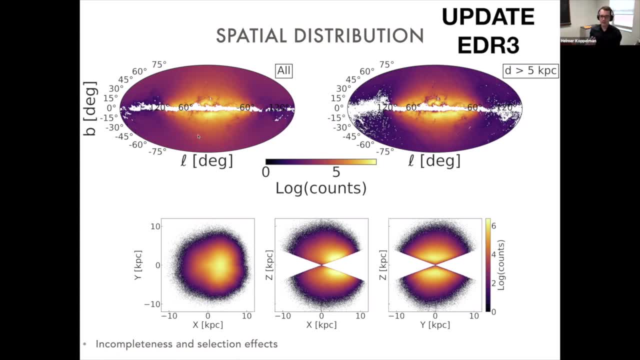 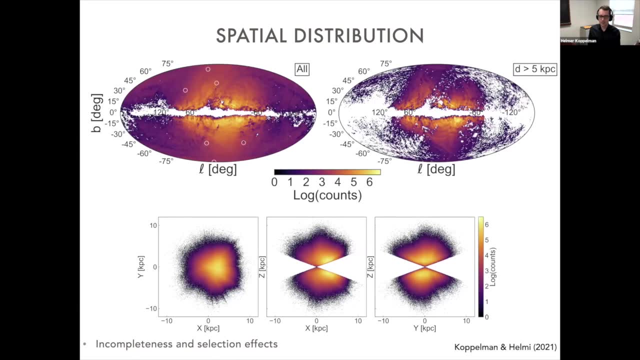 And so the expectation is that with the forthcoming data releases, we will get a much more complete sample of halo stars. So I'm just flipping back and forth to see the differences, But what I'll be talking about today, which is in the paper, is this older data set which has these incompleteness effects, unfortunately. 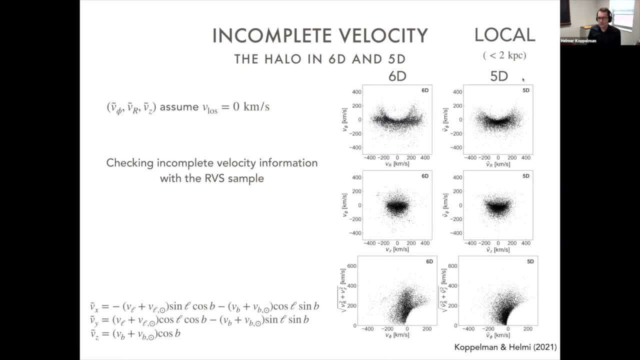 So, as I was saying, you know, for these stars there's a big issue because we have, you know, this missing velocity component. and just to give you an, a feeling of you know what the velocity distribution looks like if you kind of project it into, if you assume that this missing component is just zero, 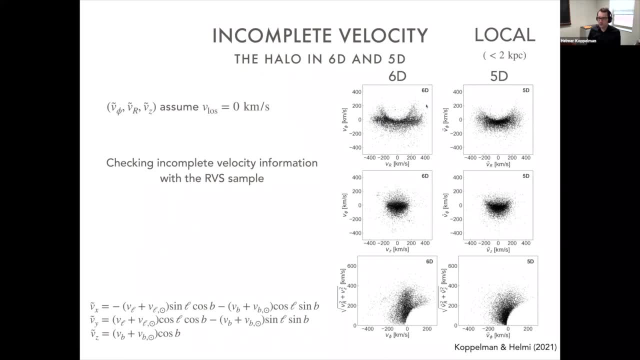 So here I'm comparing left and right the velocity distribution for halo stars, which we do have all the velocities, And so you see that the velocity distribution, if you project it into the 5D space, becomes a lot less clear, so a lot more diluted. 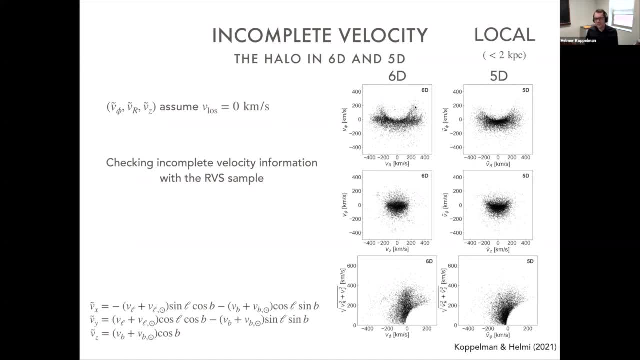 If you squint your eyes and kind of use your imagination, then you see that the overall features of the velocity distribution are kind of similar but they're a lot less clear. So this kind of selection effect here, this ring here, is still kind of present. 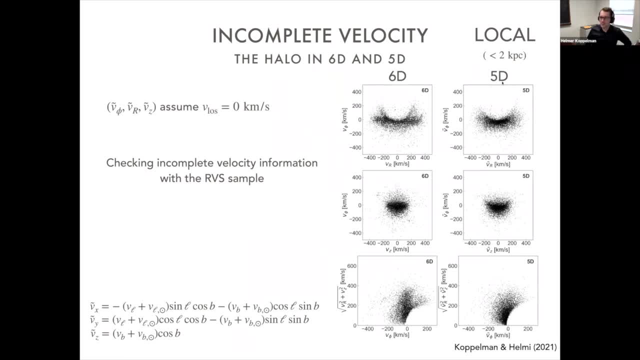 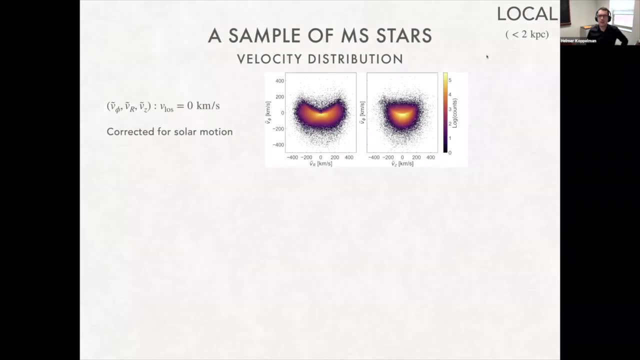 But there are. you know it's non-trivial to analyze this 5D data set, at least looking at the velocity distribution. So I'm showing here the velocity distribution of these main sequence halo stars for stars that are for a subset, a local subset, for stars within two kiloparsecs. 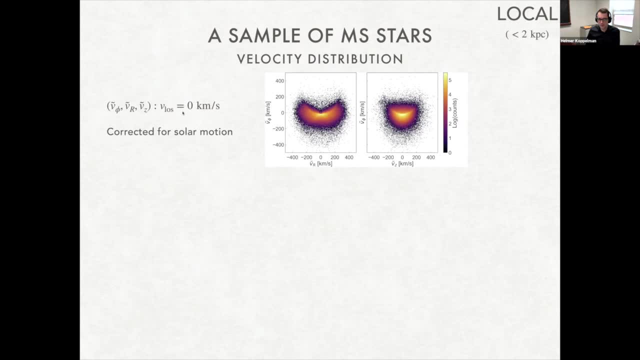 So this is the velocity distribution, assuming that the line of sight velocity is zero. And then, so what you see here? the sharp edge which is even more prominent on the right. this is just the selection effect. this is just the effect of selecting halo stars. 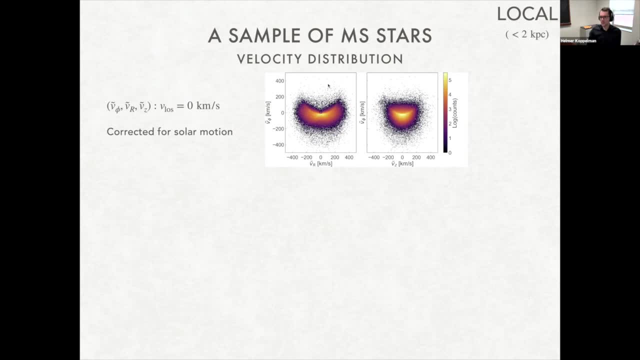 So in the empty region here, this is kind of where the disk is, which just has been removed by selecting halo stars. So this is just the selection effect. Then what else you can see is that the velocity distributions are pretty smooth. It is elongated in VR and this is completely expected. so we do see the same elongation in a 60 sample and this is actually the elongation, is actually indicative of debris from Gaia Enceladus. 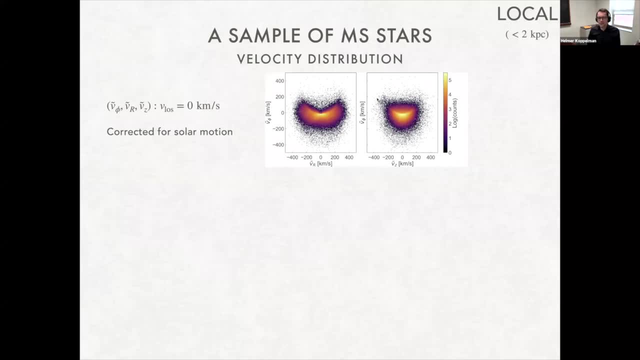 And again, if you squint your eyes then you can kind of see an over-density here, so it's not completely symmetric. So what we did is we actually we calculated the asymmetry in the velocity distributions And so what you see is that there is a strong asymmetry here, but overall the velocity distribution seems pretty symmetric, with some local asymmetries, especially in the retrograde part of the halo, which is the bottom side of the panel. 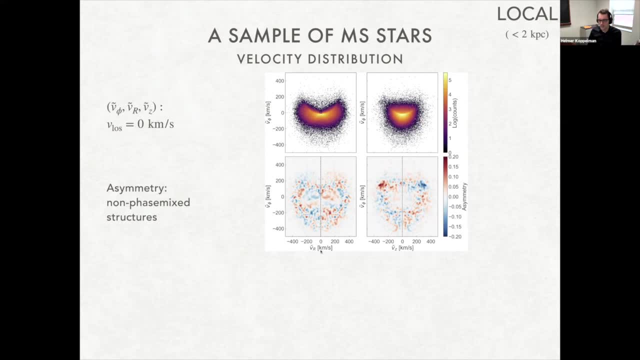 Stars tend to be have a positive radial velocity and a positive z-velocity, And so we wanted to understand what's causing these asymmetries, because, for you know, a Milky Way that's in equilibrium, you expect the distribution to be symmetric. 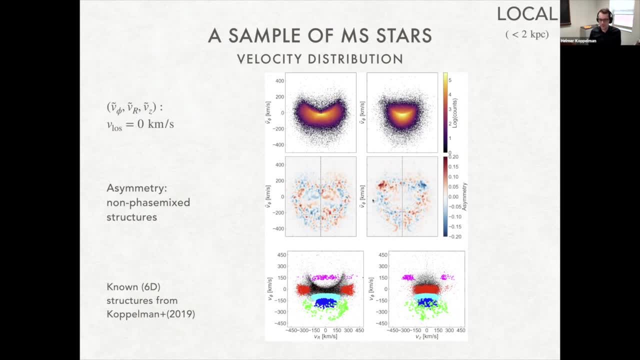 And so we think that actually all of the asymmetries that are observed here can be explained from structures that were already detected in the 60s, and that's why we did a much smaller 60s sample, For example. here I'm showing the 60 distribution: velocity distribution. 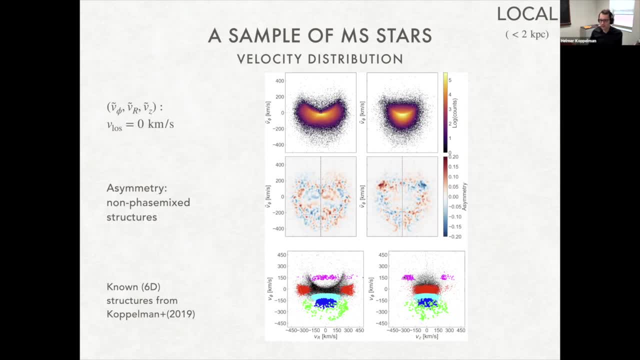 And so, for example, the stars in magenta here. this is a structure that is originating from a dwarf galaxy that emerged from the Milky Way, that was already discovered, And it has an asymmetric velocity distribution that corresponds to this asymmetry seen here. 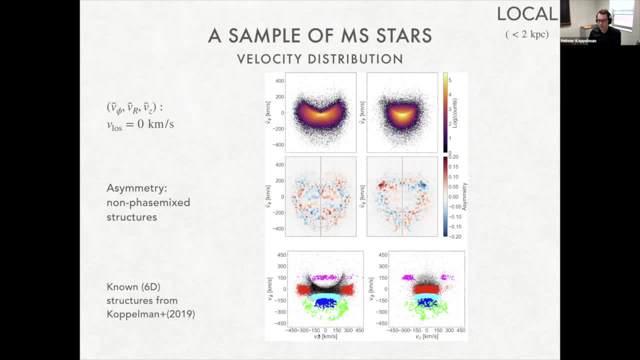 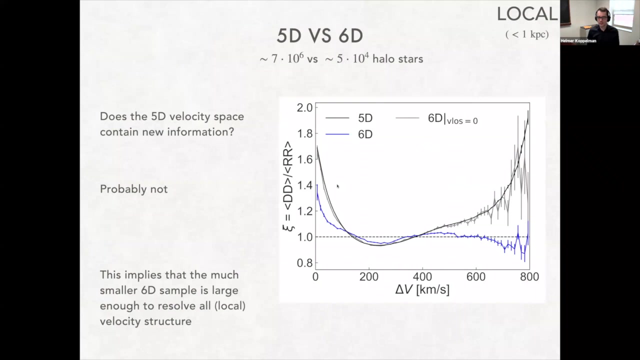 And the same for the stars in lime, the green ones. These are distributed asymmetrically in the true velocity distribution, which likely corresponds to the asymmetry seen in the 5D distribution, And so one question that you can ask is: you know? we made this trade off between using incomplete velocity information. 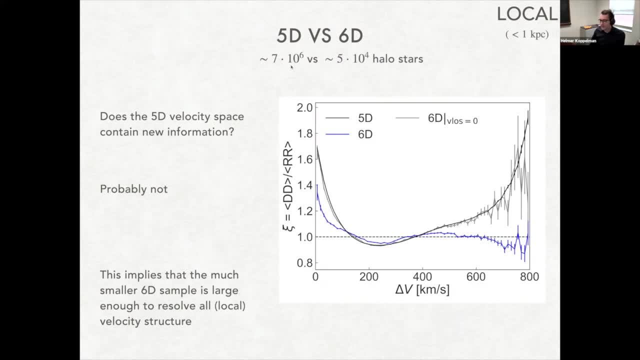 but having a much larger sample, did we actually gain some more information? Was it actually a useful way to select halo stars? No, It's not. It's a very simple question. but it's a very simple question And the kind of disappointing conclusion, at least for a very local sample, is probably not. 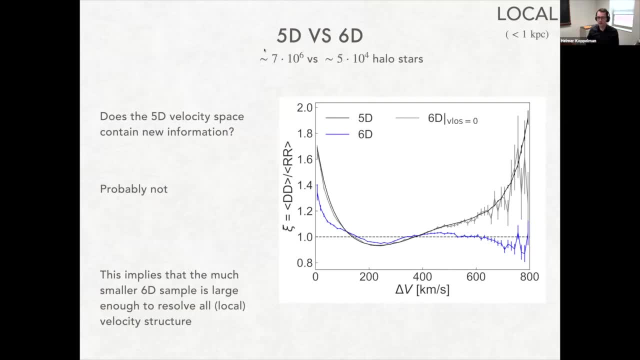 So the further you go away from the Sun, the more you gain by having this larger number of stars, just because you need, just because with galactic or with heliocentric distance the number of stars quickly drops. But for the local sample we tested this with a two point correlation function in velocity space. 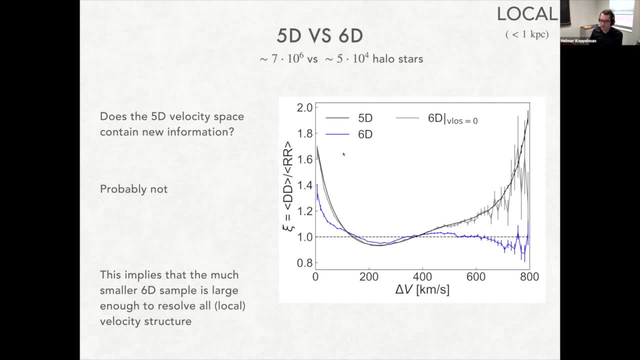 And so if you look at the small scale velocity, the velocity structure in the halo locally. So for the 6D and the 5D data there is a difference. So the blue line does not correspond to the black line, but that's because the two point velocity correlation function is measured in two, you know. 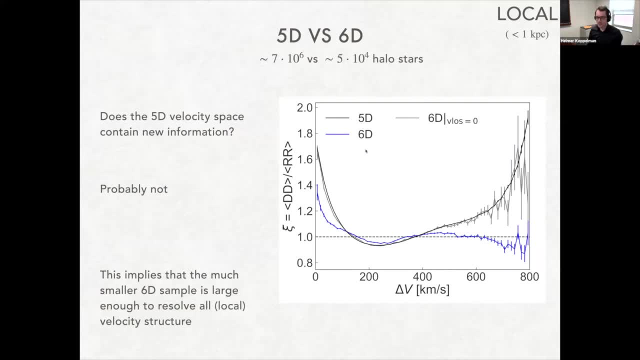 In the 5D dataset it has just two velocity components, while in the 6D it has three velocity components. So it's not a fair comparison. So what we did? we projected the 6D sample into the yellow line. 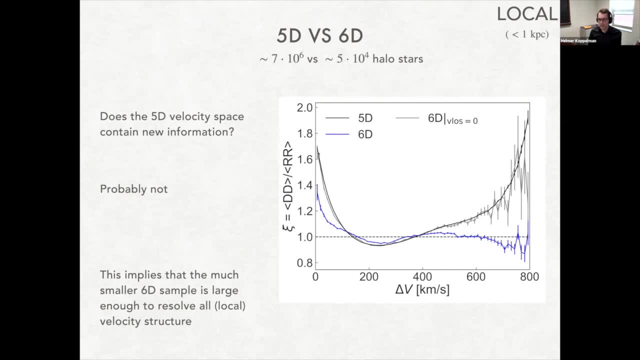 So it's not a fair comparison. So what we did? we projected the 60 sample into the yellow line. So what we did? we projected the 60 sample into the yellow line, into 5D space, which is the gray curve. 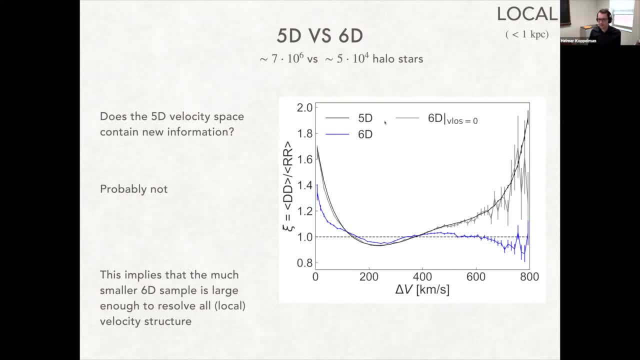 which almost exactly overlaps with the 5D observation, which is just a difficult way of saying that by selecting this 100 times more stars, we didn't actually gain a lot more statistical information, which is, in a way, kind of a disappointing conclusion. 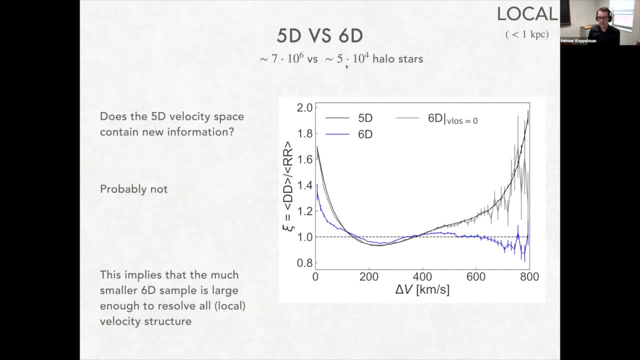 but it's also a positive conclusion because it means if you use this much smaller 60 sample, you can already use this to do a quantitative analysis and you can use it to do statistical studies Already. all the structure that is found locally at least, is present in this much smaller sample. 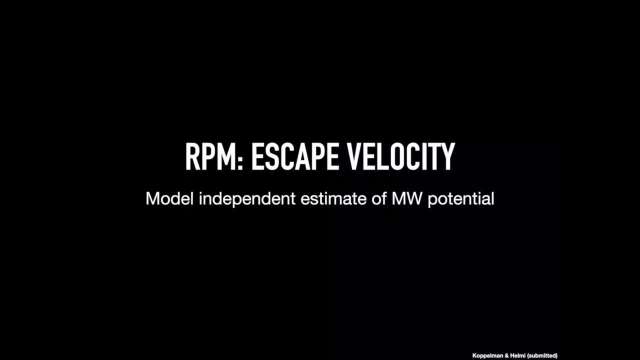 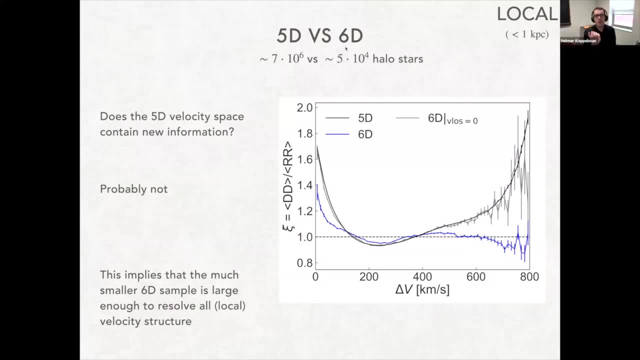 Sorry, can I ask? I didn't get the logic. So the two curves are the same. and why is that good or bad? I didn't understand. So we're wondering if there's any information in the small scale clustering of velocities of halo stars. 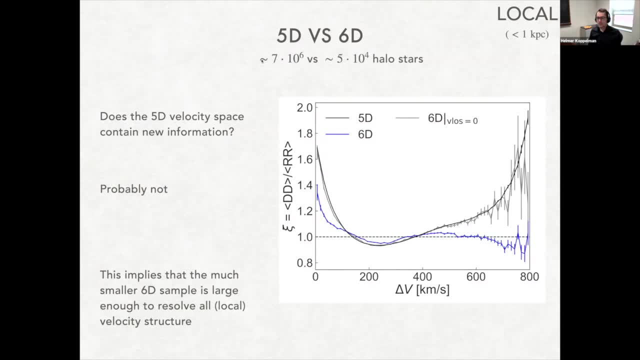 if there's any new information in the much larger data set. So one way to test this is using the velocity correlation function. at least, that's what we did. But what were you looking for? That the shapes would be different or that the error bars would be smaller? 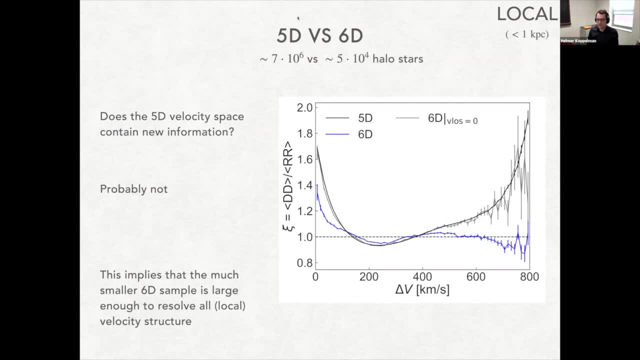 We were looking for more, so an excess of correlation in the 5D data set. So we were hoping that by having this much larger sample we would find more correlation in the velocities than in a much smaller data set. So the one of the questions we had was: 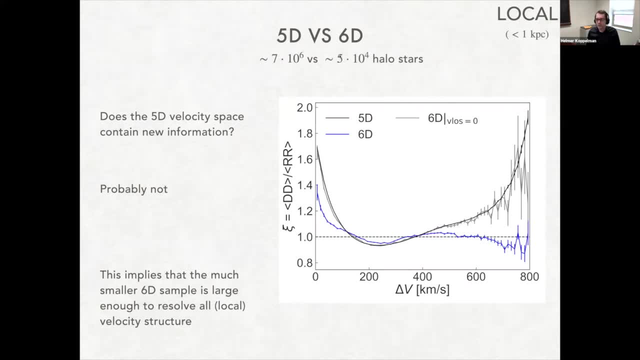 if you look, if you take this smaller sample, then one of the issues might be is that you're not resolving all of the structure that is in the velocity distribution. So maybe you're not, you're only resolving like the big structures but not the really small structures. 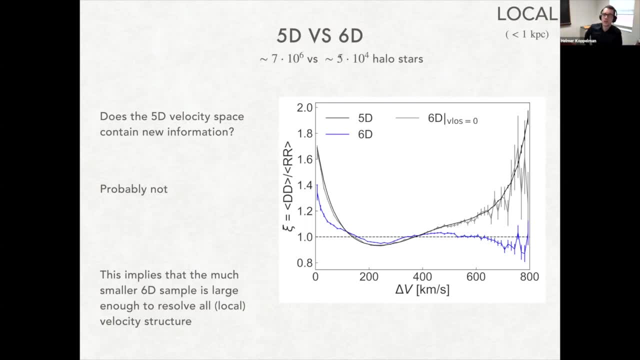 And so actually we think that the already the 60 sample is large enough to resolve all of the structure there is in the velocity space. Your error bars in the big sample are in fact much smaller. It's just that the structure of the curve is simple enough. 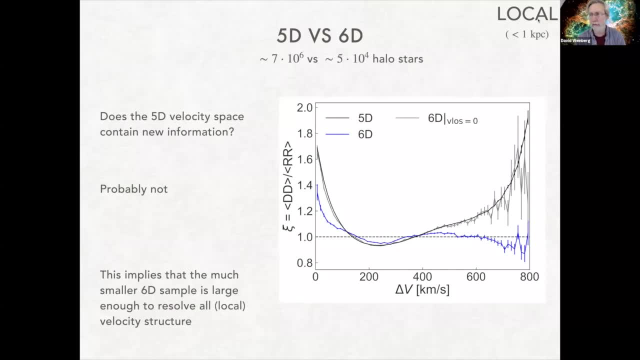 that you're not getting new physical insights from those smaller errors. Right, yes, Yeah. But, for example, because the correlation function seems like a blunt tool, like if you have a satellite or something that you expected to see in a simulation or something a much bigger difference if 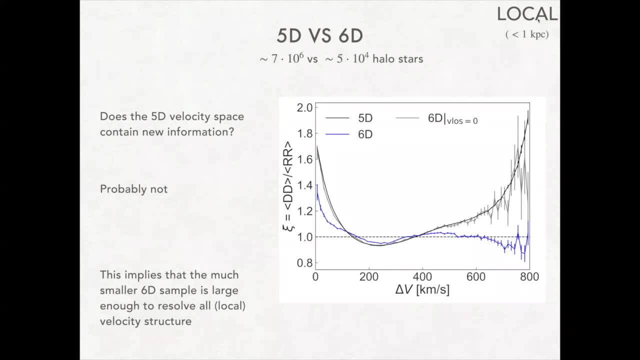 or a big feature that you're not seeing here, or because, if it's just a small fraction of the stars that are contributing to your structure, maybe this just doesn't see it because of that. Yeah, Now you're right. So it is a very blunt tool and it's just a comparison. 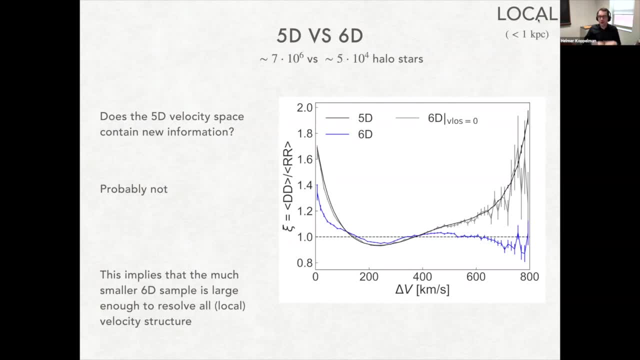 to see if there is any more information in this larger subset. So we're not looking for something specific, It's just a comparison of the two data sets. That's all. So to answer your question. Okay, yeah, thanks, Okay. So one application of this right, Yeah, I guess. So one application of this right. So one application of this right. So one application of this right. Yes, Yes, yes. Is there anything else that's interesting? 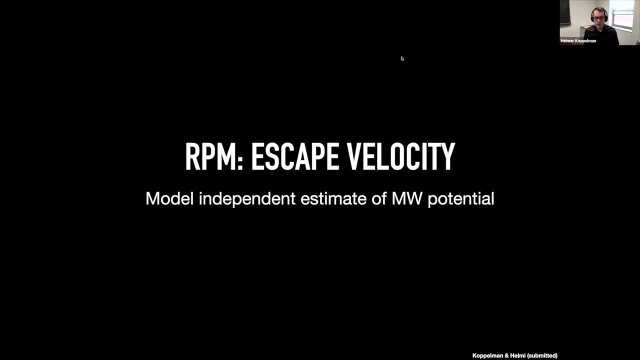 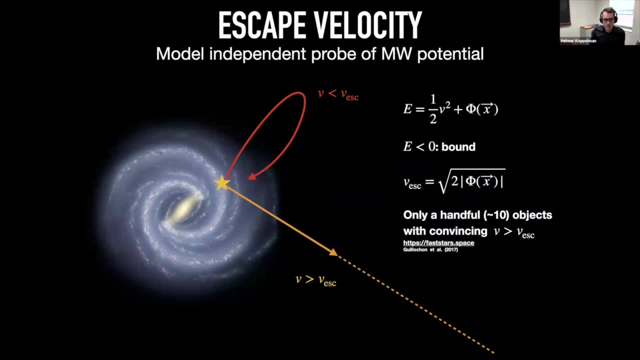 We're good. Okay, Thank you. Okay, Thank you so much for the presentation. Yes, thank you, Thank you, Thank you. a sample of halo stars is to determine the escape velocity of the Milky Way, And so the escape velocity is just simply what you expect it to be. It's the velocity that you 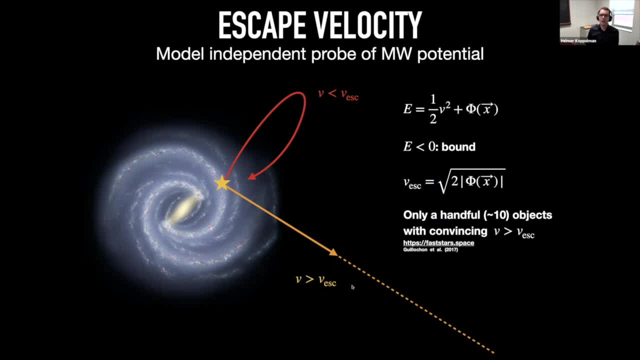 that a star needs to escape the Milky Way, And so you can define it from the energy equation. So this is: the orbital energy of a star equals the kinetic energy plus the potential energy, And so typically the potential energy is defined such that the orbital energy of a star is smaller. 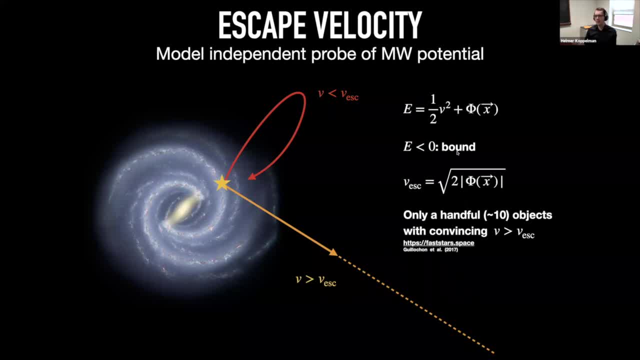 than zero for stars that are bound to the Milky Way, And it's larger than zero for stars that are escaping the Milky Way. And so, by setting the energy to zero, you can find the velocity that is required to escape from the potential energy, So you can find the kinetic energy that 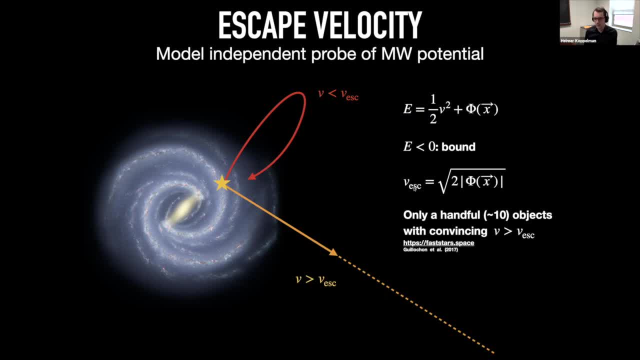 is required to overcome the potential energy which is defined to be the escape velocity. And just a side note, So typically if you look at the stars in the Milky Way, then almost none are escaping. So there are only a couple of a handful of objects which 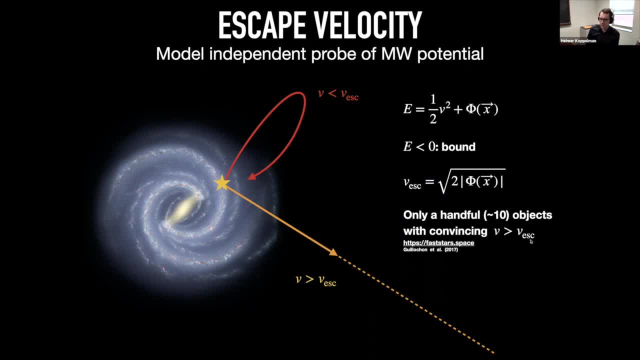 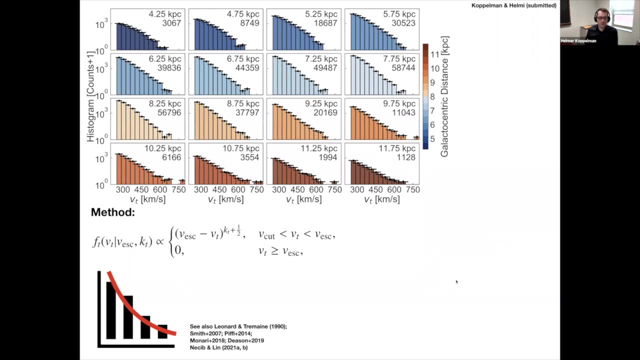 have convincing velocities which are much larger than escape velocity. So it's very uncommon that stars are actually escaping the Milky Way- At least we think so. So so a lot of so. there's a rich literature on determining the escape velocity of the Milky Way. 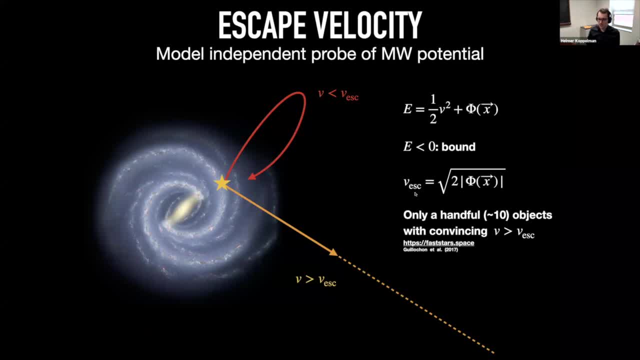 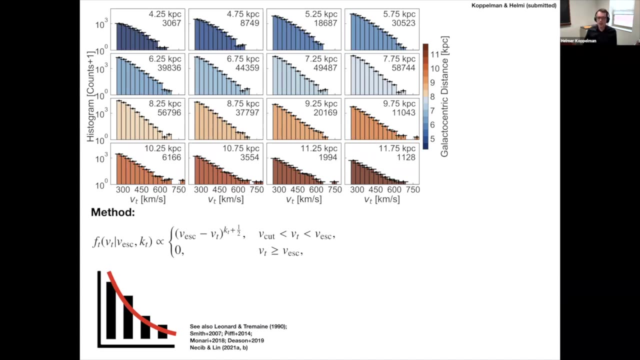 And so yeah, so the way why it's interesting actually to do to measure the escape velocity is because it's a direct measurement of the potential of the Milky Way, which is something that we don't exactly know, And so a lot of people have worked on determining the escape velocity. 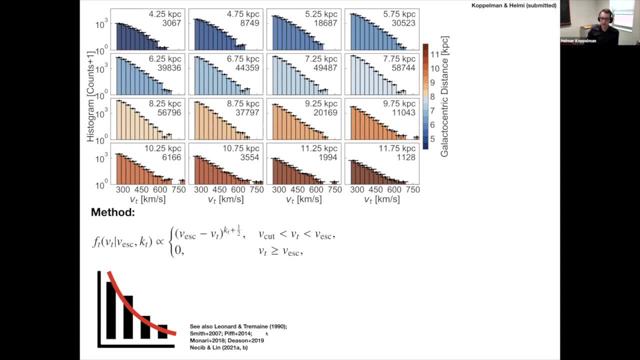 And I think one of the, if not the first, paper on on a method to determine the escape velocity is by Lennart and Germain. And so the method is to not just look for the fastest moving star but actually to model the distribution, the the tail of the velocity, distribution of halo stars. 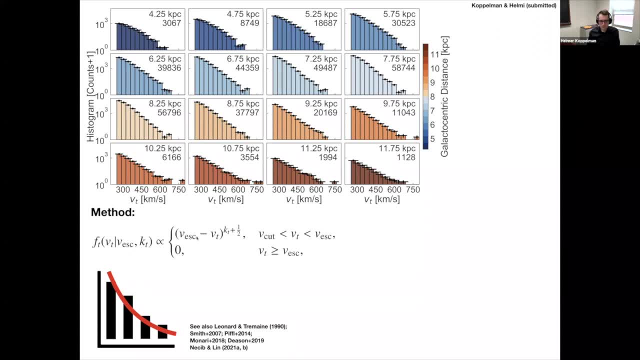 And that is to model it as a power law. So just a simple parameterization of the escape velocity and an exponent of the power law k, And so by fitting this functional shape to the velocity distribution, you can find the parameterized escape velocity. 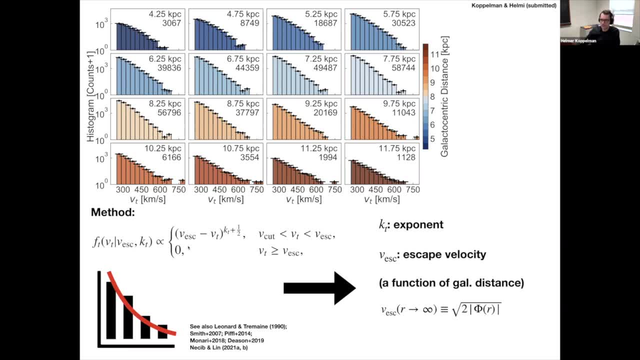 Which is just, you know, at the point where the distribution goes to zero. Just one quick question. So you said any physical reason why it should be a power law but not the other form? So not, it's just the simplest assumption you can make, especially if you look before. 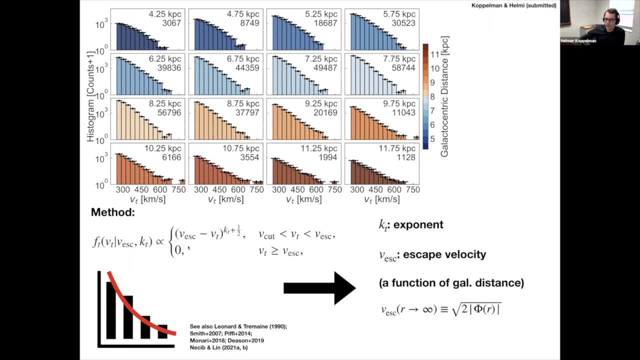 really be the end of the tail of the velocity distribution. it's just the simplest assumption you can make on the shape of the tail of the velocity distribution, Right? so, as I said, if you can observe the escape velocity or determine escape velocity, 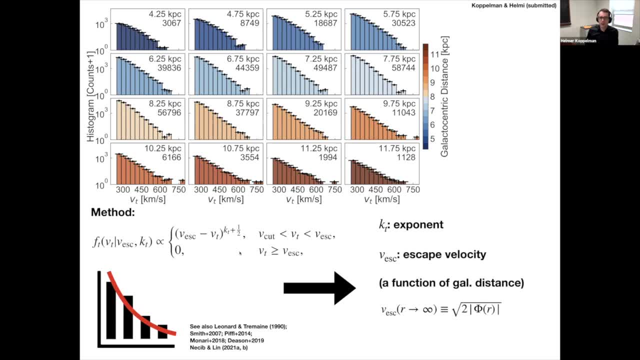 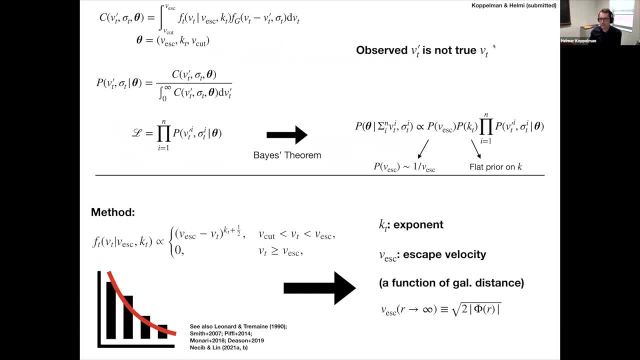 you have a measurement of the potential of the Milky Way. Of course, there's a minor concern, and that's that the observed velocities are not the two velocities, but there's an uncertainty term. So one way to model this is to convolve and to treat the uncertainties as Gaussian distributions. 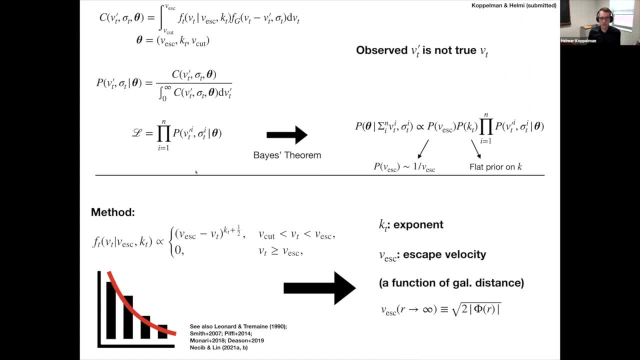 And so just to kind of skip this, but we use, we set up a likelihood and then we convert it, using a Bayes' theorem, into a pretty standard Bayesian method to infer the escape velocity and the other parameter, the k value. And so we ended up using: 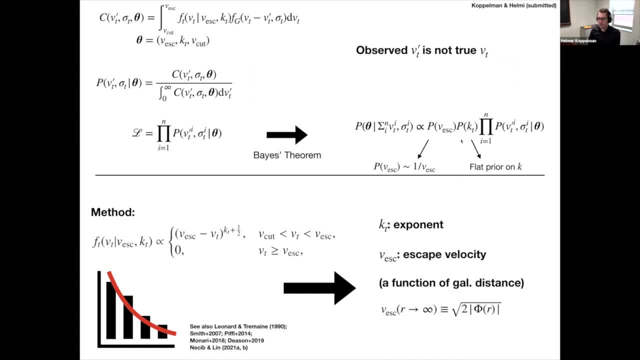 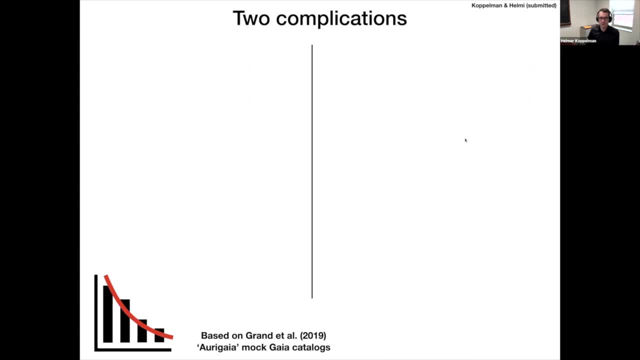 some simple priors, but actually the shape of the priors does not really influence the results. So there are two major complications with this method which people are trying to work on overcoming, but I don't think so. it's not so. these are just two kind of complications. 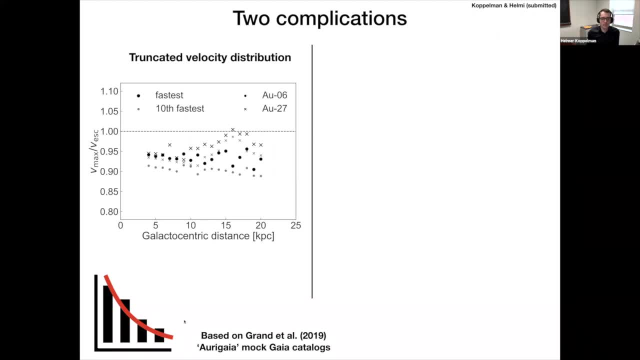 that are born into the method, And so one of them is that if you look at the velocity distribution, then the maximum value that it can reach is the escape, the velocity, But there's, of course, no guarantee that it actually reaches this maximum value. 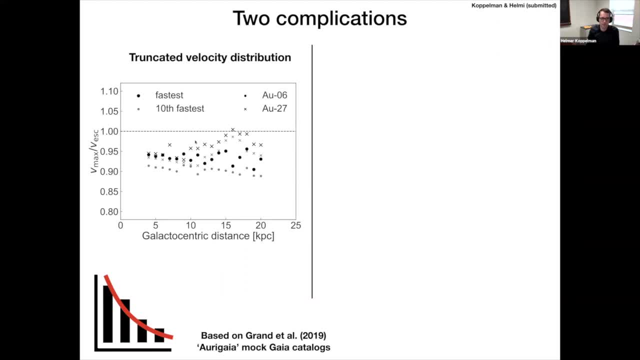 The velocity distribution might as well just be truncated below the escape velocity, And so this is actually where we find if we look at cosmological simulations, and so I've been using the mock Gaia catalogs, but also other people have looked into this. 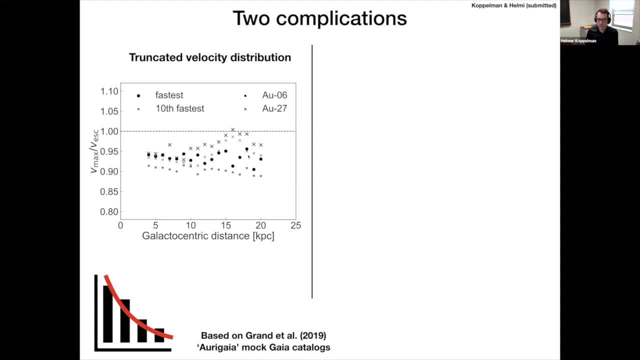 So typically what you see is that the fastest moving star in simulations is at the five or 10% level of the escape velocity. So typically what you see is that the fastest moving star in simulations is at the five or 10% level of the escape velocity. 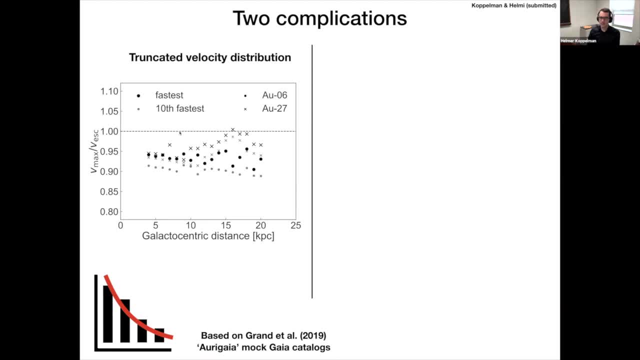 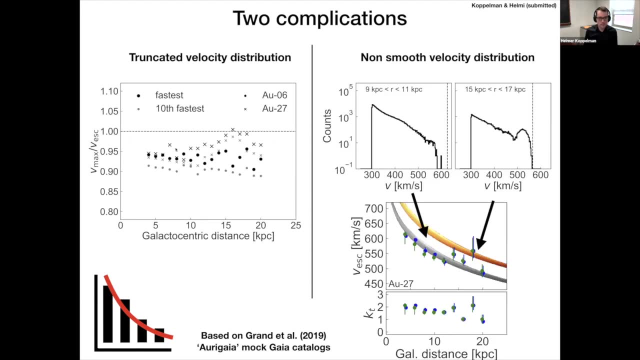 And so this means that if you determine the escape velocity, then it's not actually the true escape velocity, but it's slightly lower just because of this effect. And then there is another complication, And that is that the you know the functional shape that we assume for the tail. 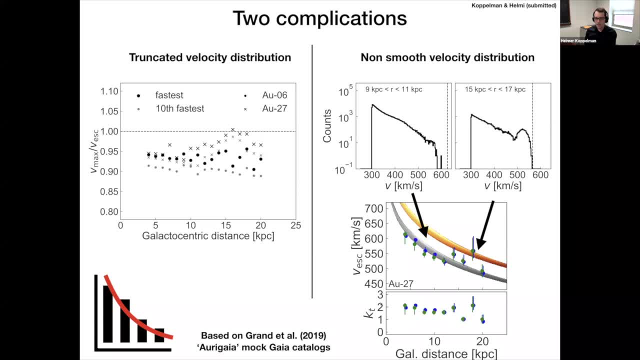 of the velocity distribution is really simple and smooth, And this does not have to be realistic. So the velocity distribution does not have to be smooth, and so in this particular simulation that we analyzed, there was this bin where the this velocity distribution has this kind of, you know, bump in the profile. so it's clearly not a 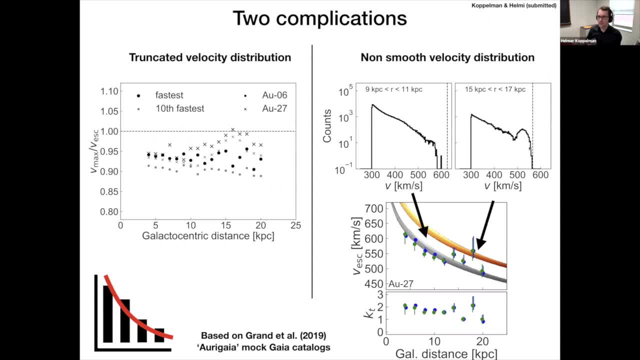 smooth profile and so this will bias the inferred escape velocity and currently people are trying to, you know, think of ways to or create ways, methods to overcome this issue. but you know the results that i'll show in the next slide. this is kind of the issue we have to deal with helmer. i have 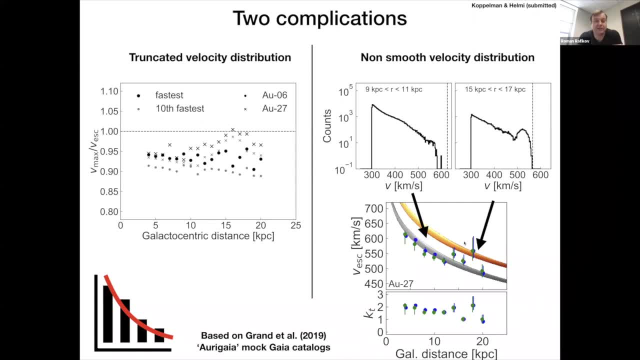 a question. so in this case, do you have enough statistics- i mean enough particles in simulations to get statistics basically reaching to this escape velocity point, or maybe you don't have enough particles and that's just you know kind of short noise that you're getting and how does it? 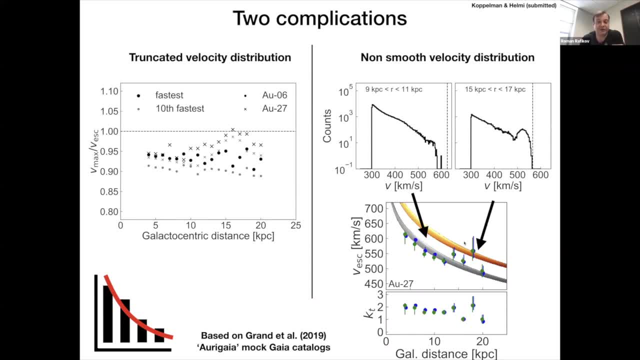 compare actually to the real sample that you will have when you look at the halo stars. how do the number, how do the numbers compare right? so the the specific uh mock catalog that i analyzed is designed to resemble the gaia catalog, so the number of stars are similar. 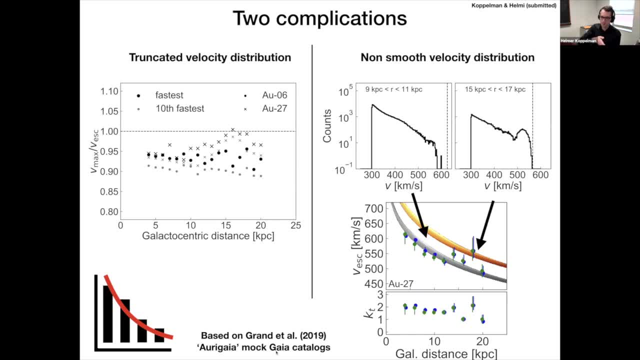 and also downsized it such that it matches kind of the stars per bin that we have in the data. so there there can be two explanations for this. one is that we just don't have the resolution to resolve the stars reaching the escape velocity, and the other one is that there is no guarantee. 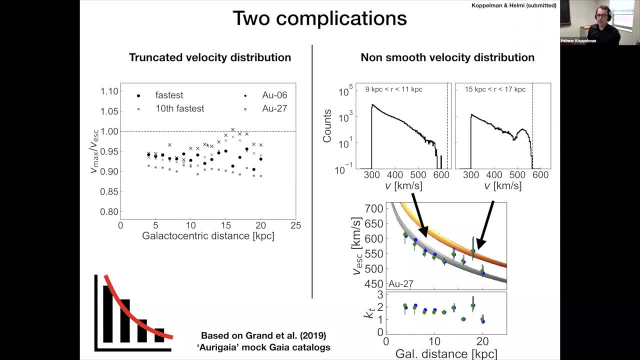 that actually has to reach the escape velocity and of course you know this, these specific values are for the simulation and we don't know for the milky way, uh, what the effect is, but given the number of stars that we have measured in the milky way, uh, this is what we think is, uh, kind of a. 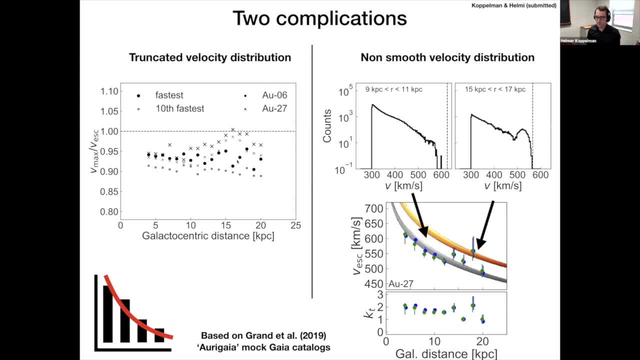 typical truncation that we might find. so we think that these are fair numbers. yeah, okay, thanks, all right. so what's the origin of that bump? is there, it was there a merger in the simulation? this here: yeah, yeah, yeah. so this is actually, it's a merger, so you can actually see in the 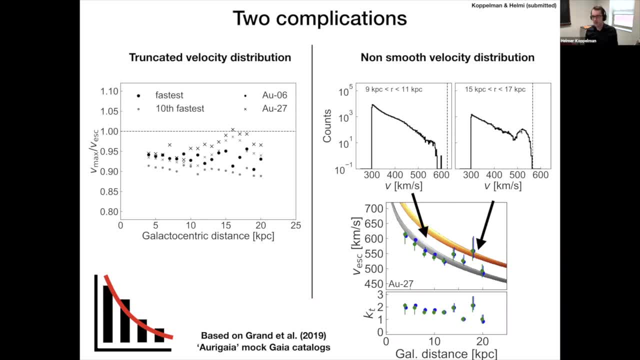 spatial distribution of the stars. you can see that there is this um, uh group of stars, a merger, uh, flying past the, the, uh, the sun, kind of yeah, and so here i'm just showing quickly what, what, the, what kind of escape velocity is, the method determines for the simulation. so the, the orange banana here. 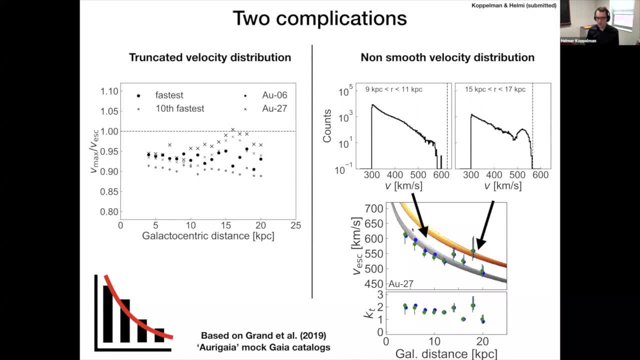 this is the true escape velocity, which we know because it's a simulation and the markers here indicate what the method determines. and so the the gray, uh contour is just the, the orange one, but offset by ten percent. and we see that the determined values typically are offset by ten percent from the two true value, except for in this region here. 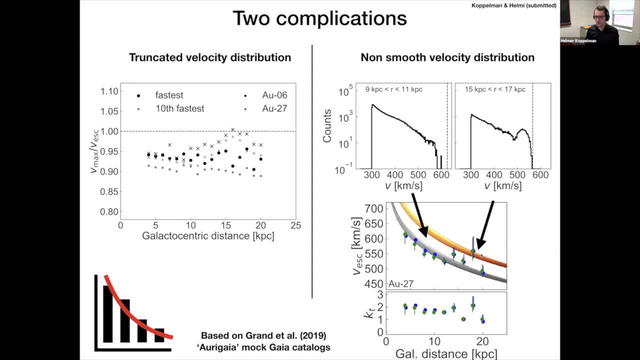 where there is a clear kind of bias in the determination of the escape velocity. and so this bias we think is- or, uh, we show is actually because of this, uh, clumping of stars in the plastic distribution. but this is kind of what we would expect for the milky way. how does this? how? 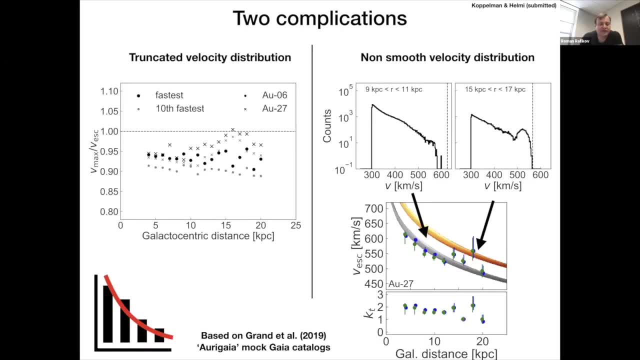 does this catalog actually works? i mean, you have a simulation with certain resolution, right? i mean, what is the mass of particles in this simulation? right? so the the simulation. it's actually very similar to the the plates simulation, right? so the the simulation is actually quite similar, but the 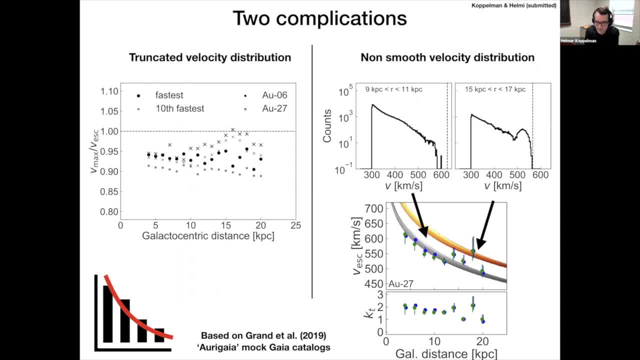 has a much lower resolution than the. the guy data. yeah, and so the stars have been artificially kind of the. the star particles have been artificially split into multiple stars to match the. the number of stars in the diagram are they? are they given some velocity dispersion within each? i mean what? 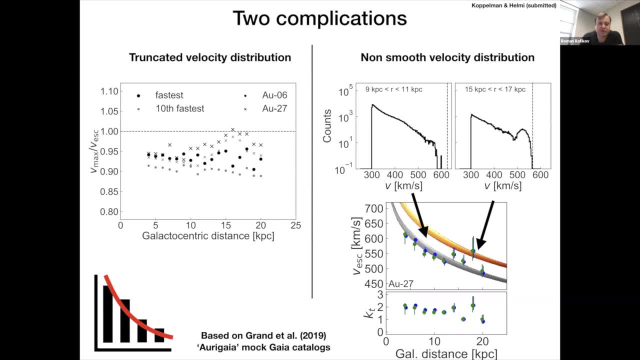 is it? what is the mass of the particle in the simulation, right? so there's, as you're hinting, that there's. one issue is that you know, if you split a kind of a velocity particle, multiple stars, you get stars with which all have the same velocity, and so there are two methods to do this. 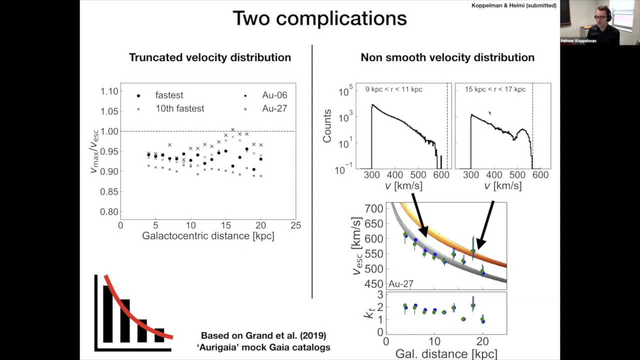 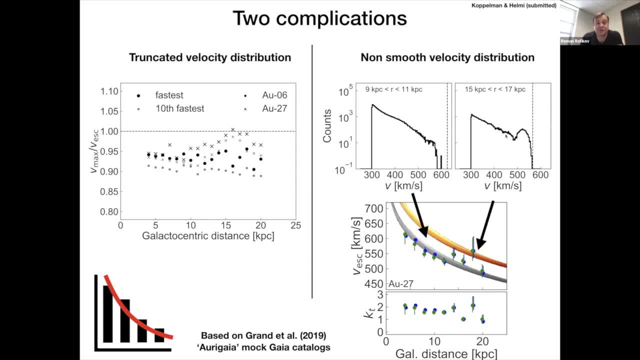 in your simulations. they would act like sort of like molecular clouds, so they might actually give you some. i mean two, body relaxation maybe. i mean, of course, velocities are pretty high, but still something like that could be happening and pushing some of your stars across this watershed at the escape velocity. so i i would be curious to see you know how. 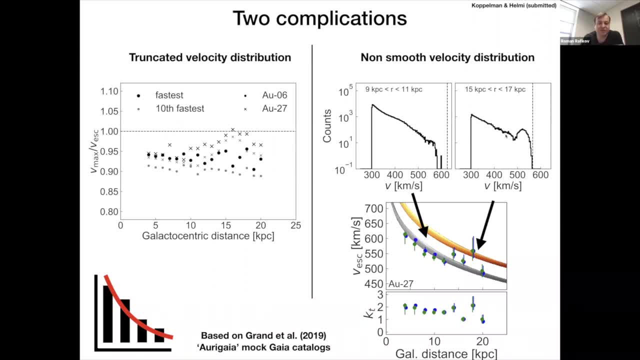 this picture would change as you vary the resolution in your simulations, as you, you know, decrease the size of simulation particles in your simulation in in these simulations. yeah, that's a, that's a good call and i don't have any answer for that. i think that's one of the 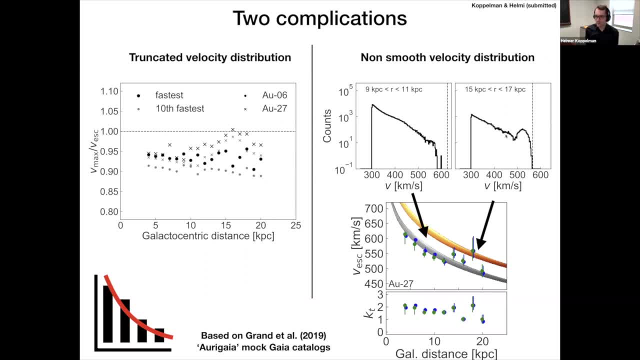 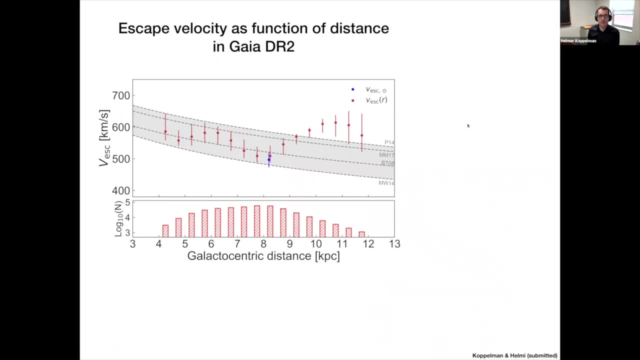 things that people have been struggling with with using this method is that typically, simulations don't have the resolution that you need, um, so yeah, i don't have an answer for that, but yeah, that's one of the the concerns with the method. right, i'm just going to suggest along the lines of the room. i'm just asked. you know, it's easier. 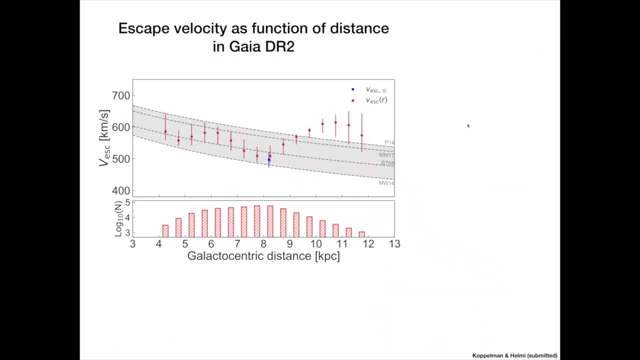 to lower your resolution, of course, than to increase the resolution of your simulation. so that's one of the things that people have been struggling with with using this method is to increase it. so if you see any kind of emergent trend as you lower the resolution, then, uh, that's another way of potentially diagnosing the effects of insulation. 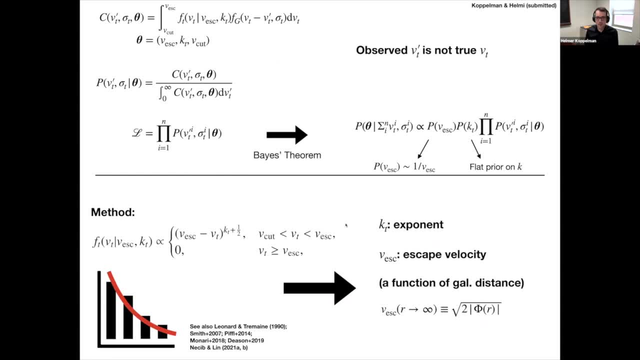 right. so one of the issues with lowering the resolution is that the um, if you look at the, the parameters of the power law is that if you have too few stars, if you lose inference and the parameters become degenerate and so you don't have a good handle. 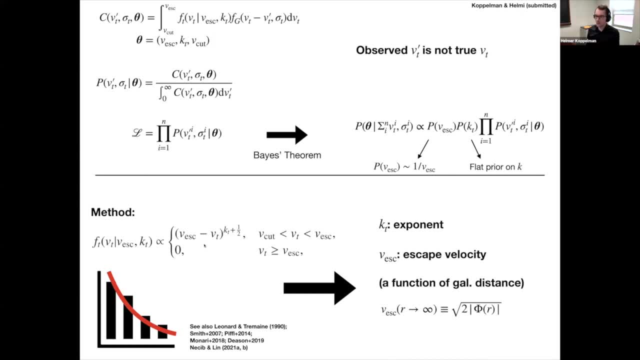 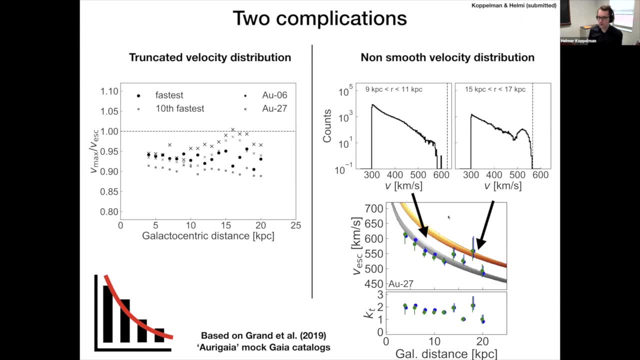 on the determined escape. so the uncertainties and the determination become really large. you do need a base resolution to get uh or an accurate determination. otherwise you need to impose a really strong prior on k, for example, which is what people have done in the past. so most of the results have. 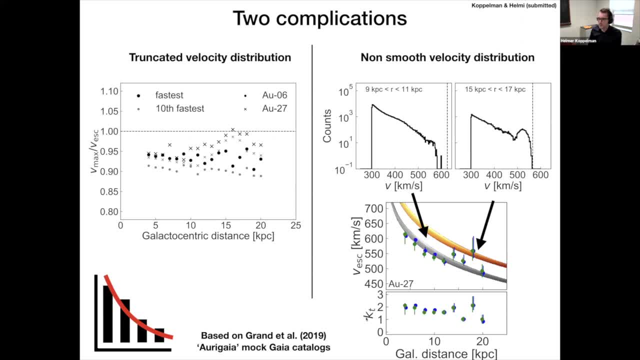 imposed a really strong prior on the exponent, just because both the simulations and the data don't have the resolution that is necessary to, uh, infer both of them at the same time. right, but so actually the benefit of having this, you know, sample of millions of halo stars that i was. 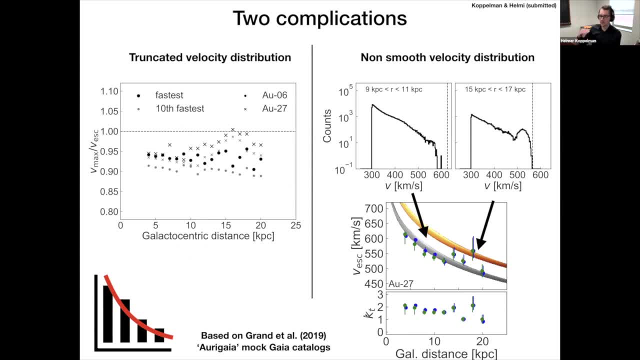 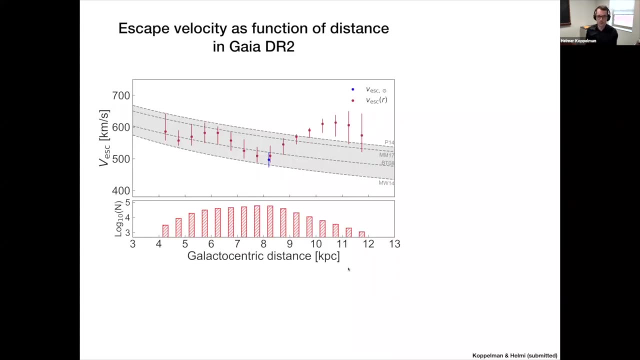 just discussing previously, is that we do have a lot of stars, and so we do have the inference power to determine both the escape velocity and k at the same time, simultaneously. so that's kind of the novelty of what i'm showing now, actually. so this is finally the the results. uh, so the determination of the escape velocity for different 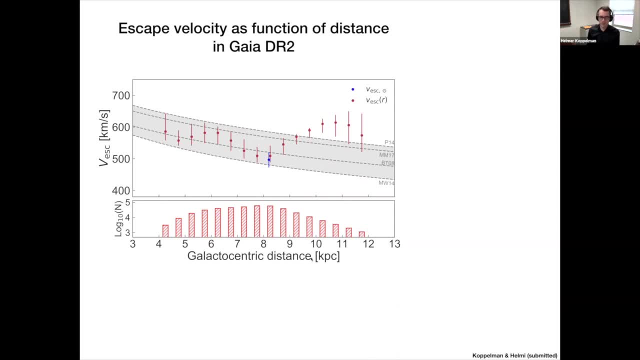 distance bins in the Milky Way is a function of galactic centric distance, the blue marker here. this is the escape velocity at the location of the sun, which is roughly 500 kilometers per second, and then in the background i'm showing the expected value for a couple of uh так. 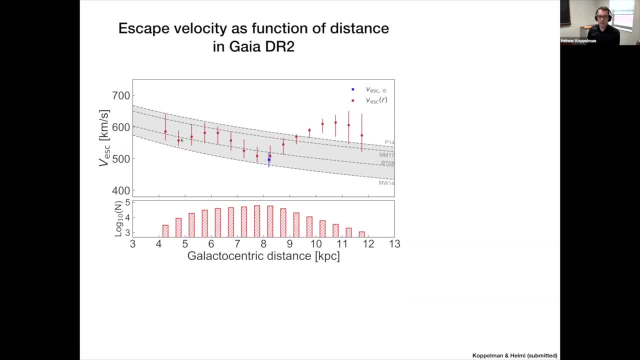 milky way models. and so you see that the expected behavior is that the escape velocity gets higher towards the center of the Milky Way and then the expected behavior is the escape velocity is higher towards the center of the Milky Way and then the expected behavior is the escape velocity gets higher towards the center of the Milky Way and then the expected 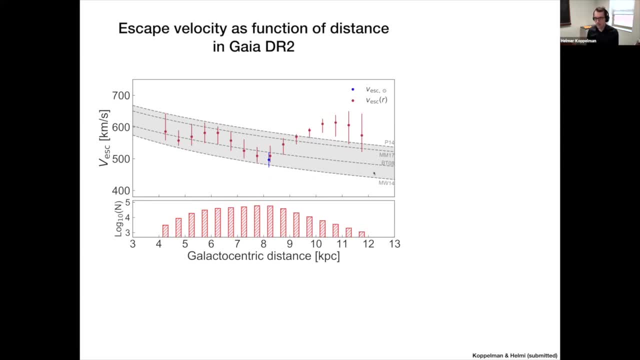 is also that it drops if you go move further outward And you see that this does not. it's not happening. Actually, it reaches a maximum of around 10 kiloparsec, which is a major concern. It should not be happening. 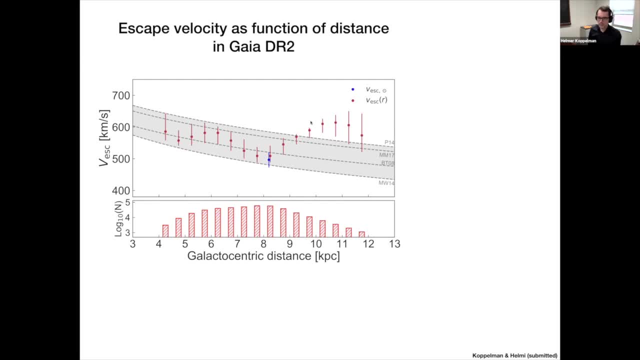 So something is biasing our results here, Something is affecting our determination here, And so the reason why I was showing this simulation, of course, is because we're seeing a similar effect in the simulation that I was discussing previously, where the estimate of the escape velocity is biased. 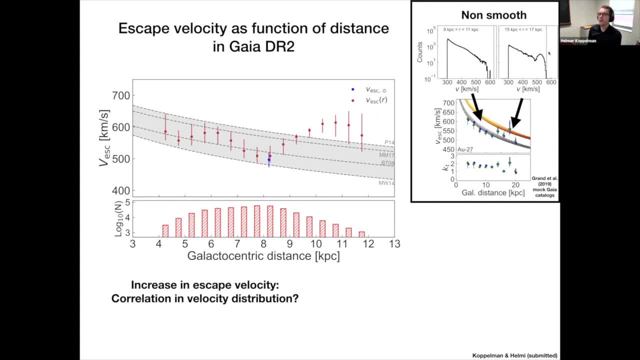 just because the velocity distribution is not smooth In the simulation. this is easy to investigate because there are no uncertainties and we have the true velocity information In the data. this is a bit more difficult, So we again tried to do this with the correlation function. 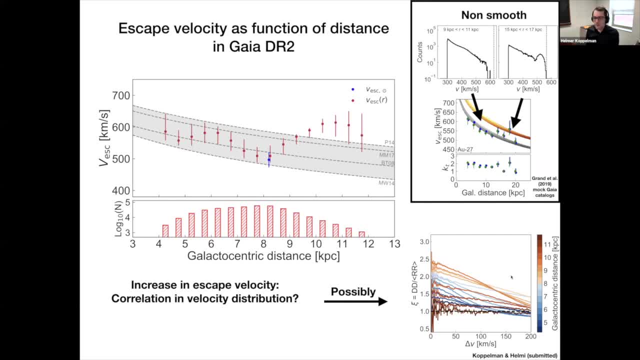 This is a little bit hand-wavingly and very blunt tool. We do find that in the orange lines here, which are for stars and the distance bins, just in the range between eight and 10 kiloparsec, they show an excess of correlation in the velocities. 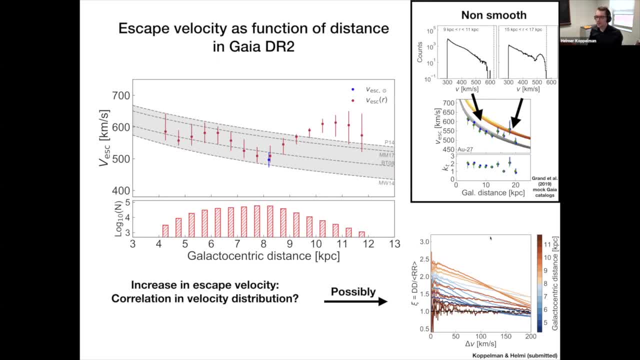 implying that the velocity distribution is not smooth, but the access is relatively small And so we don't really. we think that this increase in escape velocity is because the velocity distribution is not smooth and there's an evolution in the velocity distribution as a function of distance. 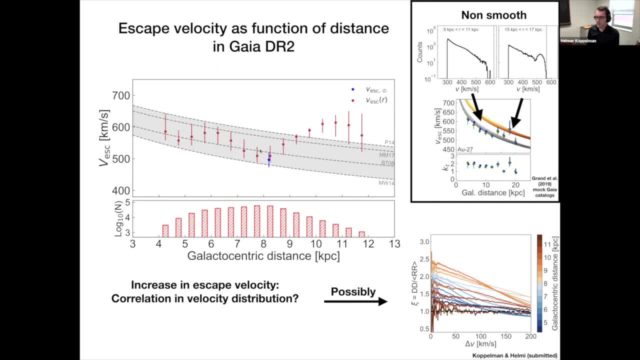 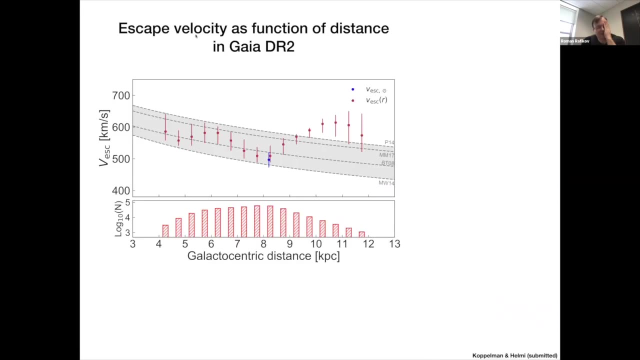 but we don't quite know, And so this is one of the issues with the method, And so, yeah, that's where we are at at the moment. So, as I was saying- Sorry, can the issue be that? well, I mean, 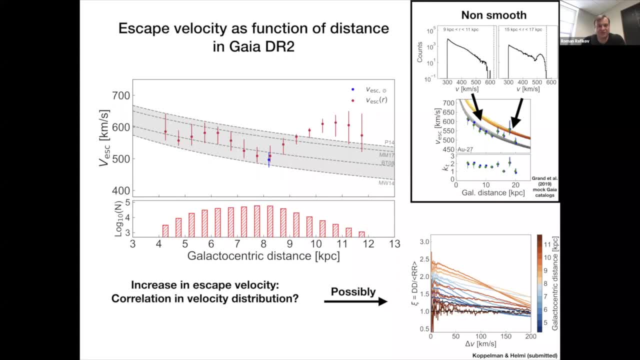 this concept of escape velocity assumes that everything is, you know, spherical, is symmetric. I mean, could this be explained by some dramatic non-spherical symmetry in a galaxy? I mean, maybe you're looking in certain regions of the galaxy, and so on and so forth. 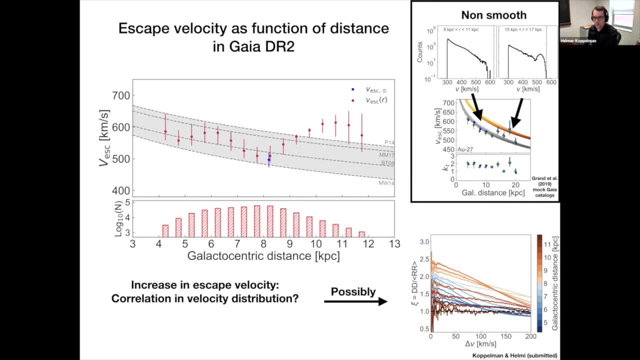 Which part is assuming the spherical symmetry that you mean? Well, I mean, it's just the whole thing. So you know, the actual escape velocity can really increase with distance, unless you do something very radical, So- Right? no, that's not-. 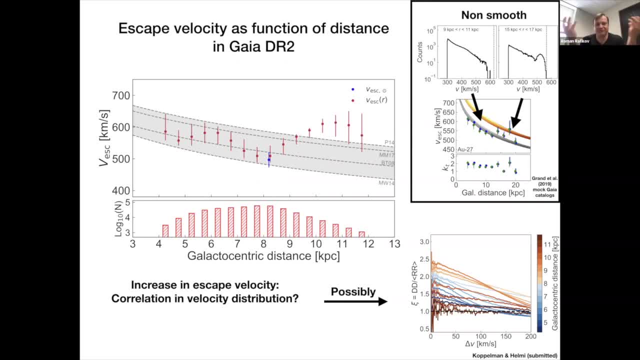 No, no, no, that's what I mean, Like something radical. Imagine that you have two black holes, like orbiting around each other. then, obviously, close to the black holes, the escape velocity is extremely high. but in the center and far away, you know it's much lower. 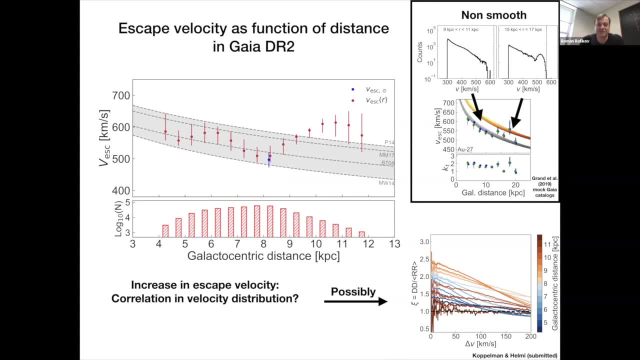 So you could play some sort of crazy games with this Right, definitely. So I don't think there's quite a physical explanation that the escape velocity can increase, except for some very exotic phenomena, And so I think the easiest explanation is just that the velocity distribution 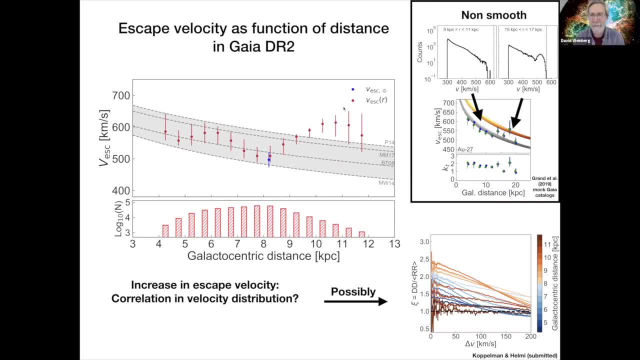 has a different shape in this region. here I'm mindful of the fact that Helmer's still on number one of the four things he was hoping to cover. so No, no, this is two. A little further, All right, okay. 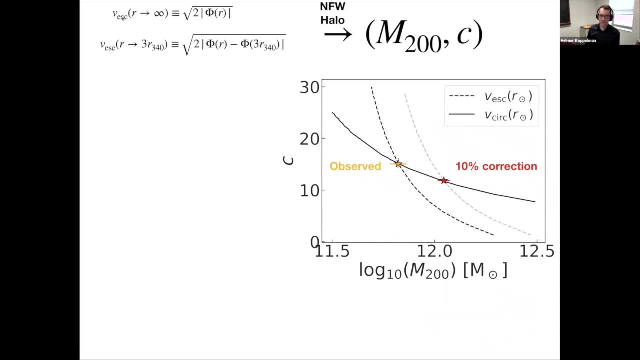 So anyway. so, as I was saying before, if you measure the escape velocity this is kind of a direct determination of the potential of the Milky Way. So we turned our observation of the escape velocity at the position of the Sun of 500 kilometers per second. 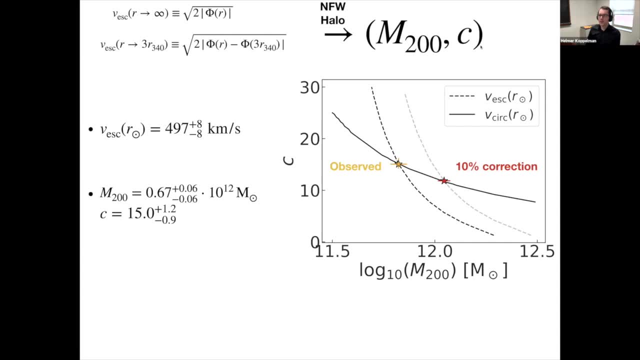 into a determination of the mass of the halo of the Milky Way. So what we did is we took just some assumptions on a baryonic component of the Milky Way and then we varied the mass and concentration parameter of the Nfw halo and so the the combination of the mass and concentration parameter that we find. 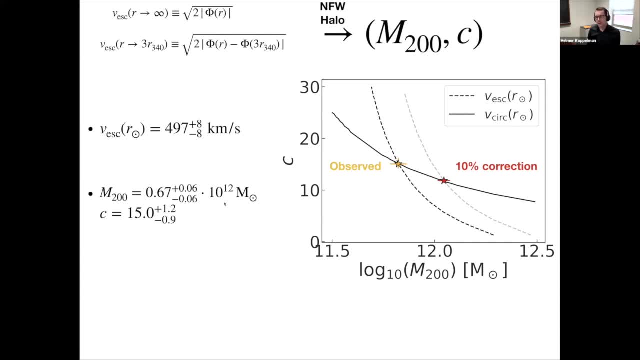 are the ones here which are a little, a little bit too low and too concentrated compared to values in the literature. but this is likely just because the determination of escape velocity is just, is likely biased low by this 10 percent, just because of the communication of the velocity. 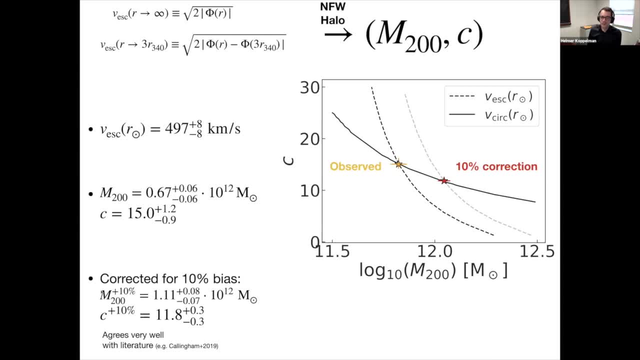 distribution. so if you correct for this 10 percent then the mass estimate does coincide very well with with expectations from the literature. but there is an issue that this 10 percent is just based on these simulations and we don't have a guarantee that actually the Milky Way should be corrected for the same. 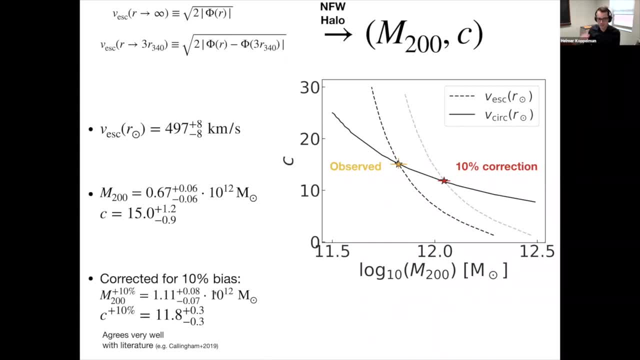 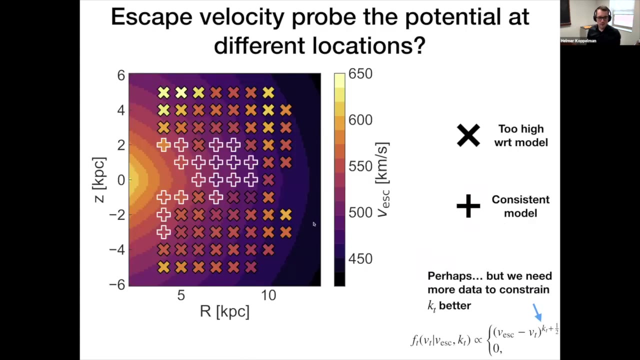 factor. so this is kind of, you know, very hand-wavingly, but we do think that the escape velocity that we determine is consistent, you know, with the, the mass estimates of the Milky Way from other results. I'll just skip over this slide and go to the next, next section where I'm going to talk about. I'm 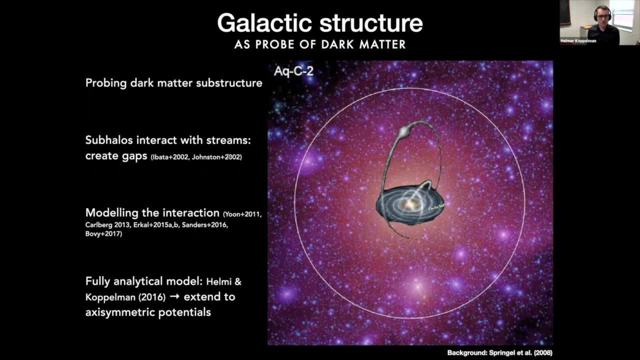 going to completely move away from data analysis and just go talk about a model, a fully analytical model, to describe the interaction of dark matter, subhalos and cold stellar streams. so, as I was saying in the first part of my talk, you know we don't have a good handle of the 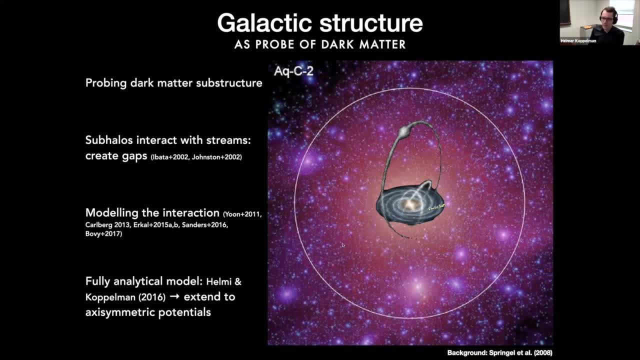 level of the Milky Way. so I'm going to go to the next section and go to the next section. so, as I was saying in the first part of my talk, you know we don't have a good handle of the level of small scale substructure in the halo of the Milky Way. 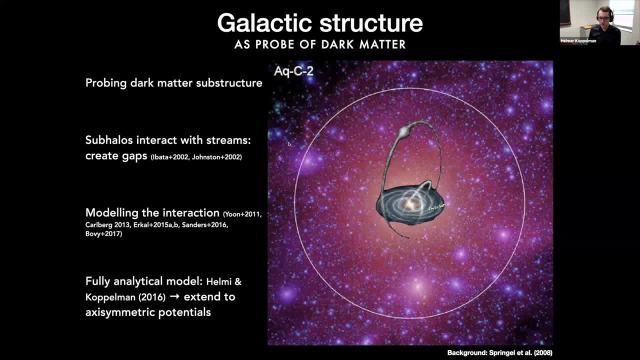 there are lots of expectations from simulations that are these dark matter subhalos, and a way to to put up the population of dark matter subhalos is to look at interactions with stellar streams. so the way this works is that if a subhalo crosses the stream, it will perturb the stream and it will create a gap in the stream. 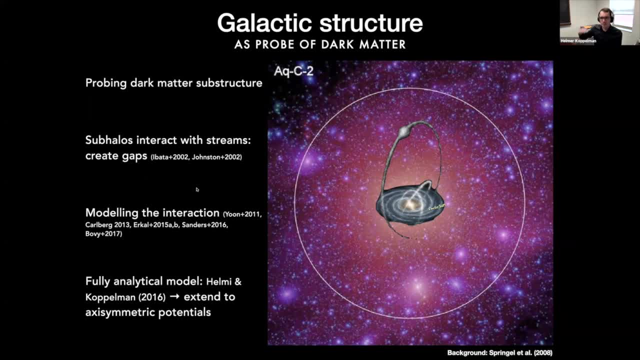 and so the hope is that, from modeling this interaction and from observing a lot of of streams, a lot of gaps and streams, is that we, from the observations, we can determine, uh, what kind of dark matter subhalo created the gap. there's a side note here is that we don't have a lot of observations of streams. 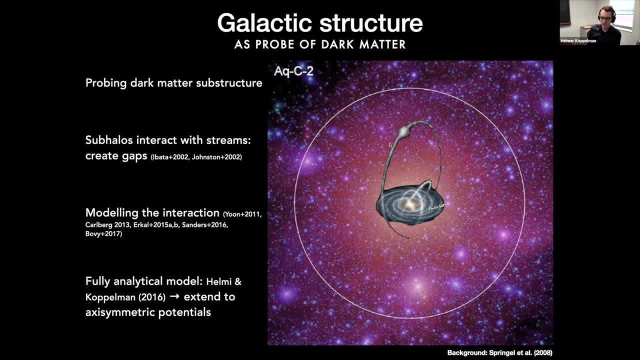 let alone observations of gaps and streams. I think there the current record is two. but so you know, even before we have these observations- we do have- we do need a, a model to to explain the interaction, And so in 2016, we worked on a model to describe fully analytically. 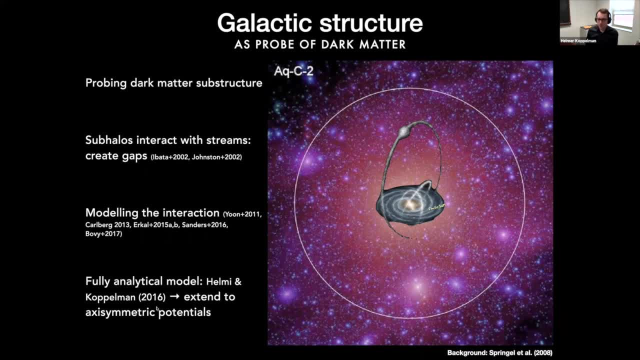 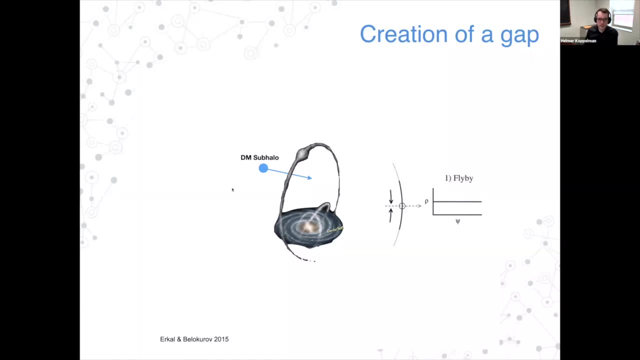 the interaction between a subhalo and a stream. This model only works for spherical Milky Way models, and so my job was to extend this to also exosymmetric Milky Way potentials And just to visualize the interaction. so if a subhalo causes a stream, it'll locally. 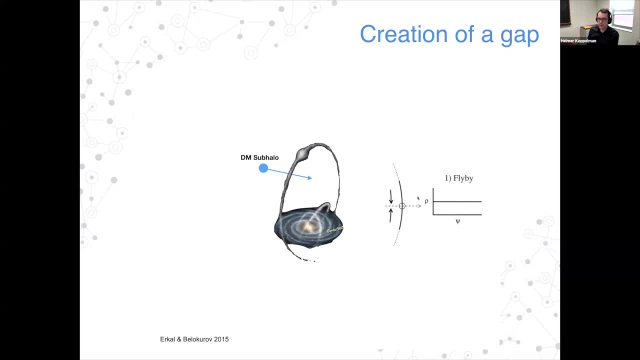 pull the stars in the stream towards the point of crossing For a very small amount of time. this creates a compression in the stream, so not a gap with the compression, But the long-term behavior is that it creates a gap. so the stars are kind of moving away from the point of where the dark. 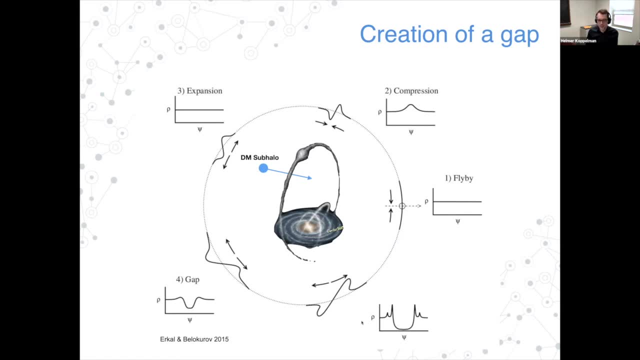 matter subhalo across the stream And there are two stages. so one is a shallow gap where there's just an underdensity and the late time evolution is just. the gap is completely devoid of stars. so you get two disconnected components of the stream. 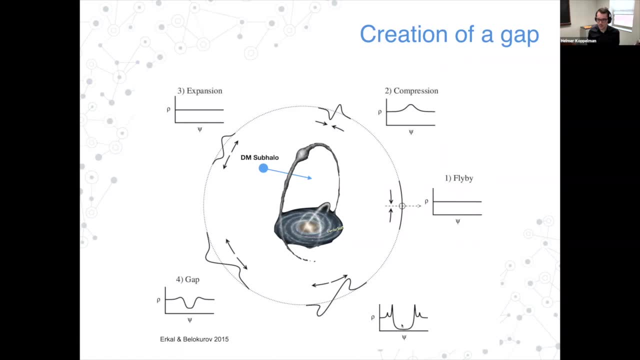 which used to be connected. so the gap truly is a gap, And so the aim of the method that we developed is, if there is an observation of the size of the gap, then to determine what kind of dark matter subhalo created this gap. Can we still determine the mass of this dark matter subhalo and the scale? 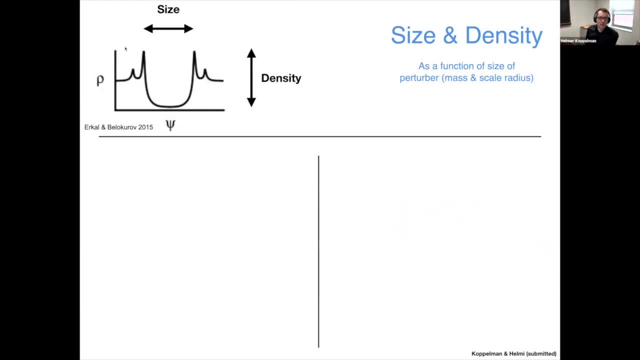 radius, And so the way that the method works is that we model the gap by two observables. One is the physical size, so it's the separation between the two edges of the gap, and the other one is the density, the central density of the stars at the center of the gap. 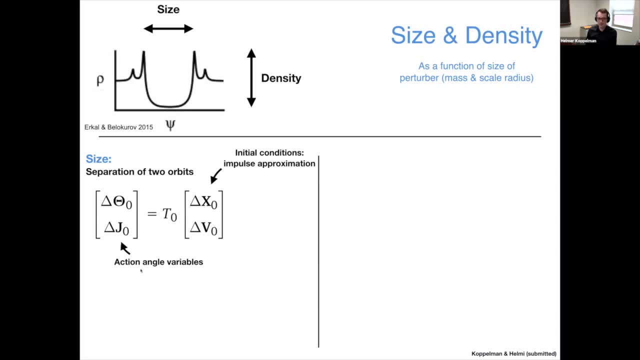 And so the way that we model this is by actually modeling this using action angle variables and by modeling things and action angle variables. um, you have to have a, or you impose strong limitations on the kind of milkway models that you can use, because for most, for the most realistic milkway models, you 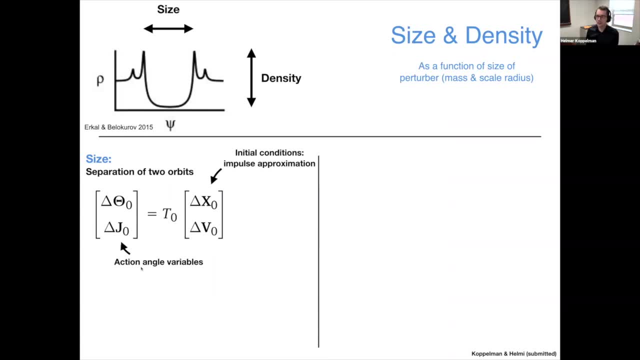 can't calculate action angle variables analytically and only numerically, and so by doing this fully analytically, we do constrict or limit our ourselves to models that are not fully unrealistic but may might not be the most realistic. so the way that the the method works is: we take the 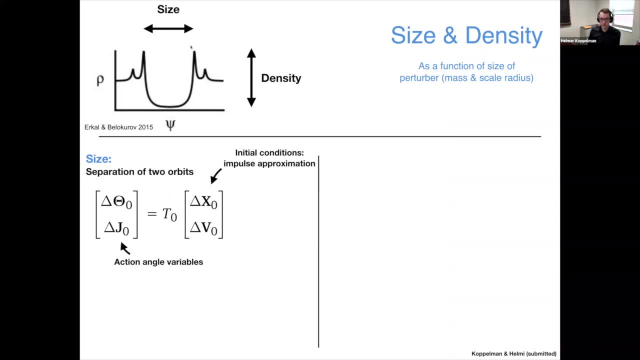 we model the size of the gap as the separation of just two orbits, one on each side of the gap. and so we take the separation vector, we transformed it with a matrix multiplication in to action angle variables, which then, subsequently, the benefit of using action angle variables would be the time evolution of systems is very simple. 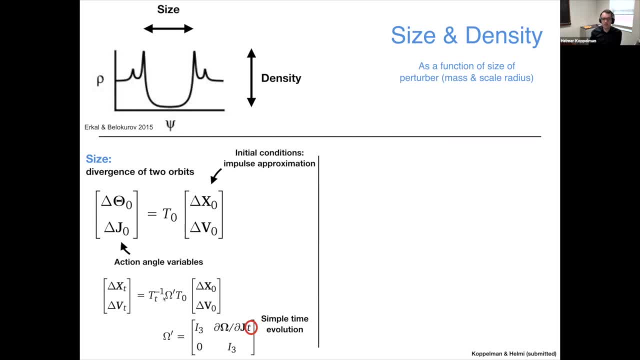 in this coordinate system so we can use a set of matrix multiplications to predict what the separation of the two edges of the gap will be as a function of time. so this is what we're after: to predict, you know, how the gap will grow as a function of time. 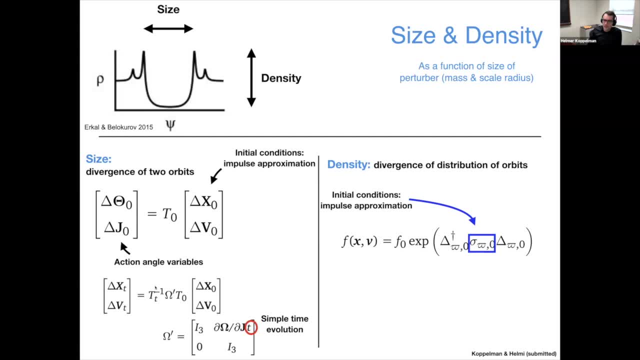 and so we're using the, the exact same framework, so the exact same matrix multiplications, to also describe the. what happens to the density of the gap? density is not modeled as two orbits, but just as a distribution of orbits at the center of the gap. initially we assume it's a gaussian distribution. 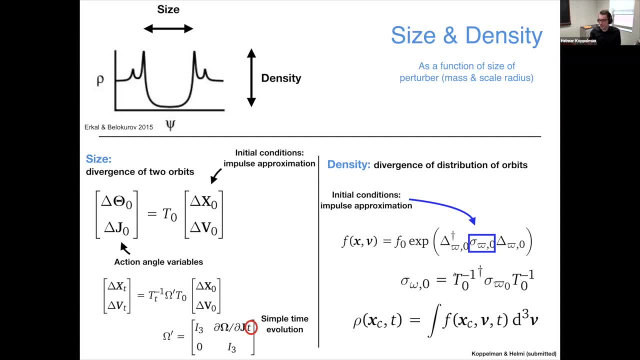 using the same matrix multiplications. we then evolve this gaussian forward in time and then, at any given time that you know where you want to evaluate the properties of the gap, you can marginalize the velocities or a gaussian over the velocities to obtain the physical density at the center of the gap. 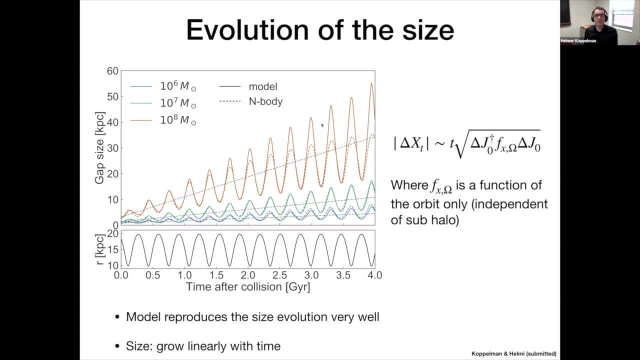 so that's, that's the technical part of the method, and so now i'm just comparing the predictions for the evolution of the, the gap as a function of time, compared to m body experiments. so what we're looking at is three different measurements of the evolution of the size of a gap in a stream for three different 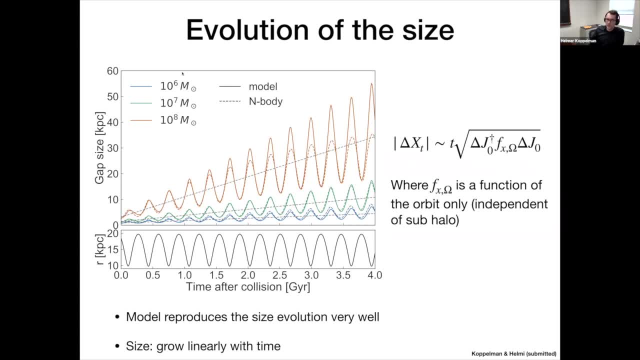 experiments where the stream is interacting with three different subhalos with varying mass. so, as you, as you would expect, the, the most massive sub halo, creates the largest gap, which is just a very intuitive um result. and so you see, the, the, the model uh, agrees very well with the end body, except for for very large gap sizes. but this is just a. 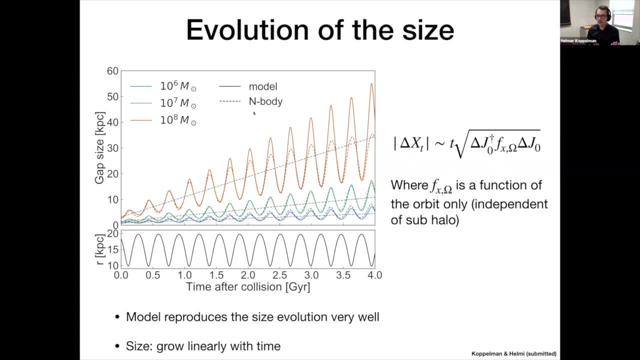 restriction from the the body experiment, the way that we measure the gap size. this is not actually. it doesn't reflect, uh, an issue in the model. it just reflects an issue in measuring the size of the gap in the m body. so, just overall, the agreement with the m body and the model is really accurate and so we can use now the analytical framework. 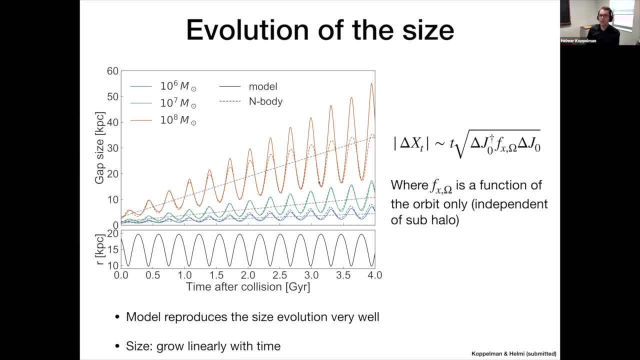 to calculate what is the average time evolution of the gap, and so the average time evolution is linear, and the the reason that you see these non-linear wiggles is just the kind of the orbital motion of the gap as it moves between paracenter and upper center. 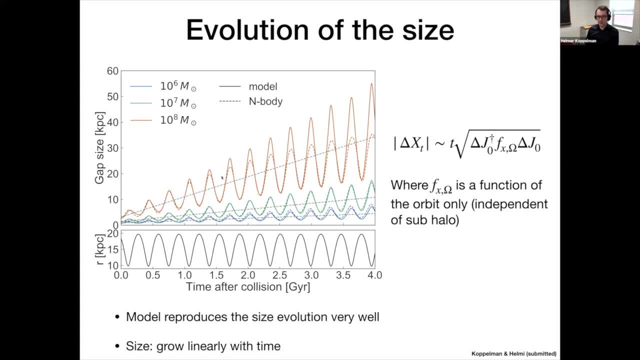 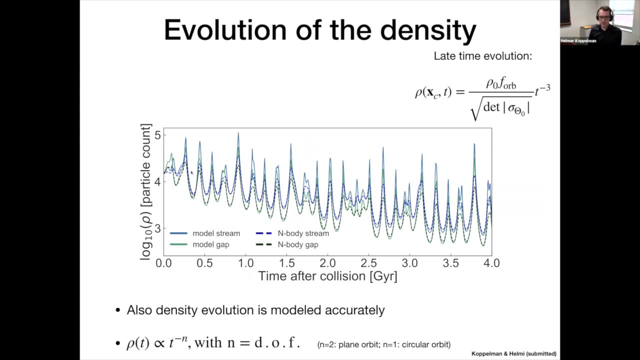 and so if you smooth these uh wiggles and take just the average time evolution, then this is linear in time. so this is the prediction of the analytical framework and so, similarly, the, the densities of the, the density, central density of the gap is reproduced accurately by the model. 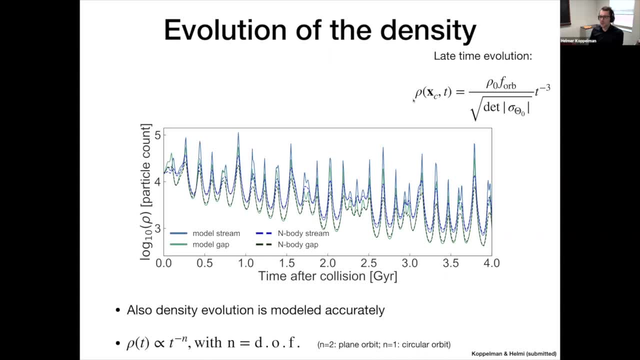 compared to m body experiments, and so the prediction is that the density of the, the gap, decays. this is a function of time to the power of three. actually, this power here, this three, depends on the degrees of freedom in the orbit. so for a circular orbit, the density drops less quickly than for a non-circular orbit. 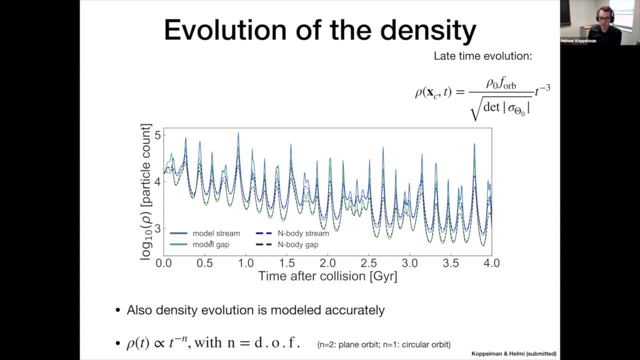 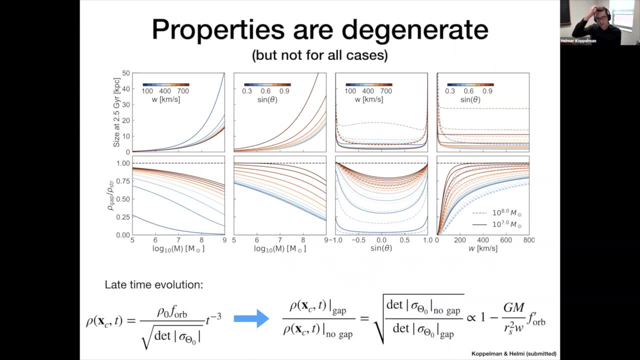 well, just to show that the, the, the model, predicts to high accuracy what happens to the, the gap, as it evolves in time. and so now the you know, ultimately, the goal is to be able to infer the mass of the sub halo by observing, for example, the size of the gap. 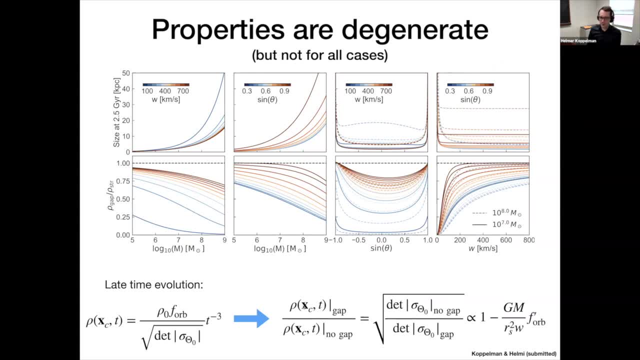 and the density of the gap. and i'm showing here the density contrast, which is just the the ratio of the density of the gap relative to the ratio to the density it would have had if there were no sub halo impacting it. and that's just because, if you take the ratio, the time dependence drops out. 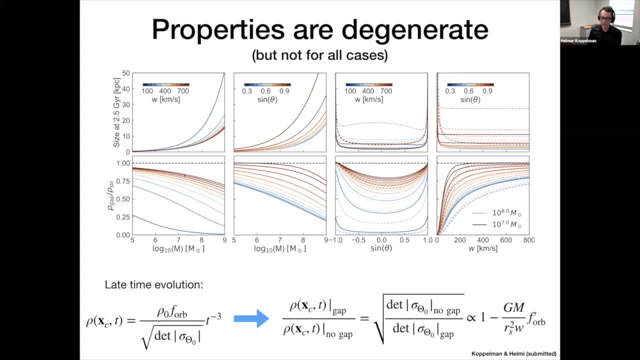 well, just for understanding the panel here, this is just showing the density, and so the three, uh, the four columns show the, the dependence on the mass, the impact angle. so which is the angle at which the sub halo impacts the stream and the relative velocity at which the sub halo impacts the stream. 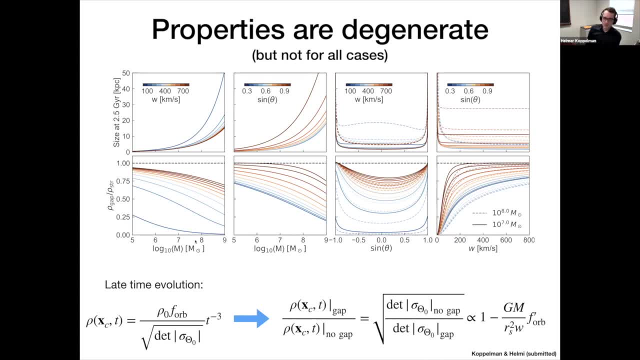 and so what you see is, if you just focus on the left column, is intuitively: the more massive the sub halo is, the larger the gap in physical size, but also the steeper the gap is in density, so the more affected the stream is is, however, some small or not a small, but the major issue is that the 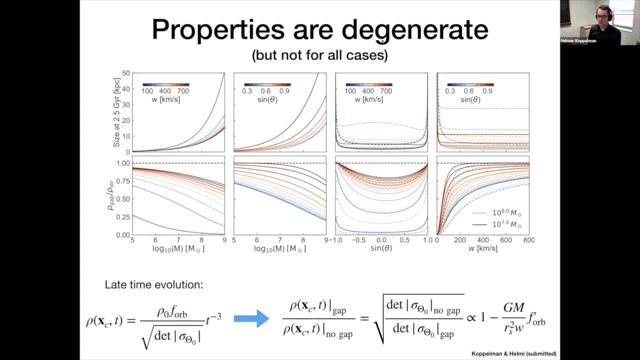 impact parameters. so the mass impact angle and relative velocity are degenerate, but they're only so. the from the literature, the expectation was that the degeneracy is pretty high. we actually saw. our model shows that the degeneracy, the sort of degeneracy, and the 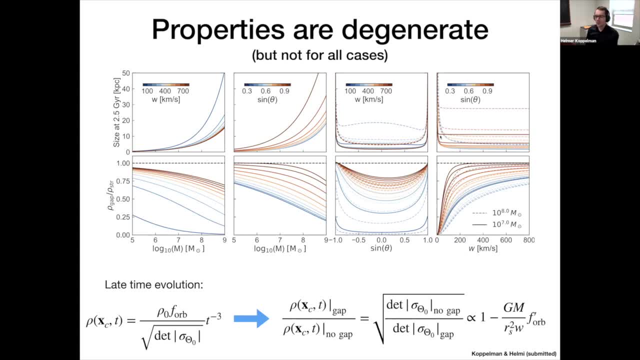 mass impact angle. relative velocity is only the case for very extreme impacts. so only where the uh, the global, the linear demonstration is, the impact angle is head-on. so when the stream and the sub-halo move head-on or tail-on, or for really low relative velocities, 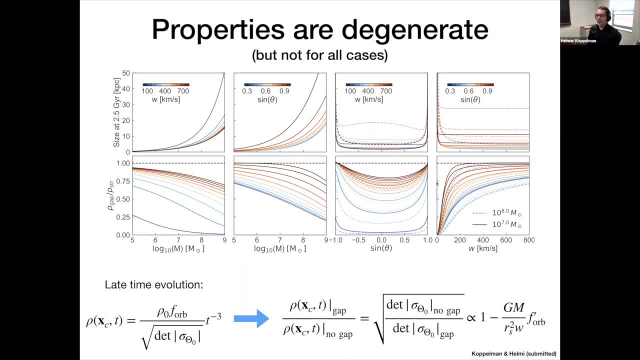 it's actually from our model. we showed that you know if you assume any most likely impact angle, which is most likely zero, and most likely relative velocity, which is 200 or higher. Under these assumptions, the parameter is actually not degenerate, and so you can from observing the gap, you can infer the mass of the subhalo that created this, which is a very positive note for when we do have observations of gaps and streams. 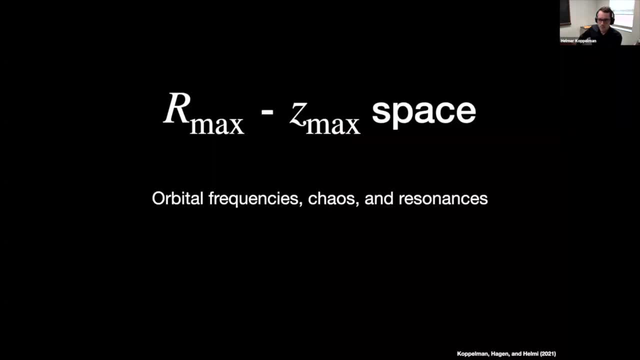 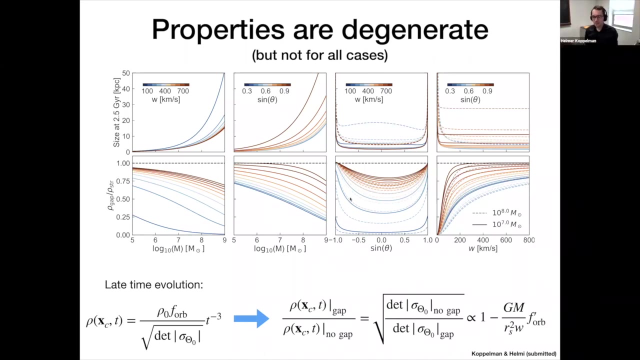 Right, I don't know if there are any questions. I'll move on to the next section. Is there a degeneracy between perturber mass and time? Yes, so here we do assume that we have complete knowledge of the time when the impact happened. 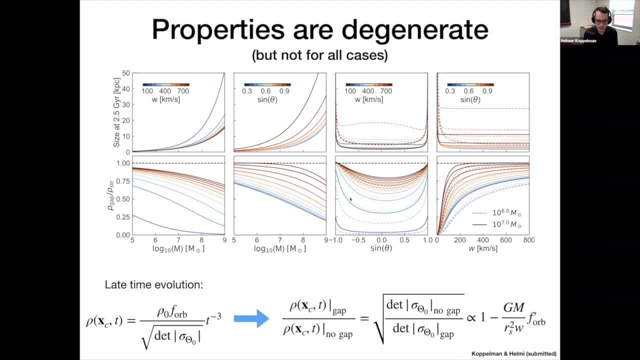 This is not fair. so we do assume that this is something that you can infer from the observations. So there are a couple of ways to do this. But yes, so for this particular assessment, we do assume that we know when the subhalo impacted the stream. 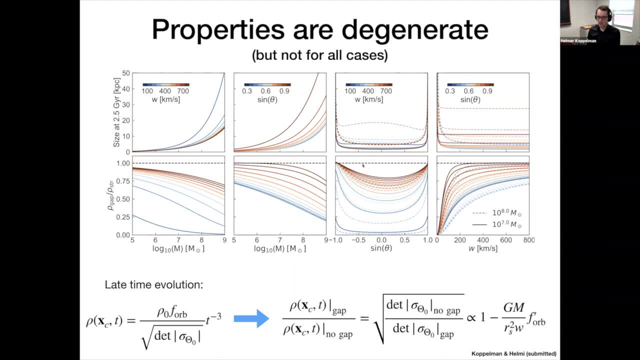 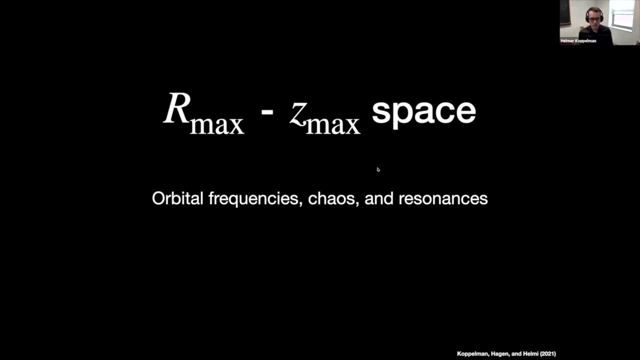 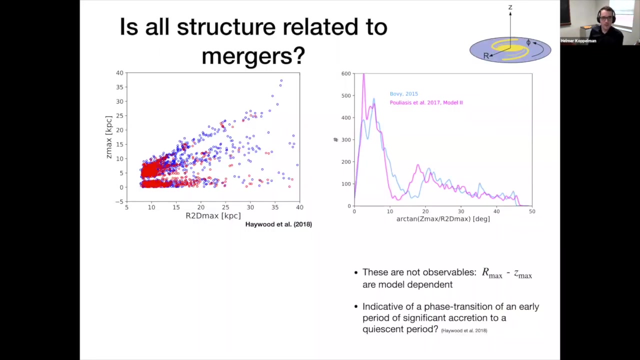 Right, And so in the last bit of today I want to talk about structures in a very particular dynamical space of rmax and zmax, which I'll show in the next slide, what this means and their relation to orbital frequencies. And so the particular structure in the halo that I'm talking about is 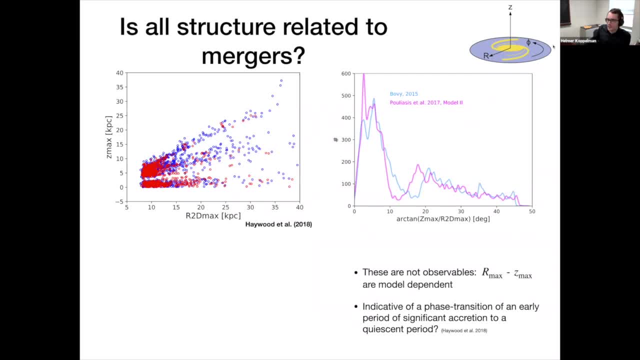 So zmax and rmax is just simply: if you take a halo star, integrate the orbit of the halo star forward in time for a long time and you just identify the maximum z value and the maximum r value of the star and then you plot this in a diagram. 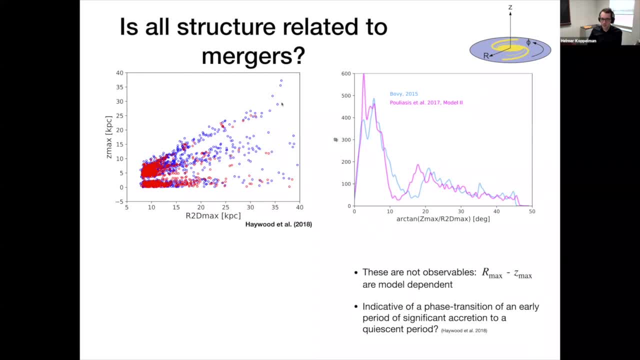 And so what you see is that in this diagram, the distribution of halo stars is not uniform, but the stars tend to be populated along these lines And there tend to be this very strong, These very strong regions where you know there's these empty regions where there are no halo stars. 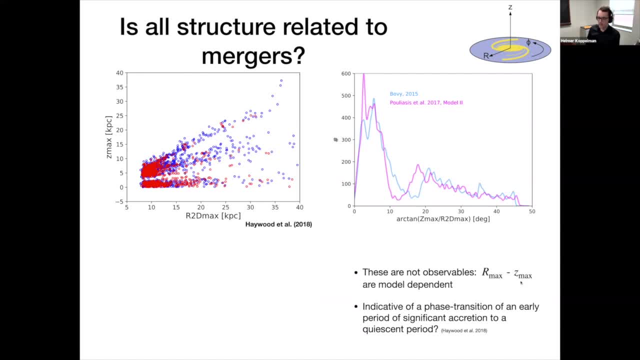 And so there's a major side note here- is that these rmax and zmax values are absolutely not observables. These are very strongly model dependent And so actually so. the diagram here was created by these authors, and they analyzed the model dependence by showing, for different models, what happens to these features in this space. 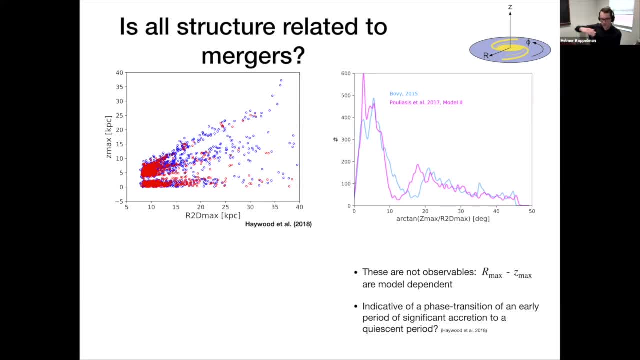 They showed that the features do change in location, So this large gap might move upward or downward, But on average, in general the features are there for the models that they they compare to, And so it's very amenable or very attractive to then draw lines in this diagram, select stars and start to study them and think that you know it's very. 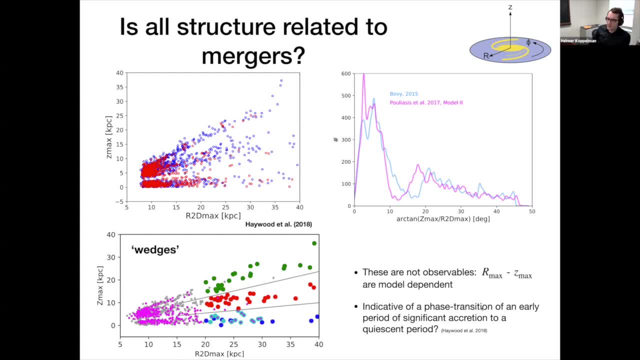 attractive to say that these structures are created by some kind of phase transition And the merger history of the Milky Way, So that these each independently correspond to mergers with dwarf galaxies in the Milky Way. And so we got interested in these structures. We try to understand what is creating these kind of, you know, non-uniform structures in this space. 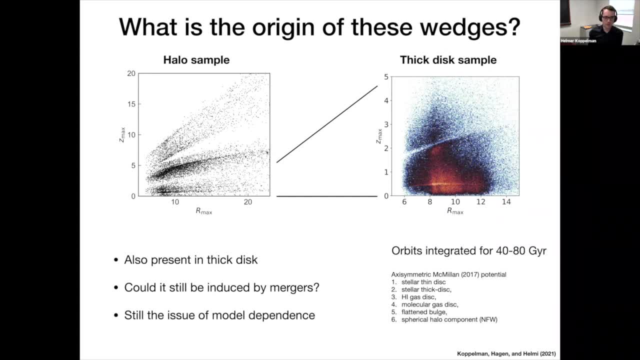 So we did the exact same test or exercise: to take a halo sample, calculate orbits, identify the maximum z-valves, maximum Z value and R value and plot the distribution in this diagram. And so you see the same. so we use a different Milky Way model. 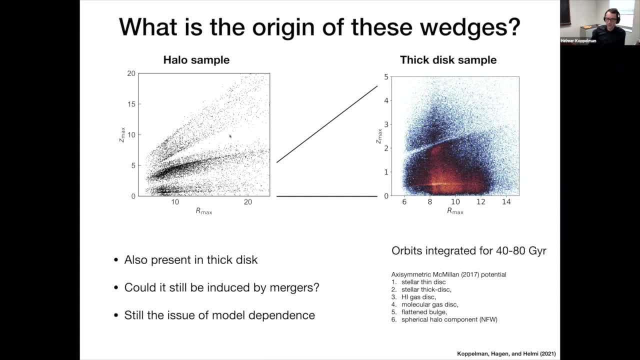 but you see the same global structure. It is sharp lines, empty regions and over dense regions. And this is the Gaia DR2 sample. Yes, And so one concern is that the similar structures features are apparent in the thick disk sample. 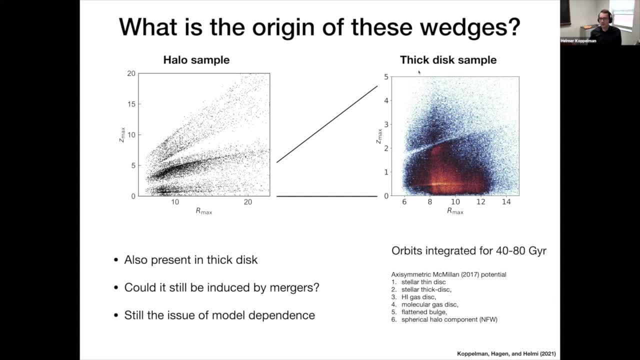 So it's not just something that's present in the halo sample, it's also present in disk stars. Naturally, disk stars don't have a very high maximum Z value, so that's why it's zoomed in, But already this shows that it's unlikely. 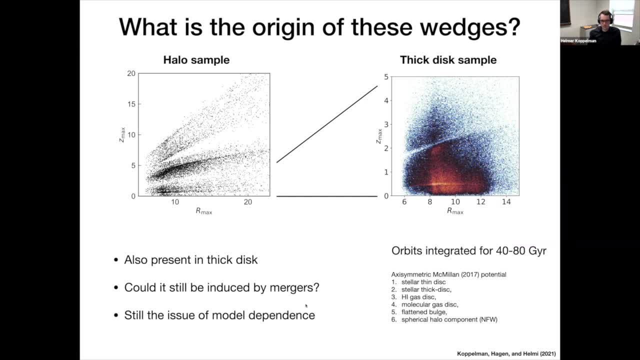 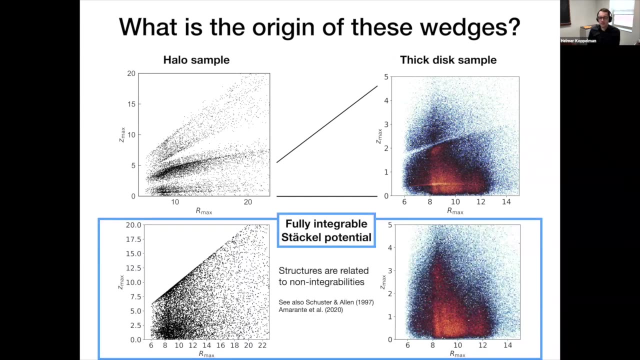 that these structures are related to individual mergers, But there might be still a hope that they're induced by mergers. There's some kind of effect of dwarf galaxies interacting with the population of halo stars. The most compelling evidence I can show you that this is not the case is by taking a 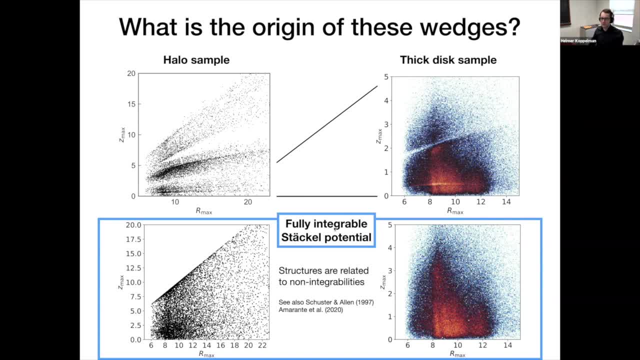 doing the same exercise, but now for a Milky Way model that's fully integrable for a so-called stack of potential, And so what this means is that the orbits in this Milky Way model are all regular, So there's no chaos. All the orbits are periodic and well-behaved. 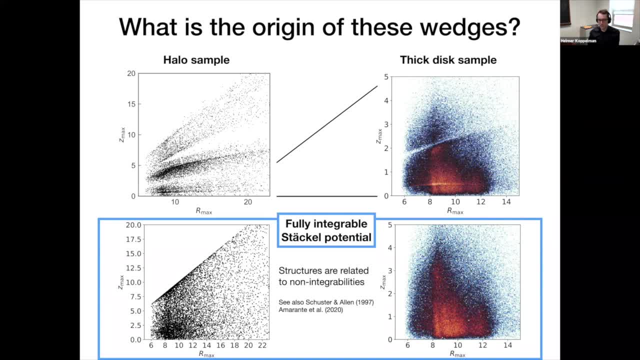 And so in this Milky Way model none of these features are present, So especially the panels on the right. they show that the overall distribution of Z max and R max is the same. except for that, these very strong empty regions and over-densities are just completely gone. 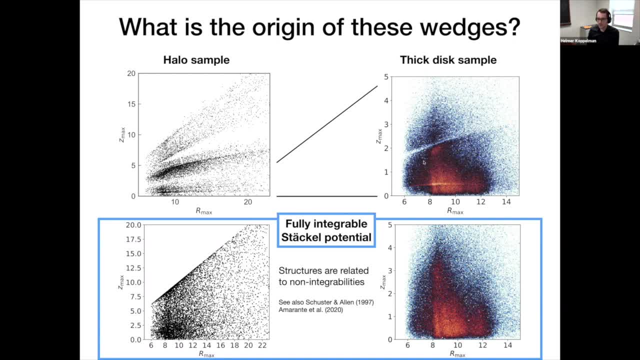 And so this means that these structures are purely artificial and induced by the Milky Way model that you assume. So they're due to non-integral abilities in the model of the Milky Way, And so, and just because of time, I think I'll just skip the next slides. 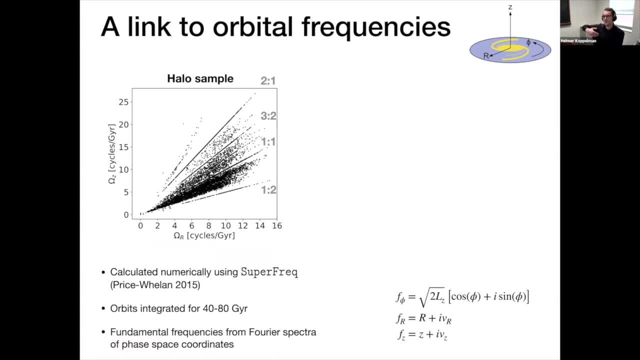 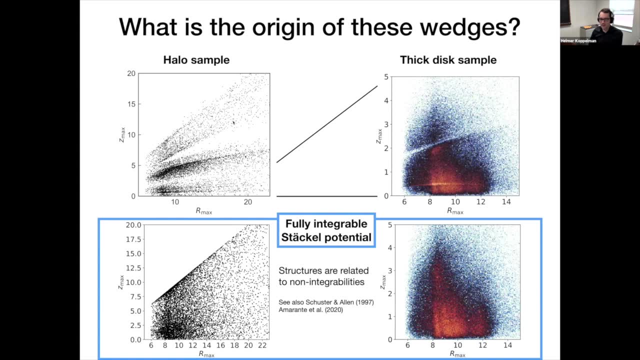 So we- the rest of the paper is just us- explaining and analyzing this further, showing that indeed these structures are caused by chaotic regions in the specific Milky Way model that's assumed here. So these are completely artificial and not related to merger history at all. 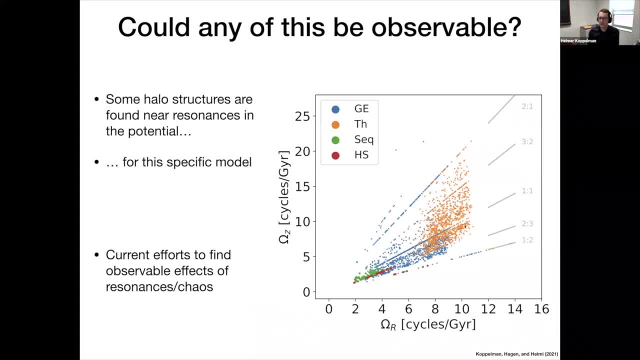 And so the interesting question is: because these structures are artificial and induced by the assumptions that you make on the model for the Milky Way, is there a way to turn around this argument? Can you find observable features in the halo of the Milky Way that are indicative of chaotic regions in the Milky Way? 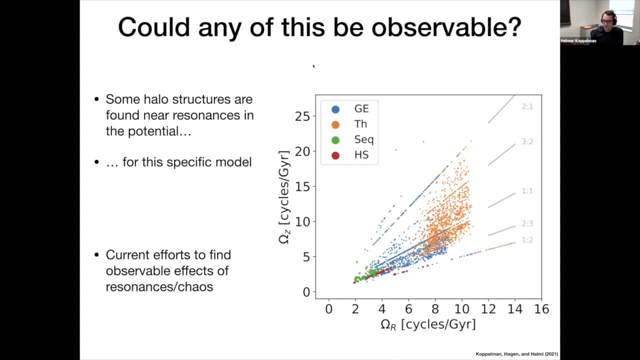 And can we maybe use this to constrain the potential of the Milky Way? And so these are questions that are currently on my mind, which I'm not too optimistic about, but this is kind of the direction in which I am moving, And I think also a couple of other people are moving. 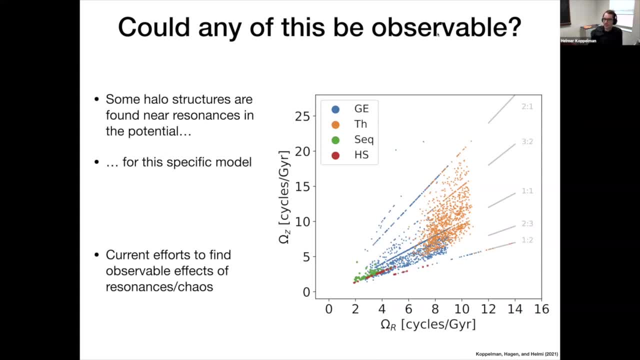 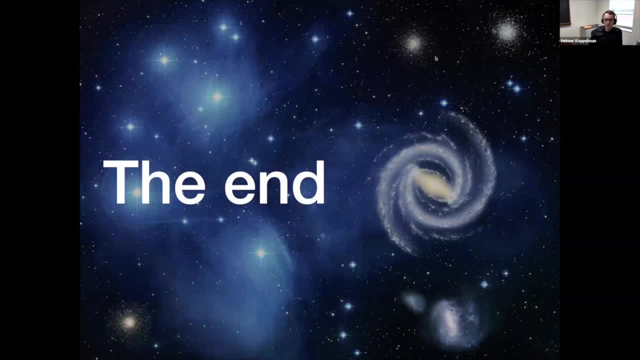 and still look for these kinds of structures that are created by chaotic regions in the Milky Way, which is not one of the ongoing works in progress, And so that's it for today. Thanks for your attention, And let me know if you have any questions. 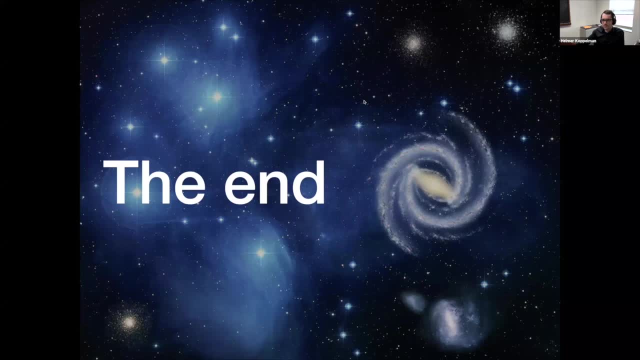 about the talk of today. Thank you, We can take a few more questions. To go back to the escape speed for a minute, if you divide up your sample by angular direction, can you check whether you're getting consistent values at different angles? 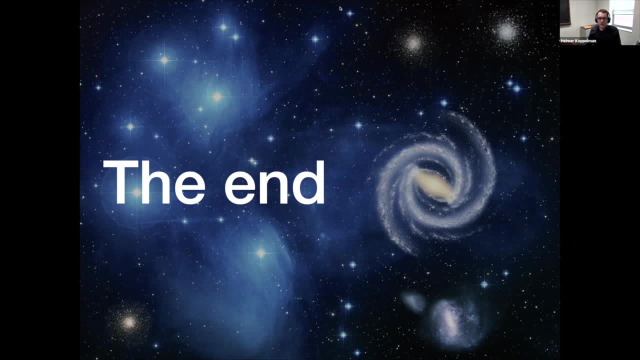 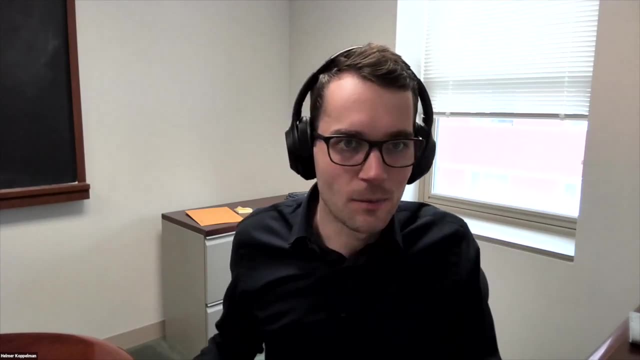 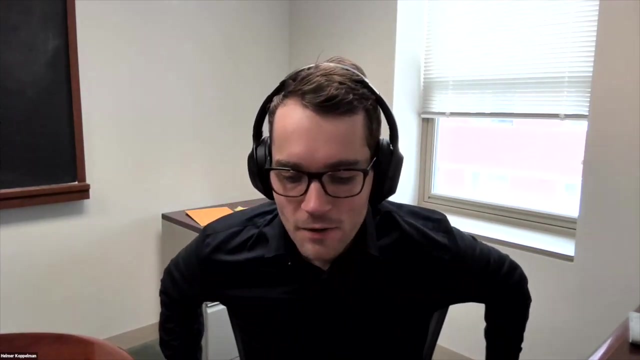 Yes, I did try this a little bit. I'm still looking at my screen our mi —, our Slides. Hi, there you are. So I did try this exercise, And so one of the issues is that, quite quickly already, you start to have a features resolution. 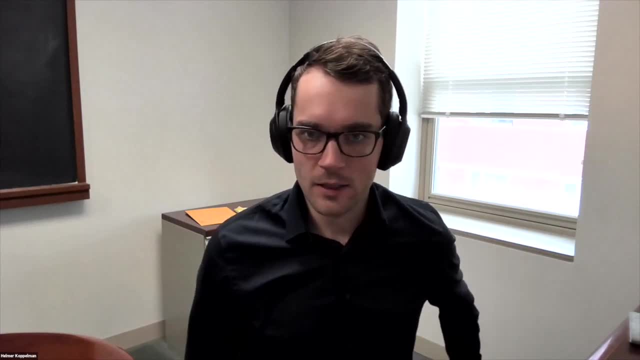 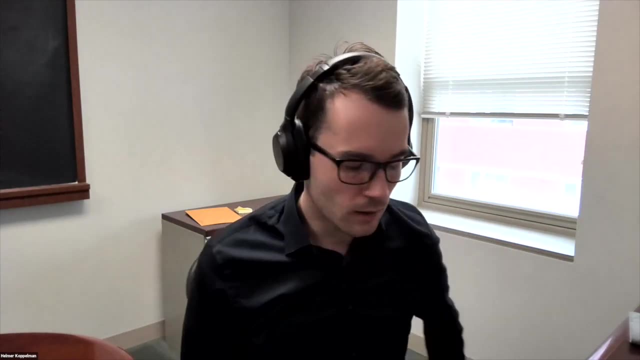 So it's a low number of stars to infer both k and the 4 côté simultaneously. So that's the issue that we have. All right, All right, Yeah, so, so many times. so, oh, is this spicy? at least we have with the sample of halo stars that we have. 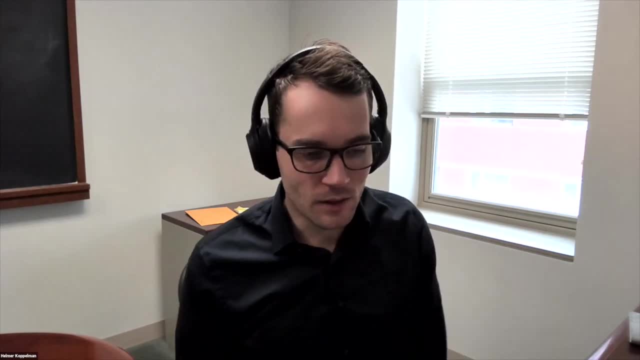 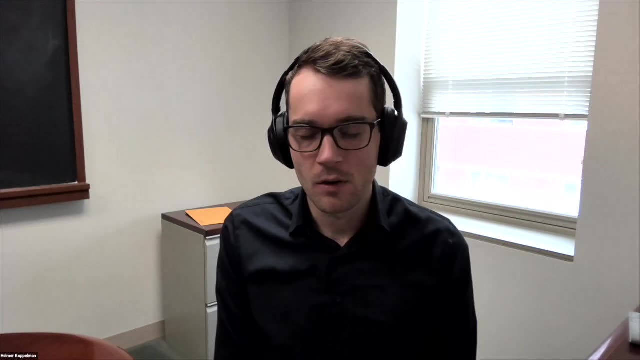 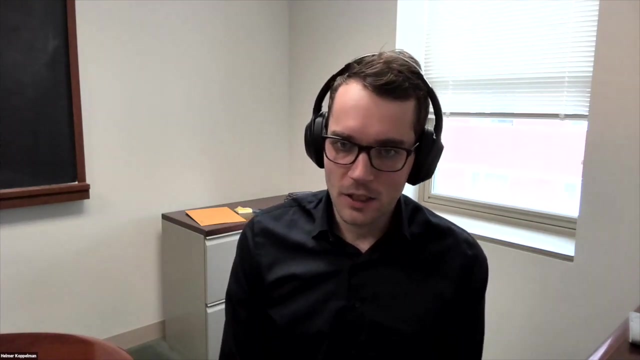 And so from the results it does look like there is not a strong angular dependence, and also not if you just take stars above and below the disc of the Milky Way, for example. the results are consistent, but the uncertainty, the error bars become significant. 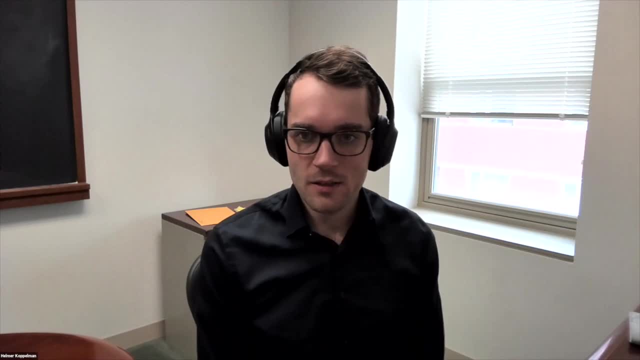 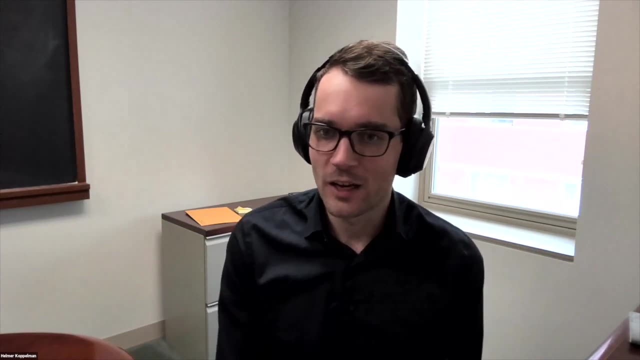 And so there is yeah, so it is difficult to do this exercise. Well, I do think that this is actually already possible with the latest, the most recent data from Gaia. It's just I haven't done this, I haven't redone this exercise as of yet. 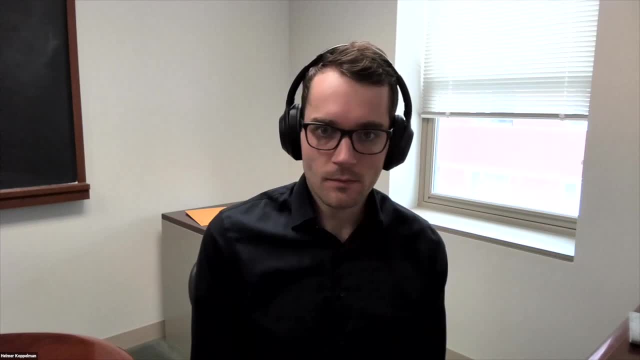 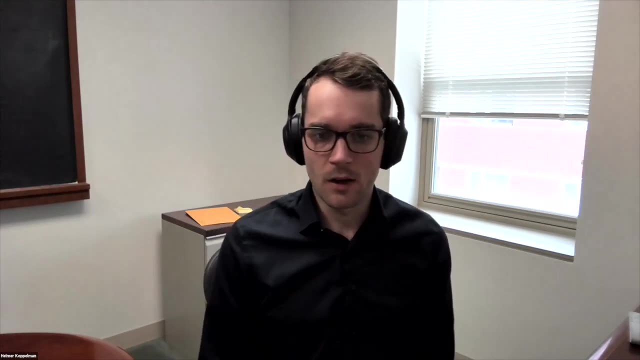 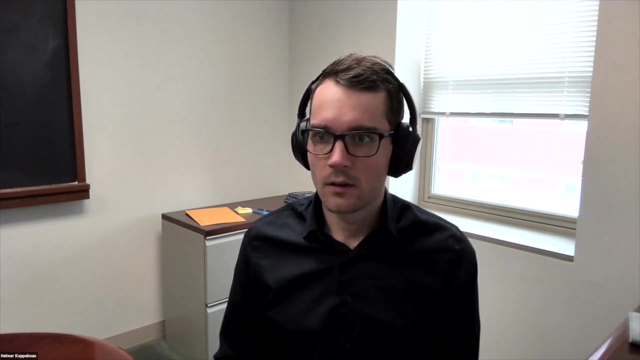 But I think currently it is possible to do this, which is, I think, actually quite interesting to do: to look at different locations in the Milky Way and to see if the escape velocity is different as a function of location. On the last part, I wanted to 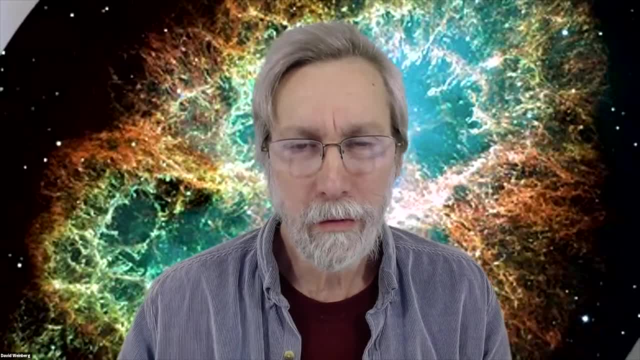 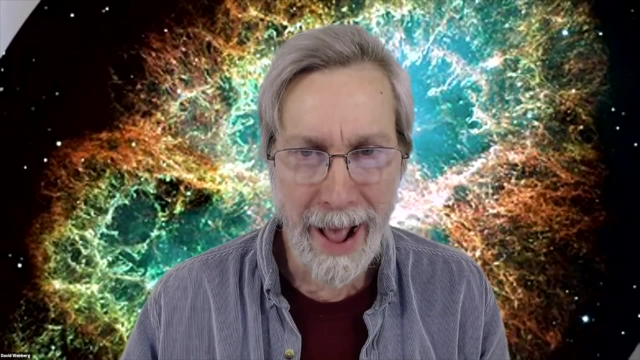 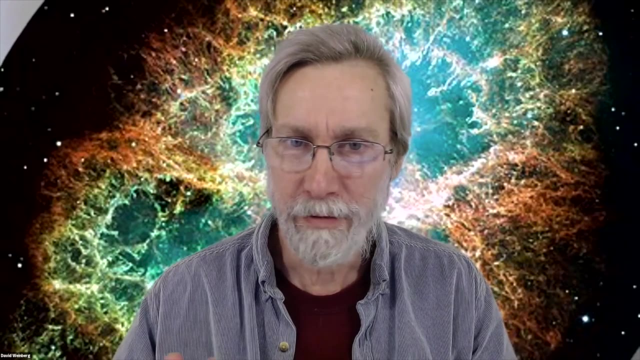 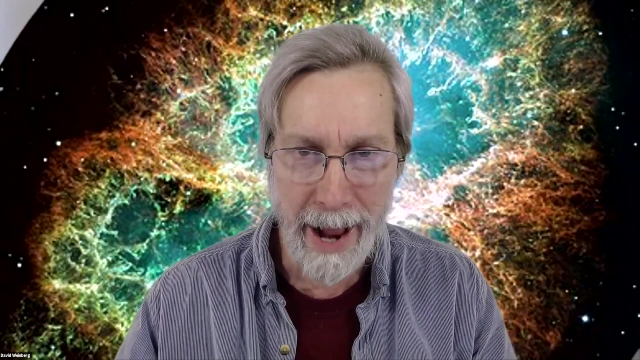 check. I was understanding the way when you how you're using the word artificial. So you mean that if you actually knew the R max and Z max of all these stars, then you wouldn't have this structure and the wedges are there because of the way R max and Z max? 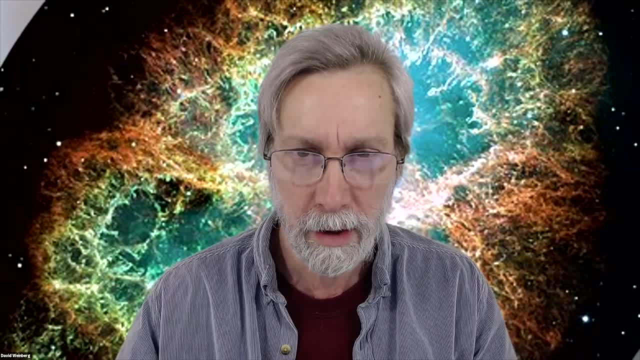 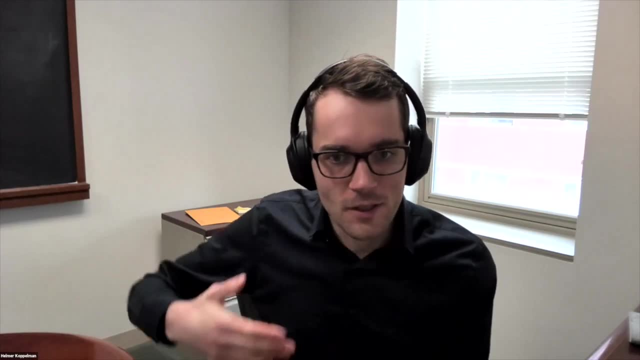 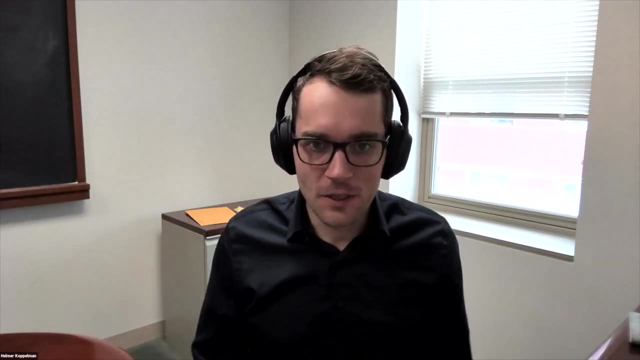 are being inferred from the observables of the stars. So what I mean specifically is that if you look at the, so what is observable is the distribution of positions and philosophies of the stars. Yeah, And so if you take just a random uniform distribution, 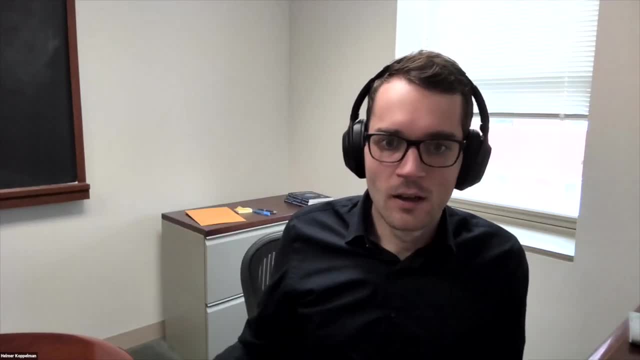 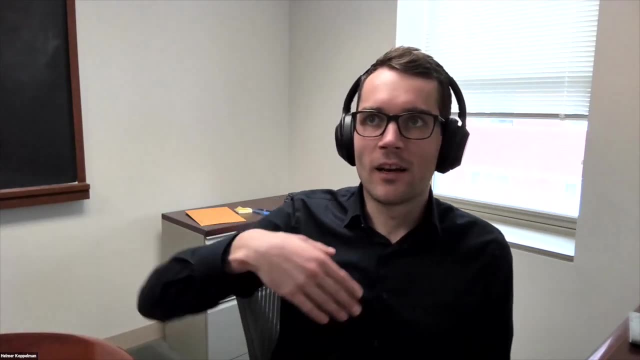 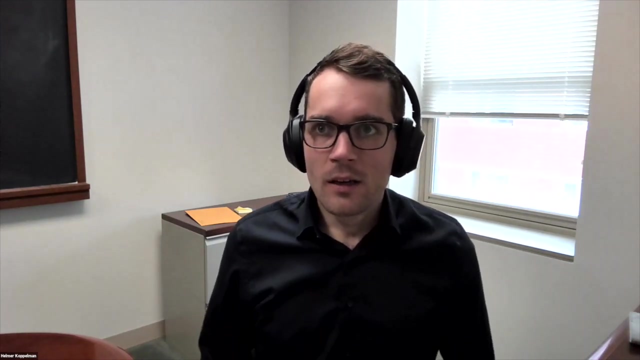 then you would get the same structures in space. So the structures are purely an artifact of the model and they don't tell us anything about the observed distribution of the halo stars, So they're not telling us anything. They don't tell us anything about the observed 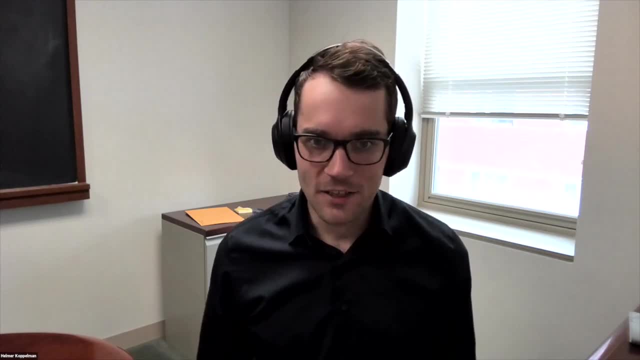 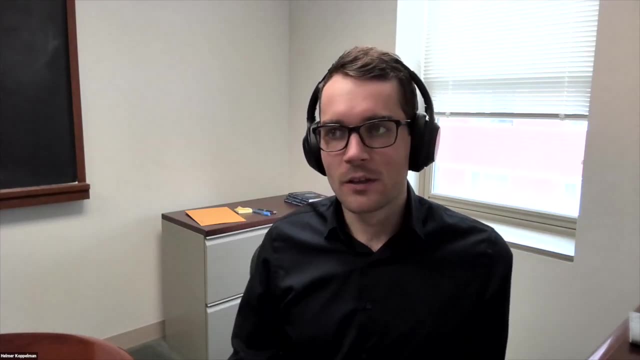 they don't constrain anything, any information on the potential of the Milky Way. They're just an effect of the assumptions of the model, So they don't. there's no in these structures and R max, Z max space. there's no additional information that we can use. 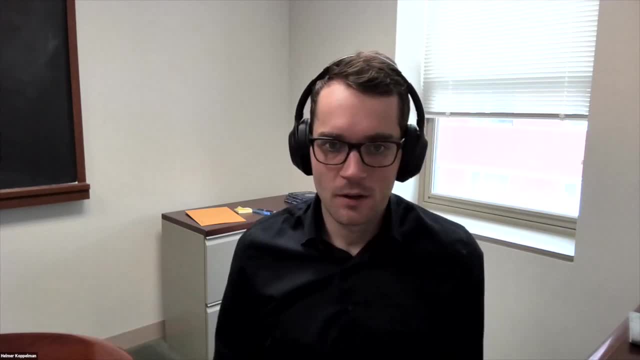 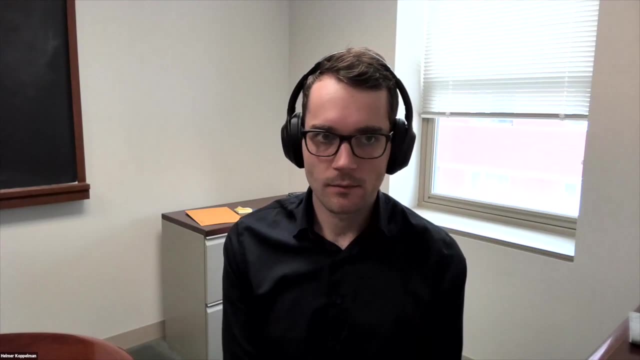 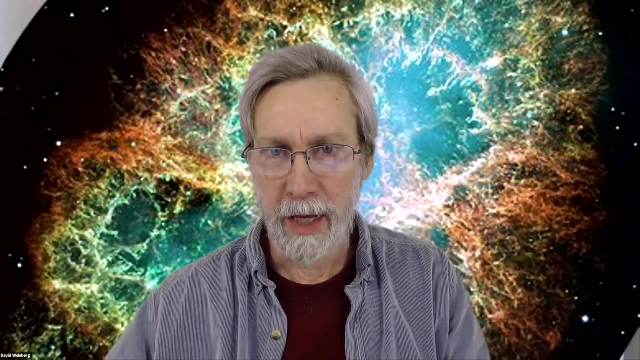 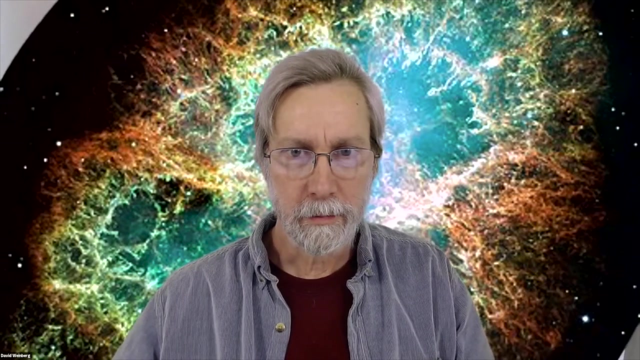 to constrain the mass of the Milky Way or its shape. That's what I'm trying to say. Okay, All right. well, if there are no further questions, thanks once again and encourage those of you who are interested to join us at three for follow up conversation. 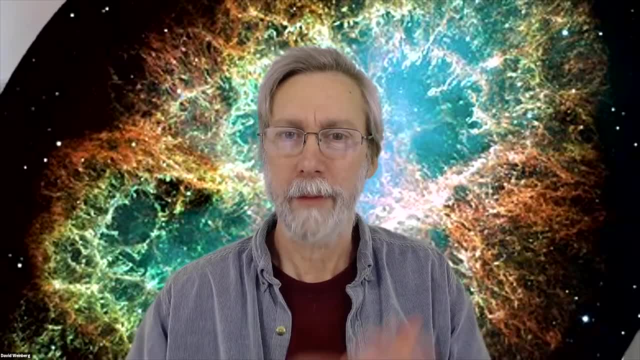 about this and maybe future projects. So great talk, Helma.